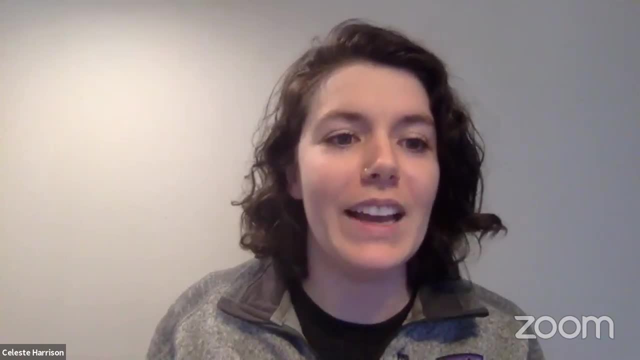 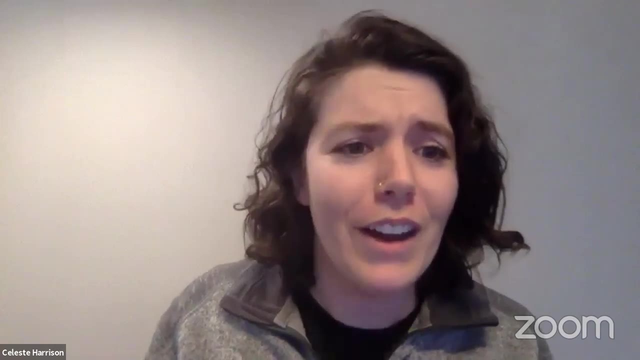 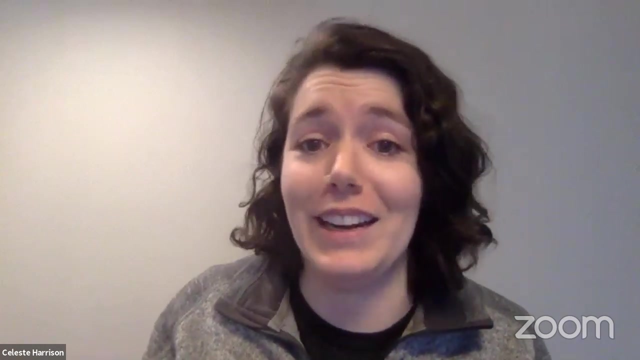 the District of Columbia, Florida, Georgia, Illinois, Indiana, Iowa, Kansas, Kentucky, Maine, Minnesota, Pennsylvania, Puerto Rico, South Carolina, Texas, Virginia, Washington and Wisconsin, plus also students in Canada, Peru, Pakistan and the United Kingdom. There are a few special groups. 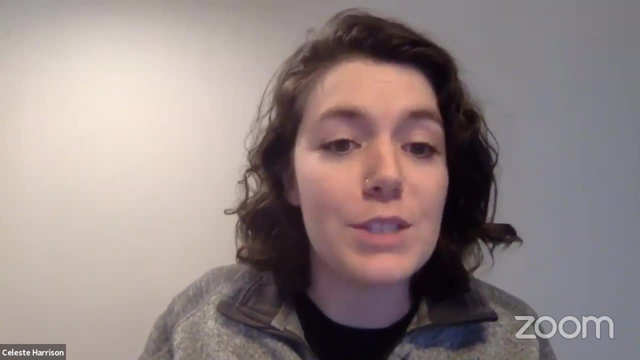 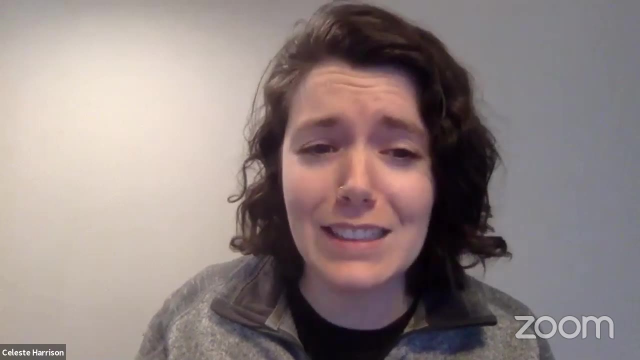 out there that need to get a shout out today. So I want to say hi to Ms Bergman and Ms Watkins, fourth graders, the elite SDGs. Ms Laura's class, surfskate science. Ms Branch's third grade. 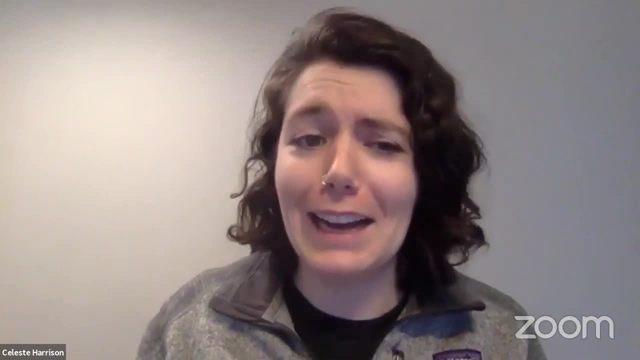 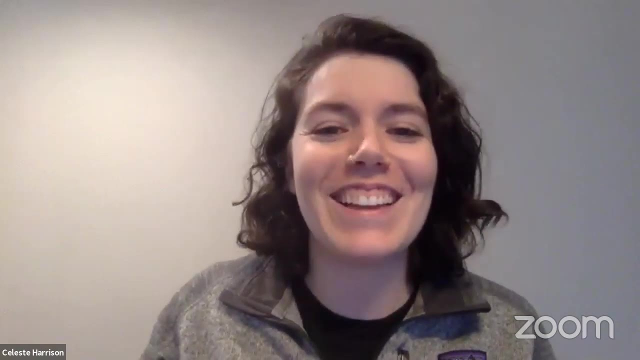 and the Burns- Phillips, Earl Gould, Green, Eisenhardt, Acosta and Meyer, as well as Sarah's family, Syrah, Keeley Brody and, of course, Grandma Marge. We're really glad to have you all watching today. 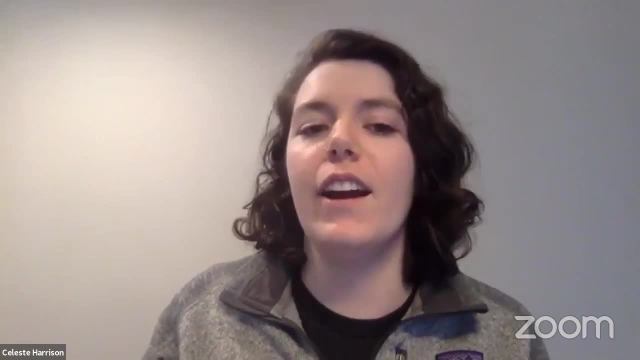 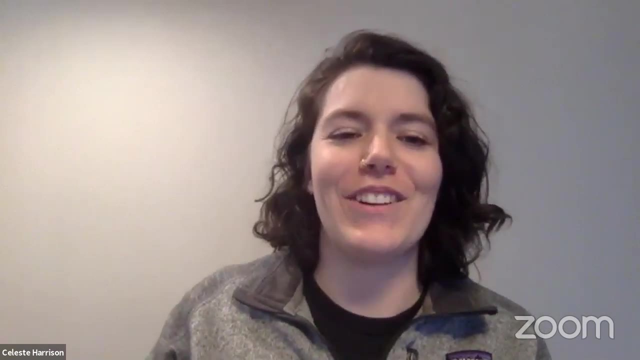 I know that I couldn't possibly have gotten everyone, so if you're out there and I missed you, go ahead and introduce yourself in the chat bar and we'll say hi. But that is plenty from me for now, so I think it's finally time to turn it over to Lauren for today's Explorer Classroom lesson. 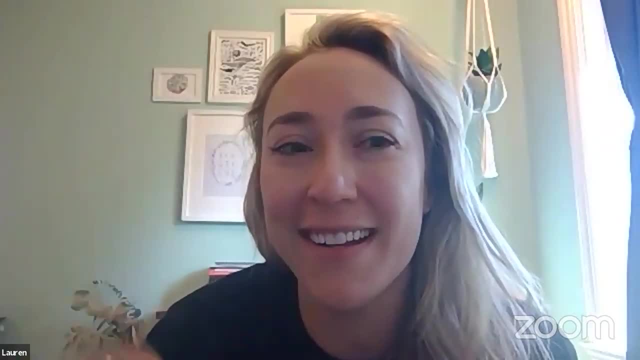 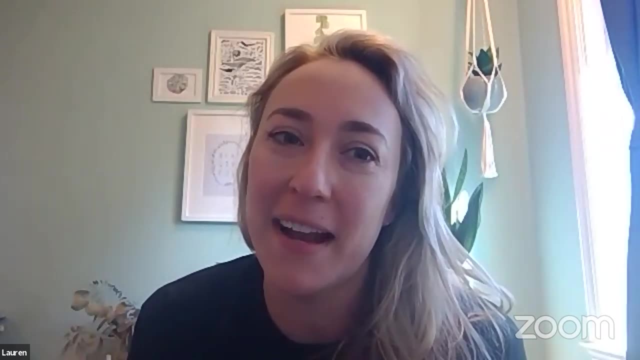 Awesome. Thank you so much, Celeste. Hi everyone, Thank you. Thank you for letting me come into your homes via your computer and give you a little lesson, tell you a little bit about the science that I do in my work with National Geographic. 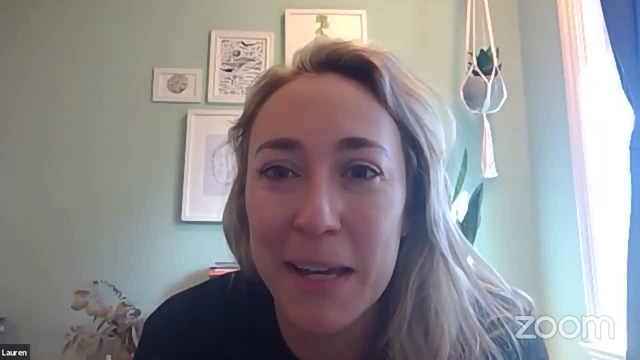 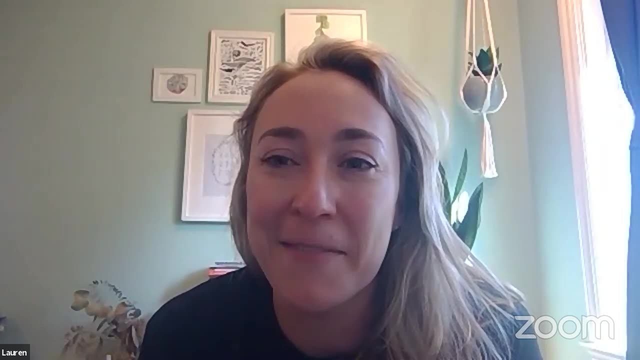 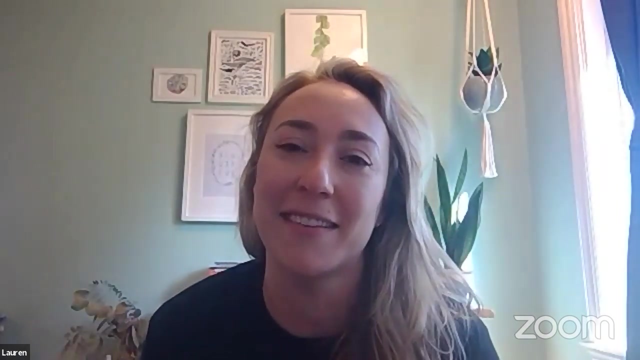 I feel really, really, really lucky right now to be able to spend some time with all of you. Many of us, probably all of us, are calling in from our homes, And it feels really good to be connected to you guys. I think we're really lucky to have access to technology that lets us hang out like this, So 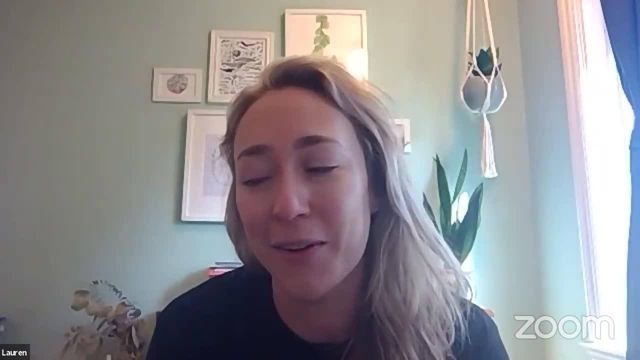 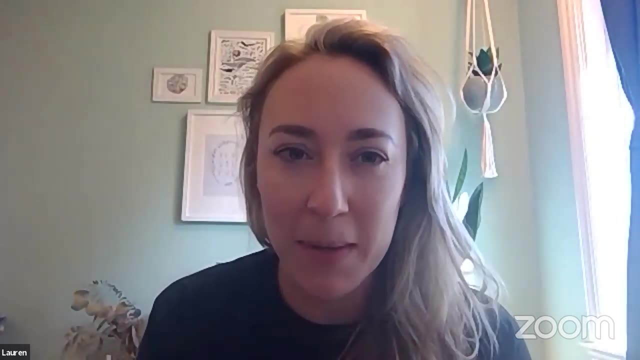 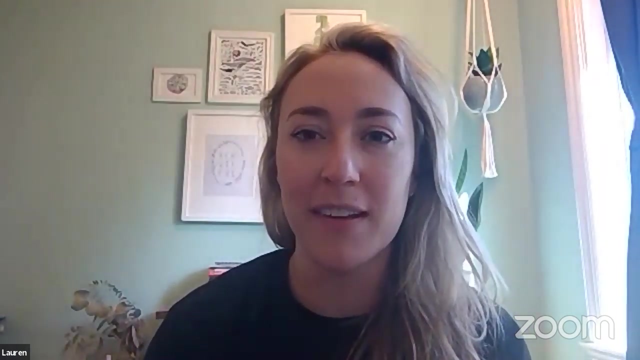 I'm really grateful to all of you for tuning in and for showing up. So, as Celeste said, my name is Lauren. I call myself a conservation scientist, which basically means that I work both with humans and the environment to try and better understand our world and how we can best protect it and help people and also wildlife and animals. 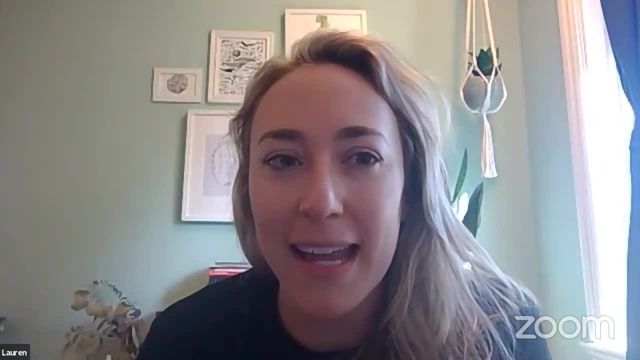 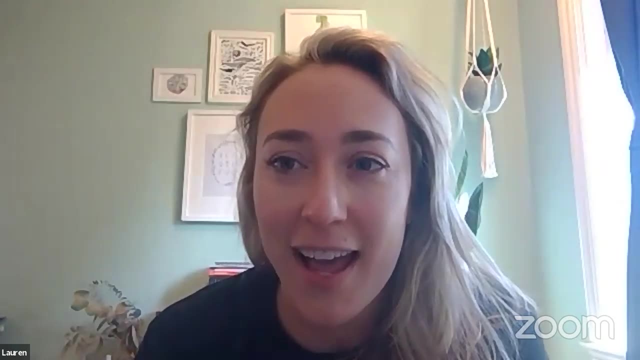 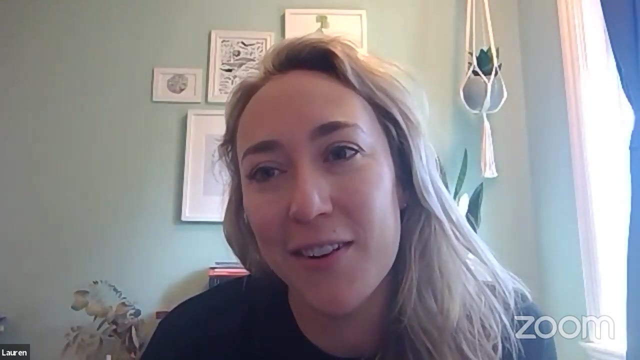 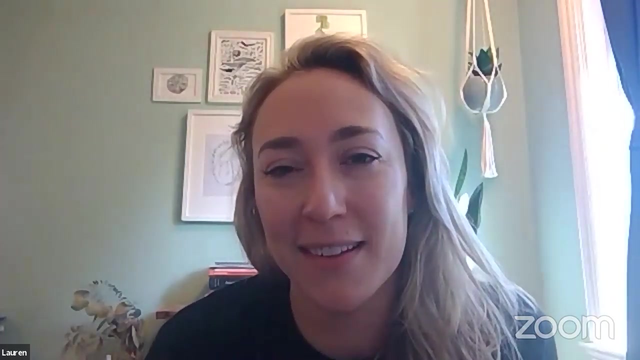 And I'm calling from Victoria, British Columbia, Canada, where I am a PhD student at the University of Victoria. But I actually was born in California and I grew up in Sioux City, Iowa- for those of you calling in from Iowa- And I went to the University of Notre Dame for my undergraduate. so I spent some time in South Bend, Indiana as well. So I have some fond memories of the places some of you are calling in from. 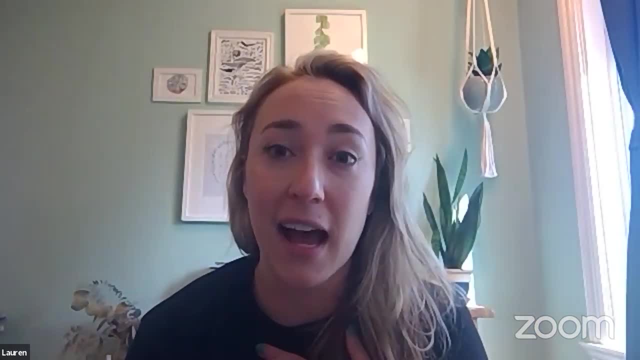 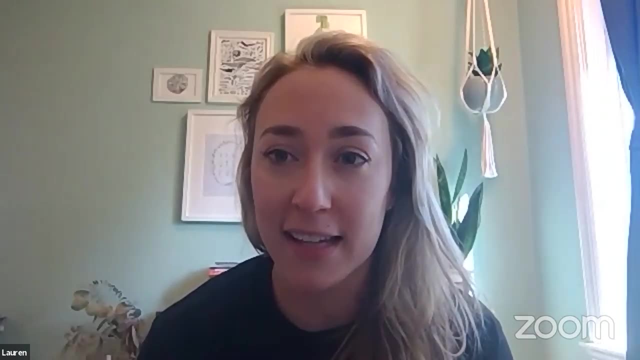 And I also want to take a moment to let you guys know that I'm calling from Victoria, but that that is also the traditional territories of the Coast Salish First Nations. So these are some of the places where I'm calling from. So I'm calling from Victoria, but that that is also the traditional territories of the Coast Salish First Nations. So these are. 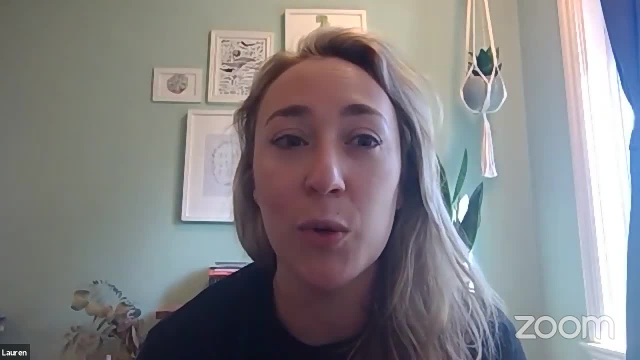 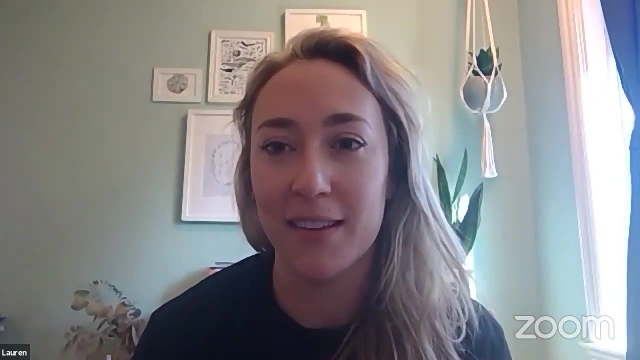 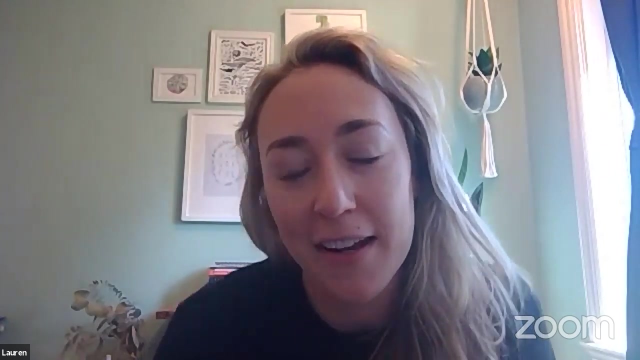 indigenous peoples which, like Native Americans who were here long before I was here and any of my colleagues were here- and continue to take care of the environment that we, as researchers, now study. So at the university, we always acknowledge that we're here as visitors on that territory, And I want to do it on this. 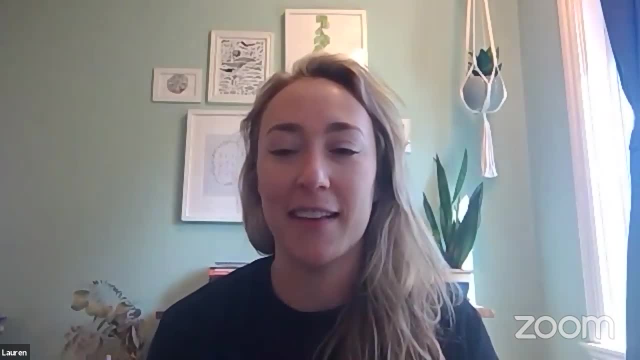 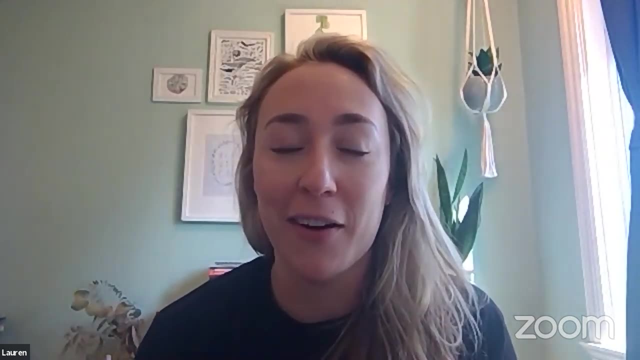 on this video call too. So now that I've done that little introduction, I'd like to share with you guys a little lesson- It should only be five or 10 minutes- about a research project project that I'm working on right now, that I've been reading a lot lately and that eventually, 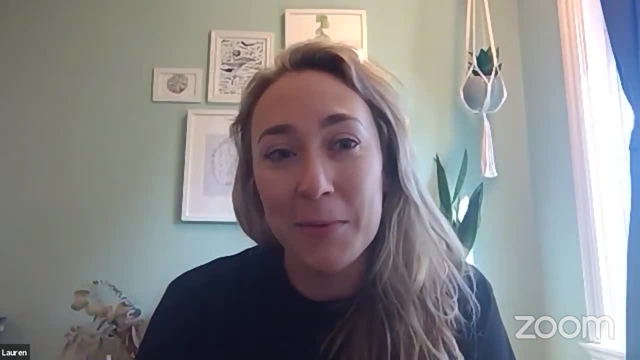 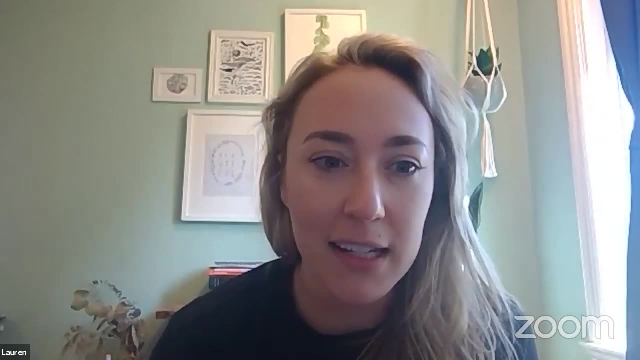 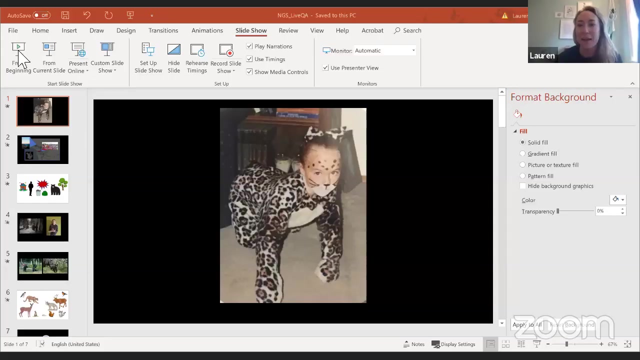 I'll go into the field to do some research on and then I'll open it up to questions and I'm really excited to hear what you guys have to ask. So I'm just gonna share my screen really quick with you guys and we're gonna start really really from um. we're gonna dig deep back into time to 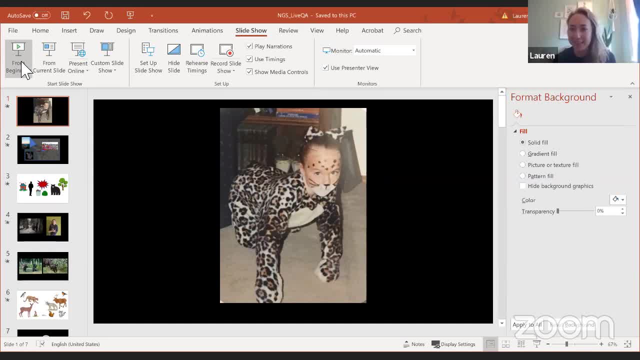 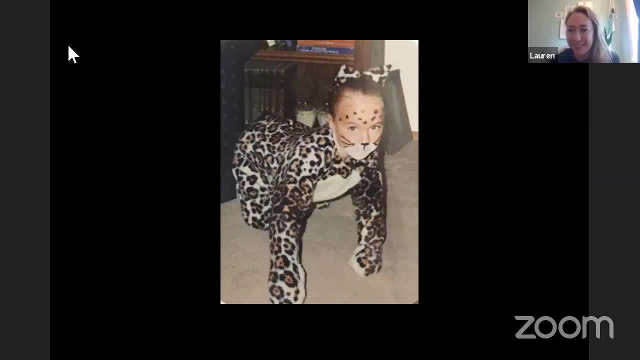 start this presentation today. So, like I said, I'm a conservation scientist and my whole life, as you can see from this image, I have cared a lot about wildlife. So when I was a little girl, I drove my parents crazy because until I was like 12 years old, I was never actually a human. I was always 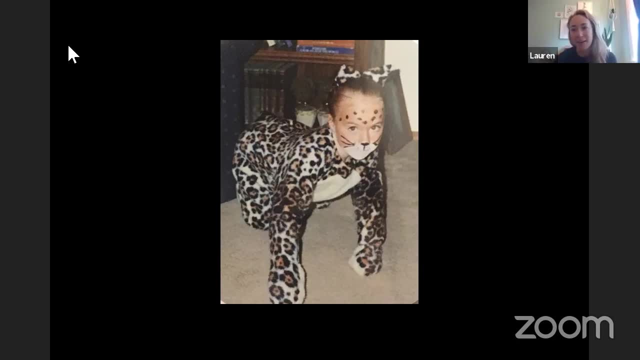 playing pretend to be some sort of wildlife animal, So my love for wildlife started at a really, really early age, as I'm sure the same can be said for everyone. So I'm going to share my screen right now and I'm going to start this presentation as if it's a really short video, but I'm going to 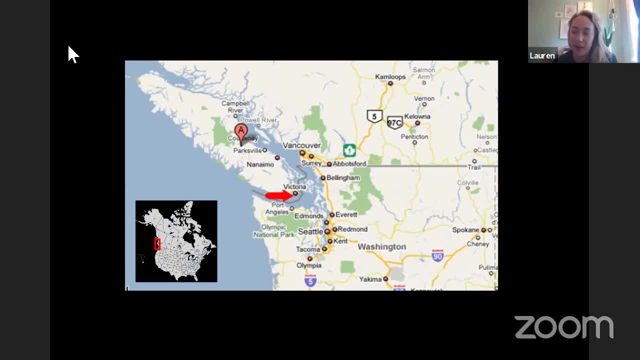 talk about a lot of the issues that I've been dealing with and the things that I've been struggling with so far. So I just wanted to show you really quickly where I'm calling from So you can see with this little red arrow pointing towards Victoria Canada. So I'm actually on a little 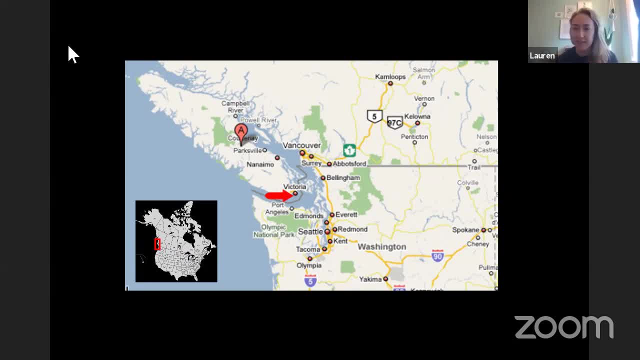 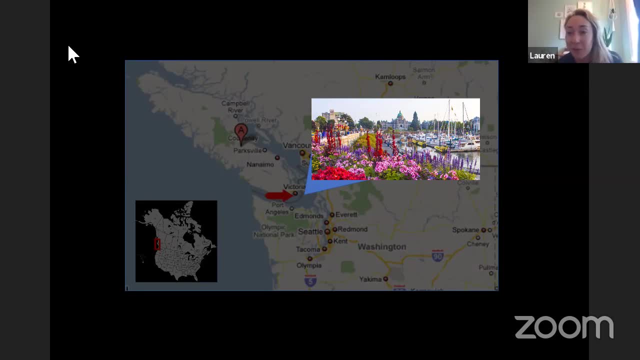 island called Vancouver Island. that's close to Washington state, and Victoria is the capital of British Columbia, and so here's a little picture of Victoria where I live. Outside of my window does not look like this, but it is a really beautiful city, quite warm and sunny right now. 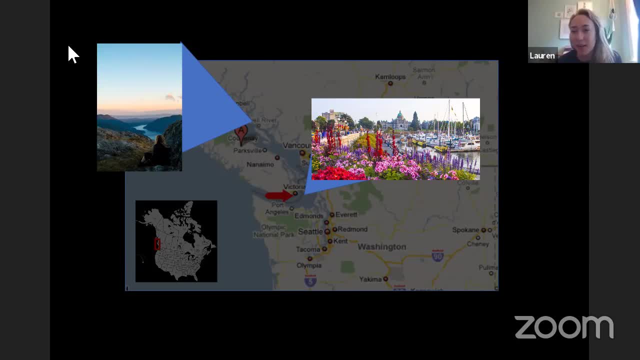 um, and so I'm going to share a little bit about where I live. So I'm going to start with a little, And the place that I'm going to do the work that I'm talking about in this presentation is called the Sunshine Coast of British Columbia. 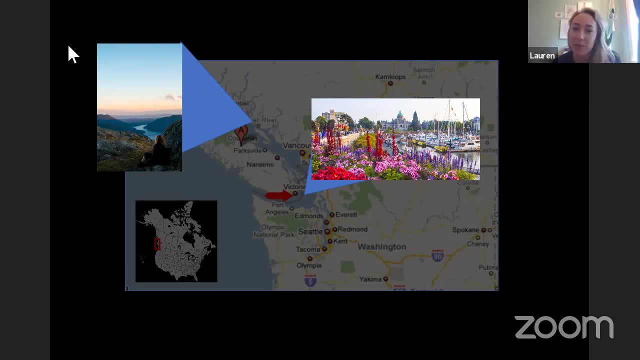 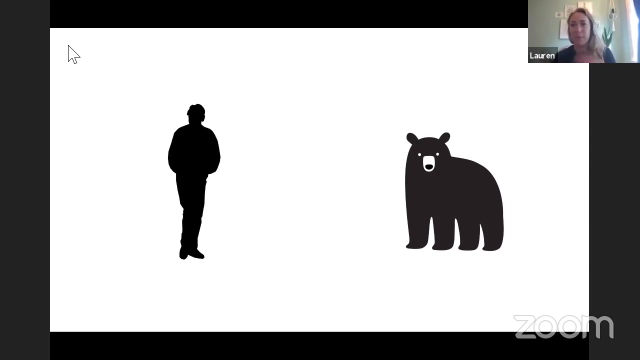 So a little bit colder than Australia's Sunshine Coast, but a really amazing place with lots of places where the ocean meets forest and where a lot of different sort of people live and work and play. And what I want to talk to you guys about briefly today in the realm of talking about 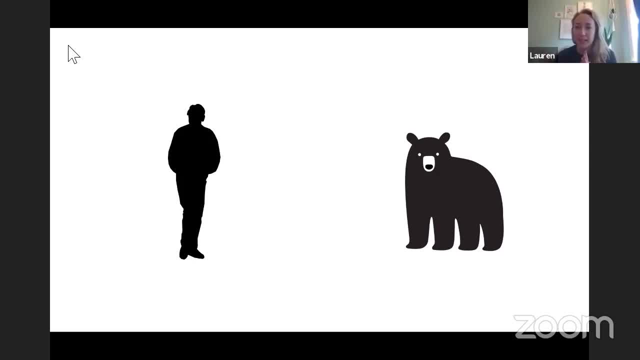 people and animals and the relationship between the two is human-wildlife conflict and human wildlife coexistence. So one thing I learned really, really early in my work and my reading and my learning as a conservation scientist is that when we're thinking about how to protect wildlife and 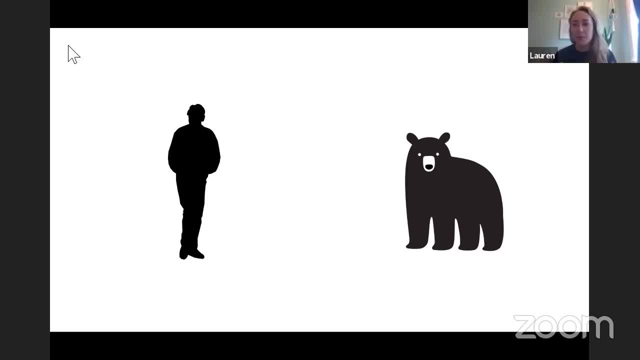 how to make people happy in this shared earth. we really need to think about our relationship with the wildlife in our own backyard, And for a lot of people in the US and people in Canada, the wildlife in our own backyard includes black bears. 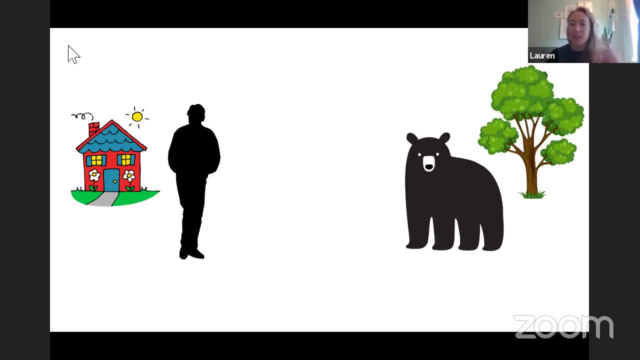 And so, When wildlife and people are living in their own homes, people in houses, and bears and forests and in habitats that they were born in, we have a pretty peaceful relationship with bears. We can coexist, as they say, But that gets trickier and trickier as there are more and more people filling up and spreading. 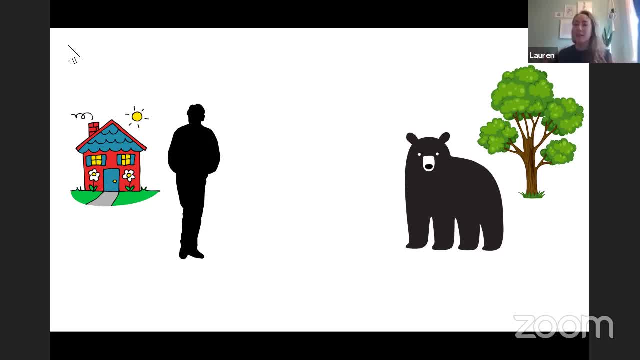 out from cities, right, And there are more bears who are hungry coming into towns looking for food, And so an increasing worry for a lot of Canadians where I live is that they're not able to live. Is that when people leave things out like garbage, or when bears come into town because 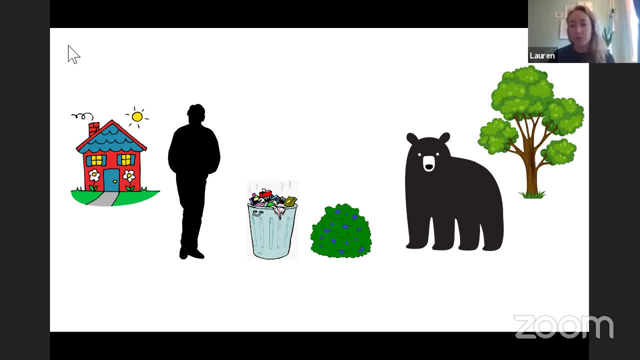 there's really yummy berry bushes or ripe fruit trees, you end up getting conflict between bears and humans, And conflict in general isn't necessarily a pleasant experience for anyone. But when conflict happens between wildlife and people, it's often the wildlife that pay the biggest price right. 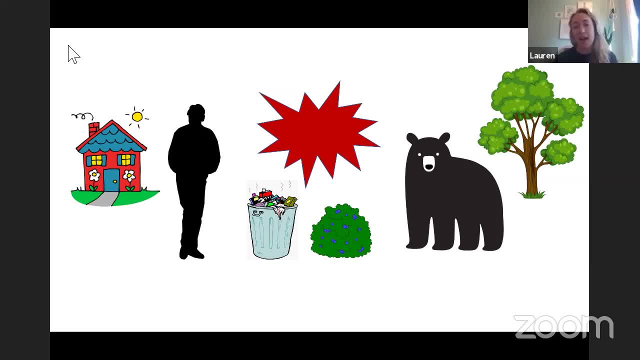 So bears can either be injured, they can be hurt. They will have to be moved if they keep coming into someone's backyard And in some cases, if they're showing up over and over again, they can actually end up being killed. So it's really really important that, both for people who don't want their houses or 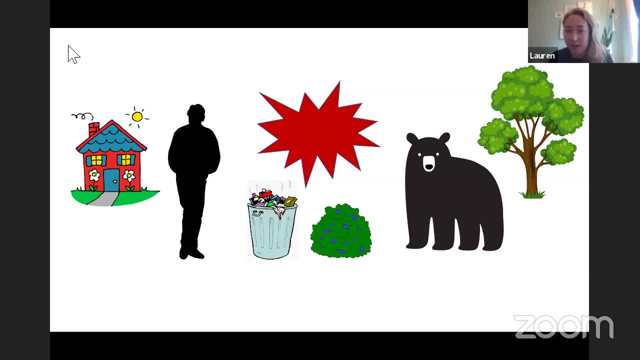 their property to be damaged or their garbage to be turned upside down, and for bears that we make sure that we are finding ways to stay peaceful together, even as we increasingly start to share space, And so there are a couple of things that we can do. 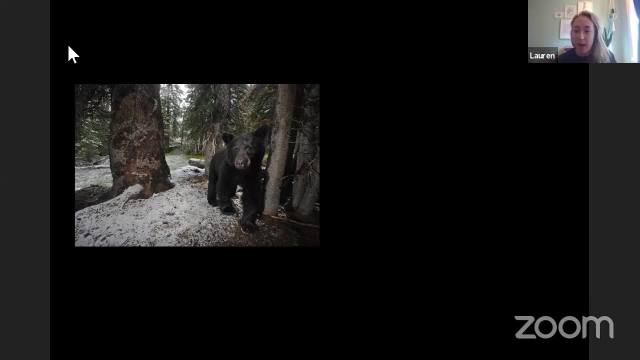 A couple ways I, as a scientist, can learn more about how to solve these problems where bears and humans are coming into conflict, And one of those ways is to set up wildlife cameras, like this one here that I'm showing on my screen, where you can actually capture images of black bears. 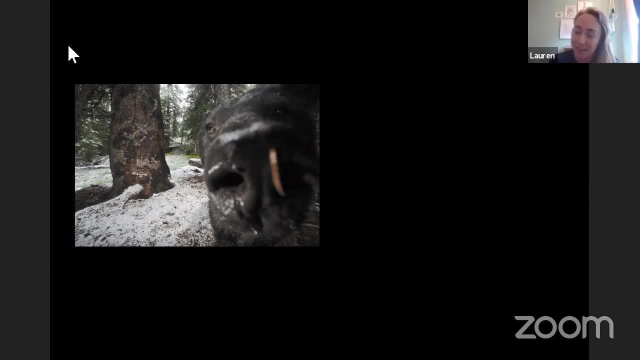 Black bears are very curious and, yes, this one has found and is sniffing the camera. You can understand where the bears are, what they're doing. if they're in people's backyard, Are they looking for garbage? Are they just passing through? 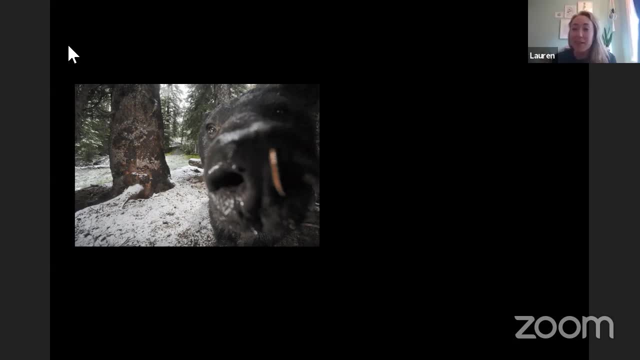 So you can learn a lot about black bears. There's someone really important that we also need to learn about if we want to understand the relationship between bears and humans, But sometimes we forget when we're talking about protecting wildlife, and that is humans. 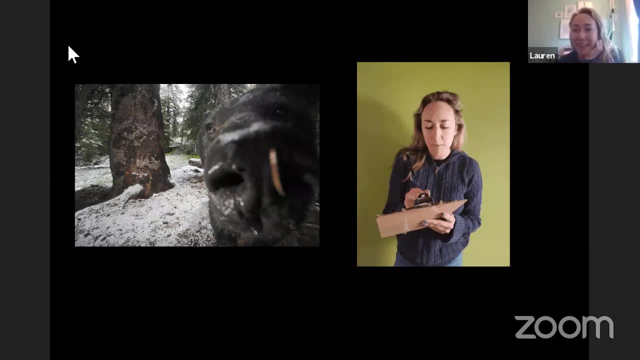 So what I do is something a lot like this: in Supermotion, I go around to households with a clipboard and a pen and a list of questions and I ask people about their experiences with bears, about how they value bears, why bears are important to them, what trouble they're having with bears. are bears getting their garbage? 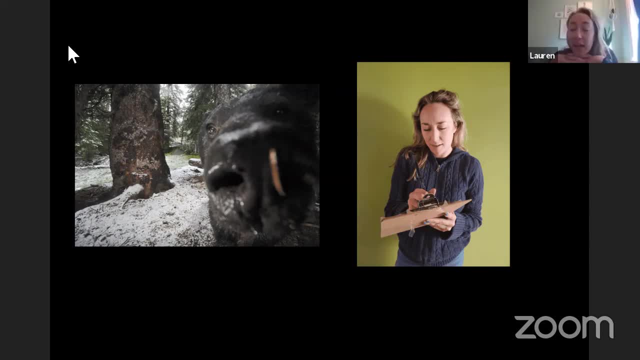 cans, are they getting their food? And I also ask people about: in their perfect world, what would their relationship with bears look like? So it's really important to not only understand where bears are and what they're doing and how many there are, but also how people are behaving around bears, what they're scared. 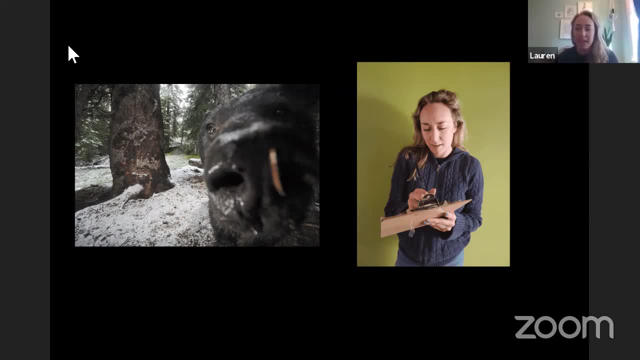 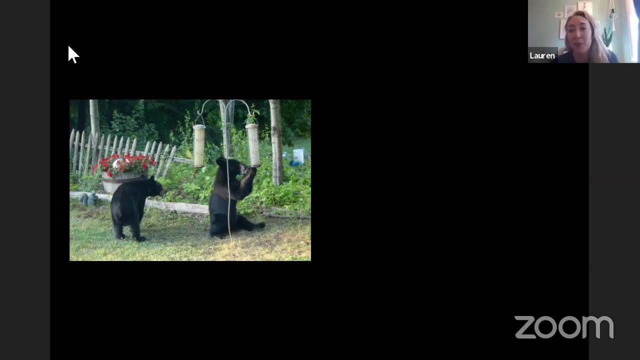 of what they're hopeful for, what they care about, And so we end up with a lot of different scenarios with bears when they come into conflict or into coexistence with people. And, as you can see in this image, these bears have found a bird feeder with some seeds. 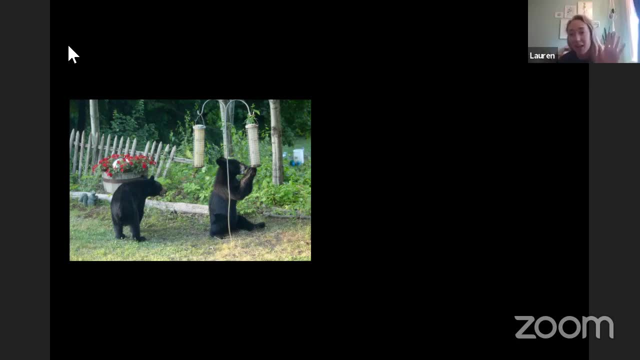 So, while this image may look really, really cute to us- and, I'm not going to lie, I think this is very cute too- we actually have to, as scientists and as people who share yards with wildlife, actually get into the mindset of that bear. 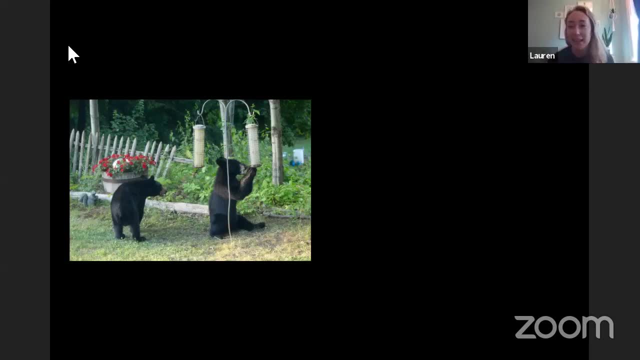 And think about. Think about how living like this, eating food from people's backyard, can damage them. And while this is a really cute image, it's also a really scary one for these bears, Because if these bears get used to finding food in someone's backyard, the chances is 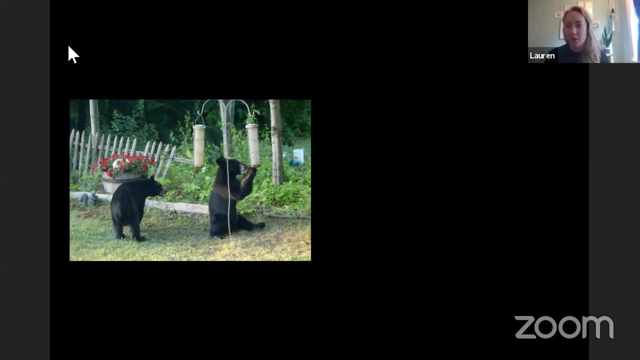 just like we would if we found like a really great burger joint around the corner. we would keep going back over and over again And once those bears start getting bigger and are a little bit less cute, or if they say, uproot that bird feeder stand. 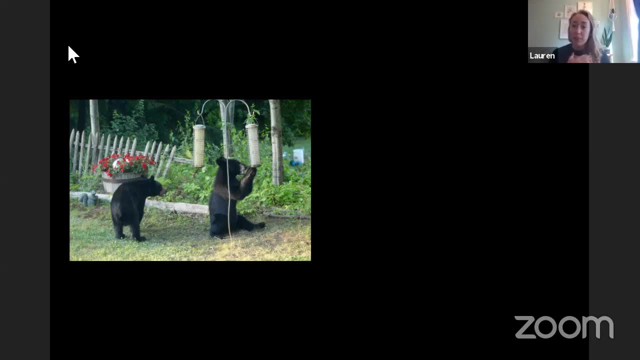 Only we're in trouble because the bears are causing damage And now the people are at risk who live in that yard And the bears are at risk who have been visiting that yard their whole lives. So what we really want to work towards as people in community with bears is something: 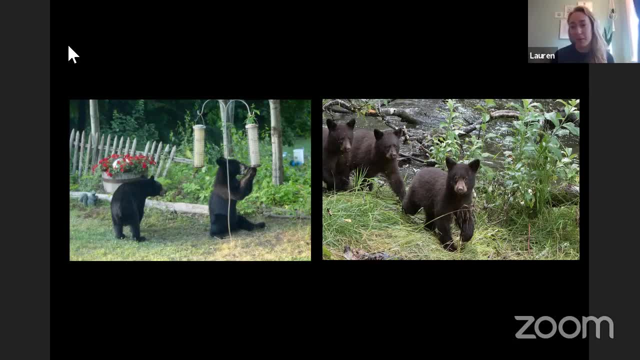 more like this, And here you see three very cute black bear cubs sort of in nature on their own, with lots of space. So, even though many of us love wildlife so much and want to see them more often, one part of my research is working towards ways that we can respect them. 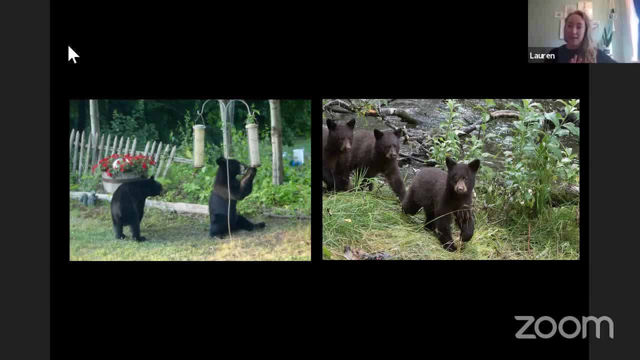 Respect wildlife while also giving them tons of space. right, Because the healthiest, happiest bear is unfortunately actually the one we don't see in our backyard, And so this is just a really really like small window into thinking about relationships between human and wildlife. 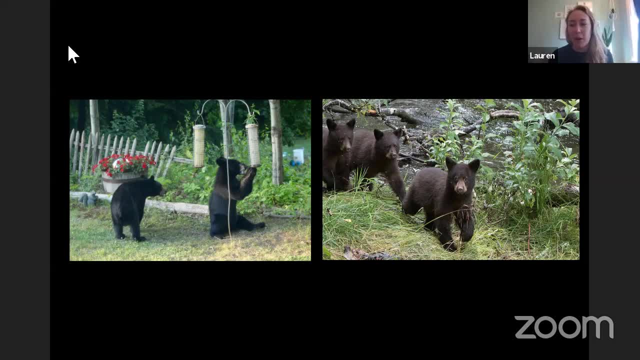 This is a really important, really visible one, because of how big black bears are and how serious conflict can get with black bears, between humans and black bears. Um, But I I want to encourage you guys now to think about all of your relationships with. 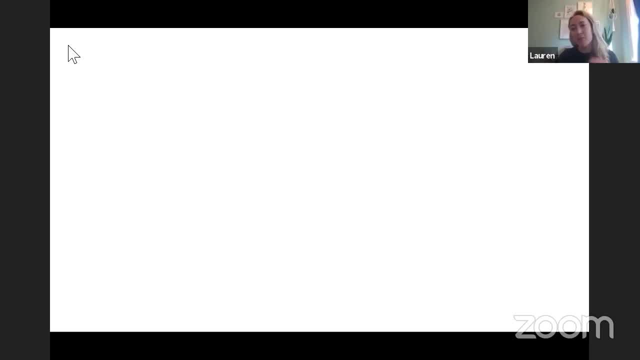 wildlife where you live. It's really easy to forget, when we're going to school and going to work, or living in the city, um, or living in our houses, that every day we exist in the world, we're in relationship with the wildlife all around us. 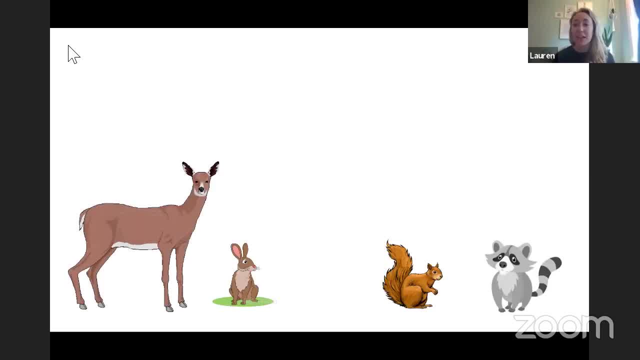 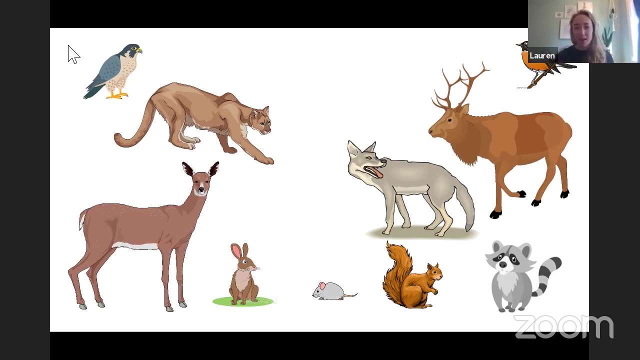 And so that can look like deer and rabbits, that can look like squirrels and raccoons, mice and coyotes- Yeah, Cougars, in some places, elk birds. wildlife is all around us all the time. It doesn't have to be a black bear for us to want to find opportunities to have good. 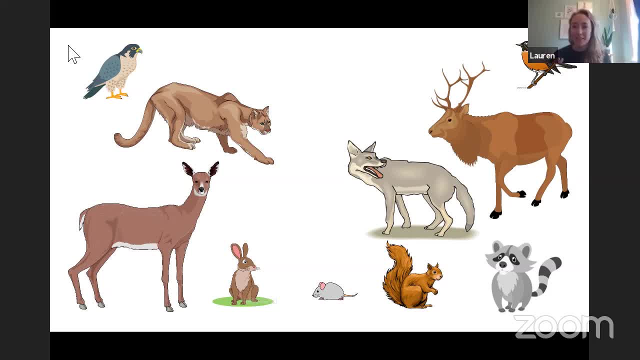 relationships with those wildlife, And so what I really like to talk to you guys about today and think about in the questions is: what are the wildlife in your own backyard? What is your relationship with the Robin that comes and gets worms out from, from the grass? 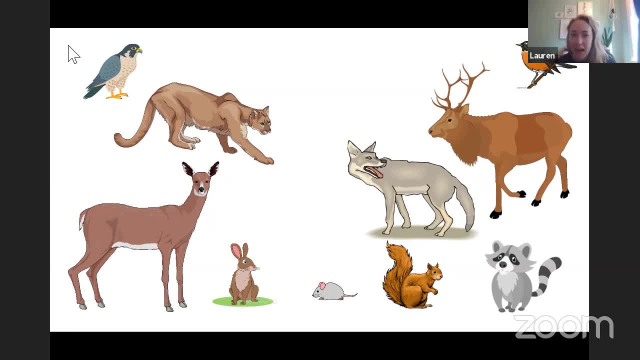 in your yard, that squirrel that nest in your tree every year. How can you improve that squirrel's life and make sure that you are avoiding conflict with the mice that live in your city, or the rabbit that eats your garden, or the deer that keeps jumping over your butts? 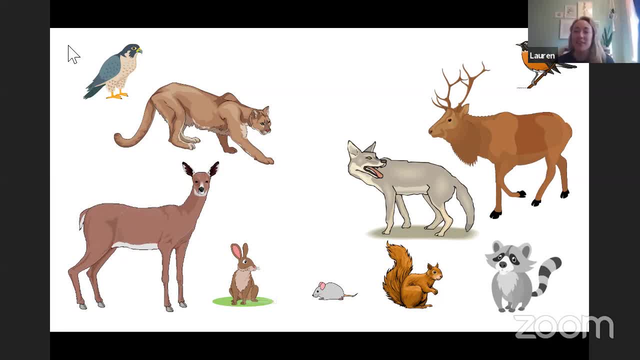 And so I want to. yeah, I'm going to leave this part to you guys. I'd love to hear from some of the classrooms and the households that are tuned in on the wildlife in your yard and what you think about your relationships with that wildlife, how. 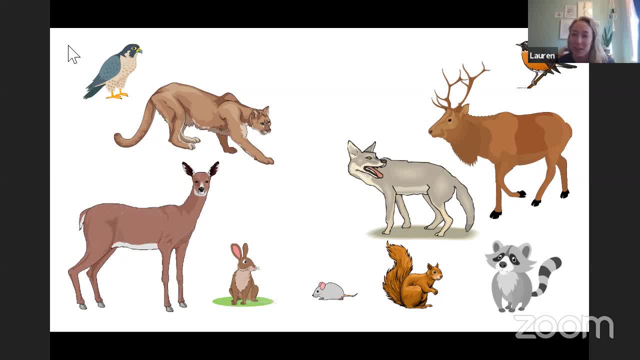 we can build better relationships in our human and wildlife communities By thinking about our behavior in them and what we value and how those animals might feel in these spaces that we've come to dominate. as they're sort of treed, forested habitats increasingly disappear. 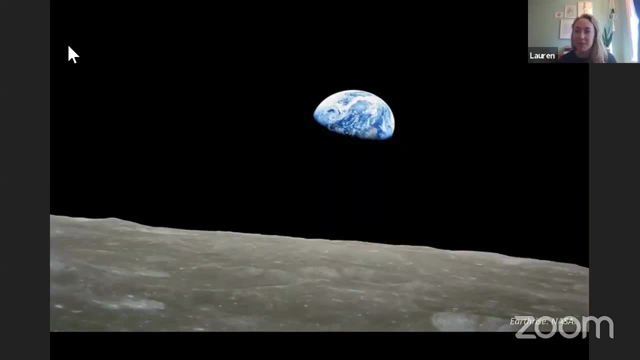 So I'll leave that to you guys, But just wanted to end by saying, when we think about our relationship with wildlife, what we're really thinking about is the fact that every single one of us, each of us on this call right now, and all of the wildlife we see every single day, whether it's the 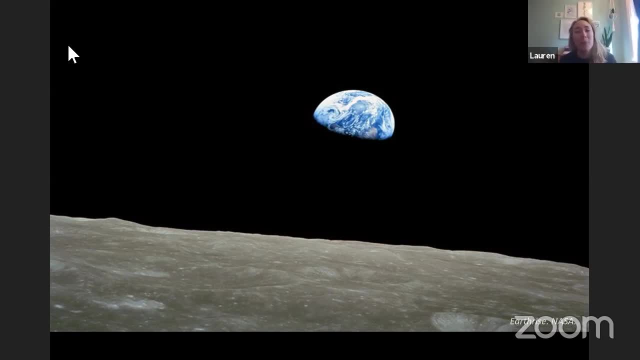 grizzly bear or whether it's a mouse, we all share this planet and we have a limited amount of space, And so being in relationship with wild animals and thinking of how to make those relationships best for people who live in communities and need to be able to thrive and be happy, and 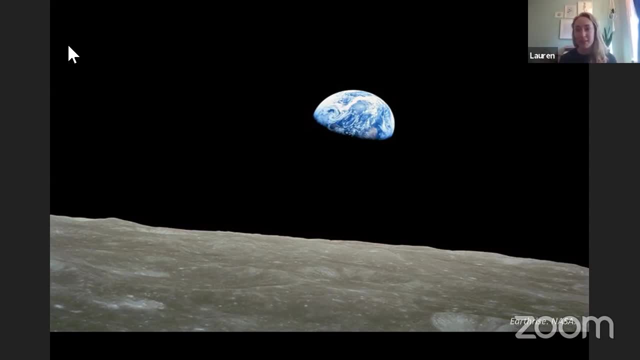 want to be safe, but also for wildlife, who want very similar things, that we're all in this together, wildlife and humans. Yeah, I think we have such a cool opportunity right now with all the technology and science and brilliant young minds. we have to think about how to better define those relationships with. 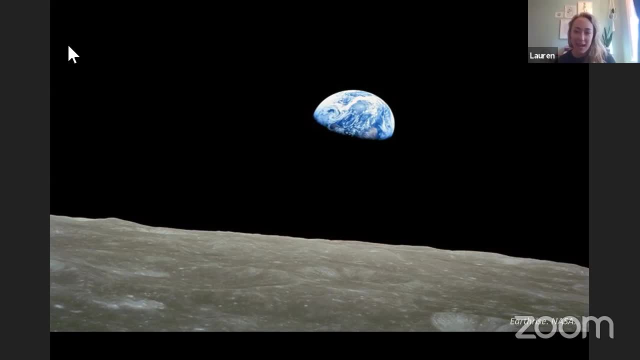 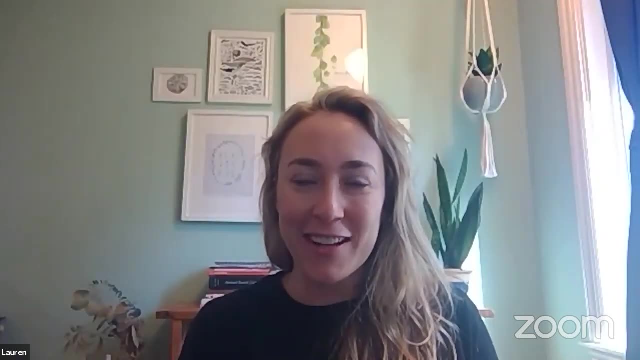 wildlife so we can all live together peacefully. So with that, I'm going to stop sharing my screen. Yeah, I'll come back to you guys and get some questions from all of you and from Celeste. That was amazing, Thank you. 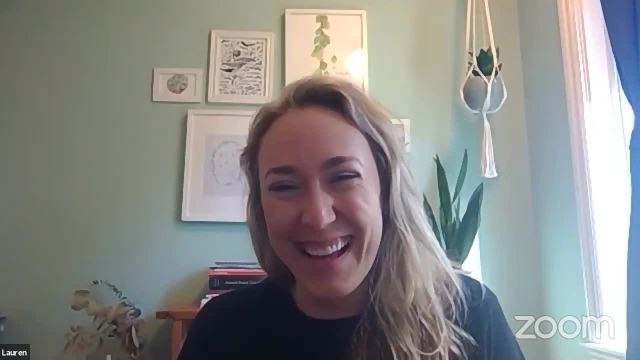 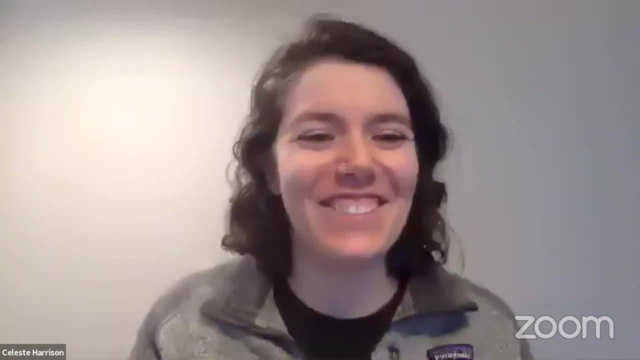 I think everybody out there is incredibly jealous of your job right now. It's amazing to think about those adorable little baby black bears all day and how to protect them For folks at home. whatever you took from that, it doesn't have to be baby bears- we. 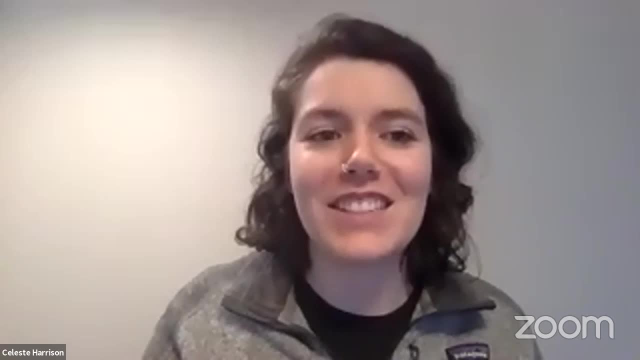 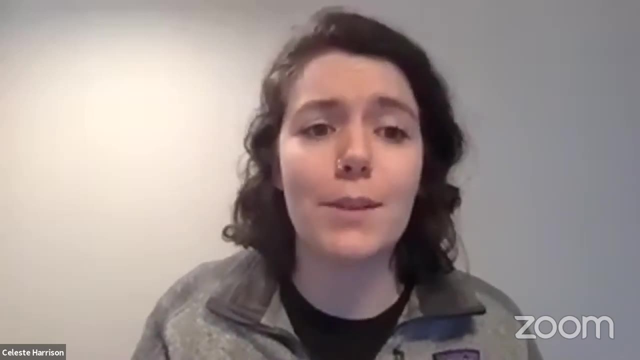 are challenging you to do a little activity for us later this afternoon. So, if you're in grade K through five, we're challenging you to draw a picture or a comic strip of something that you learned from Lauren today. If you're in grades five through eight, your challenge for the afternoon is to write a. 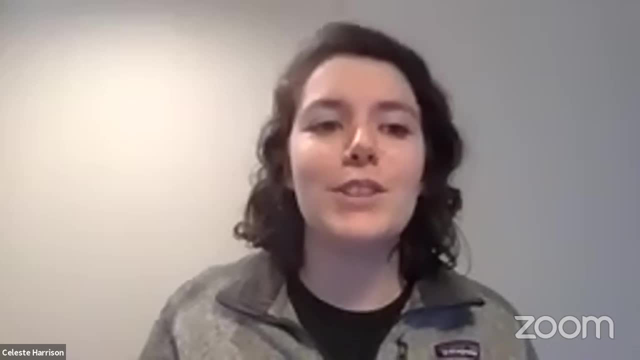 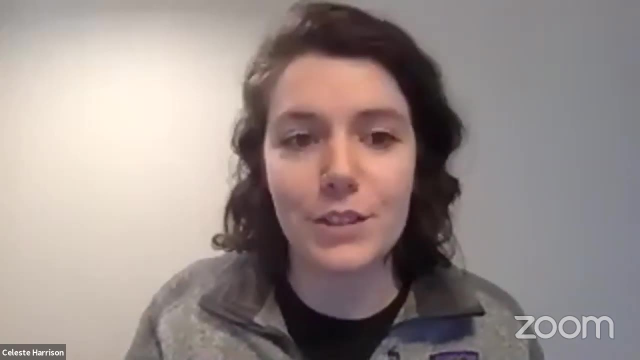 news article about her or her work. And if you're in high school, your challenge from us is to produce a short video that explains something that you learned today to a new audience, something that you could share with your friends or your family. So if you're going to participate and you're willing to share those amazing materials, you 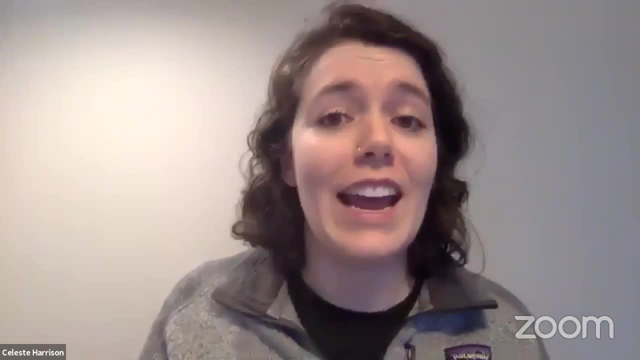 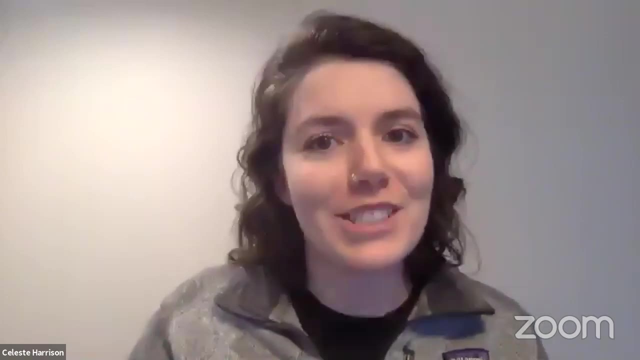 make. please tag us at NatGeoEducation and hashtag explore classroom, so we can make sure Lauren gets a chance to see them all. But now I think it's time for some questions. So if you're watching online, you can totally ask questions too. 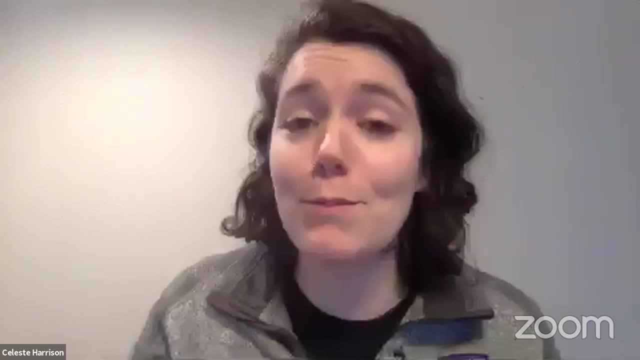 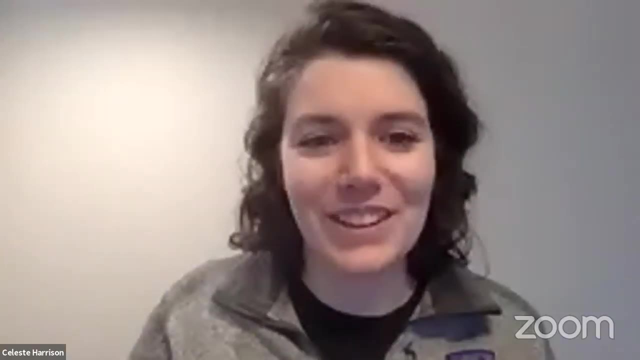 Okay, I saw all of those chats coming in. People in New Jersey are very excited. Use that chat bar for questions too. Anything that you want to know, we'll ask Lauren in a minute And for my folks on screen with me, get ready with your nice loud voice. 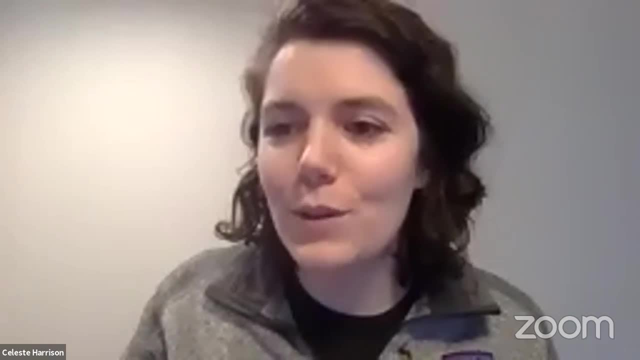 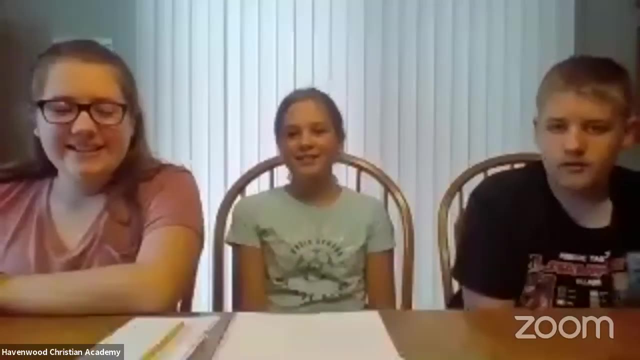 We're going to start visiting households and teachers. Why don't we start with the Havenwood Christian Academy? Your microphone's on. Do you guys have a question? Hi, We were wondering how long Lauren has been in the classroom. I'm sorry. 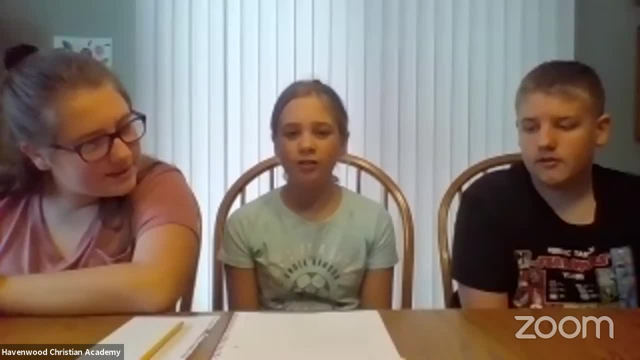 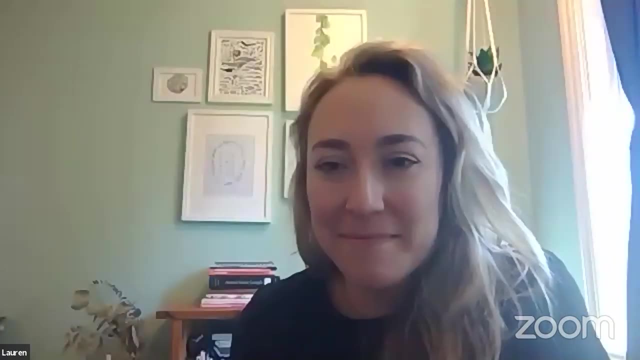 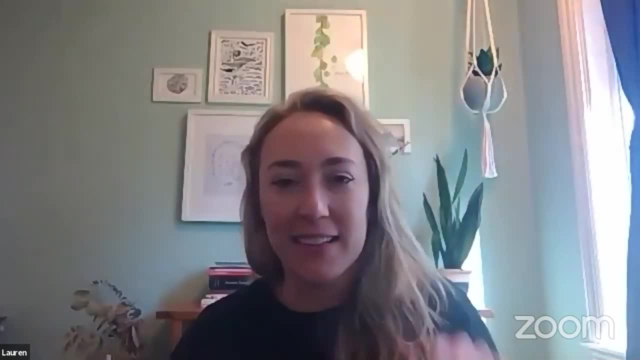 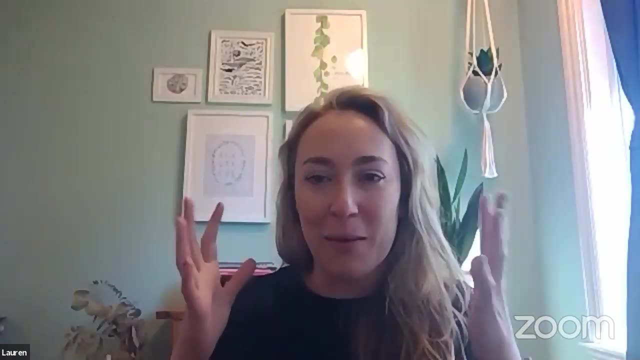 As I showed in that image where I was like walking around like a leopard, as a little kid. I sort of feel like because I love my job so much and I think about wildlife in my spare time, like not when I'm working. I've sort of been doing my job my whole life. 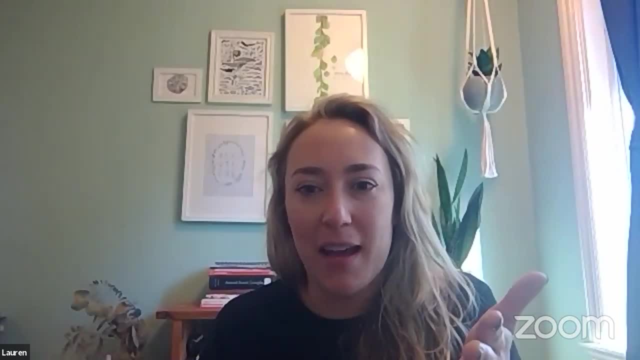 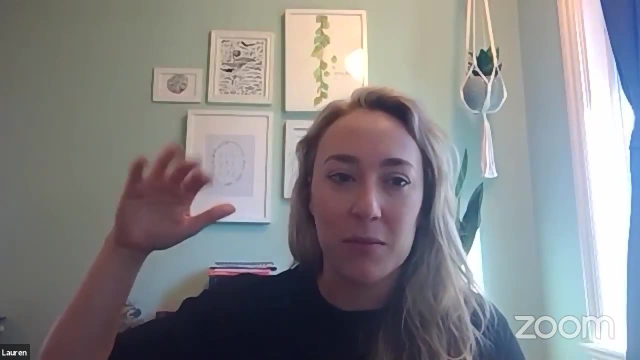 So when I was really young, I would. I would not only drive my parents crazy by, you know, by wanting to pretend I was a cheetah at all times, but I would also go to the library and not be able to decide on which books to take home, and bring home a stack of books. 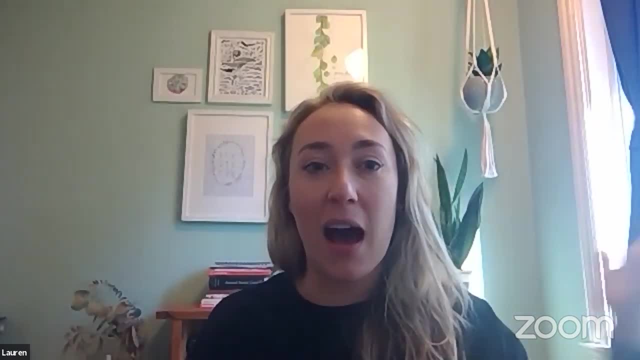 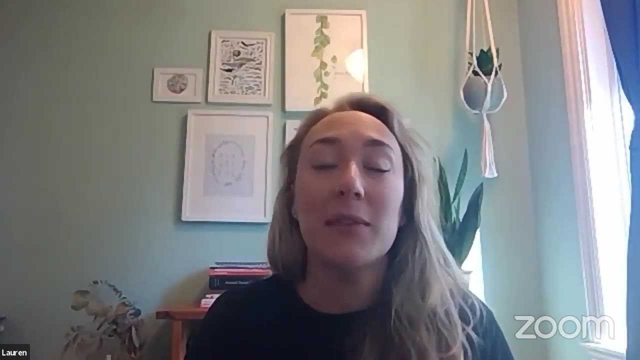 about wildlife. So I've really been curious about how to protect nature and and how to learn more about wildlife my whole life. But I so. when I was 18, I went to the. that was 10 years ago. I went to the University. 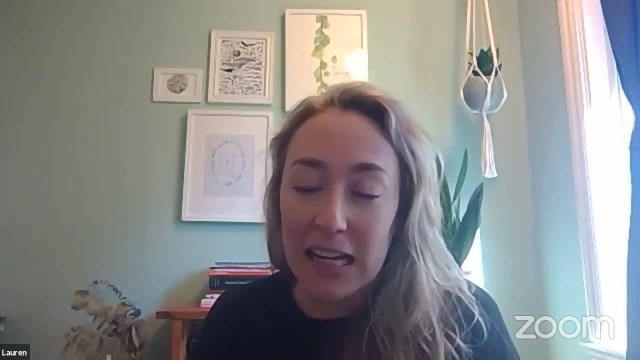 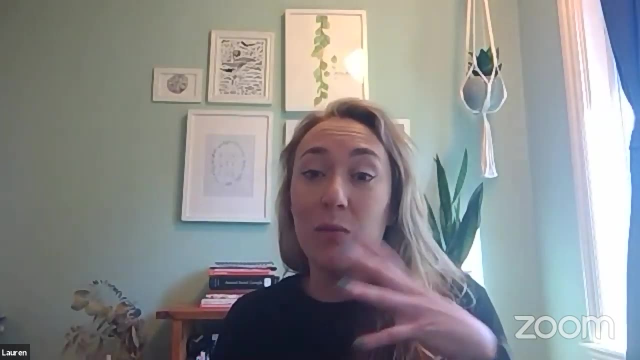 of Notre Dame and I did a environmental science degree there And and so that was when I really started doing work. So during that time I went out and I I worked on field projects that did all other people's research, but I acted as an assistant. 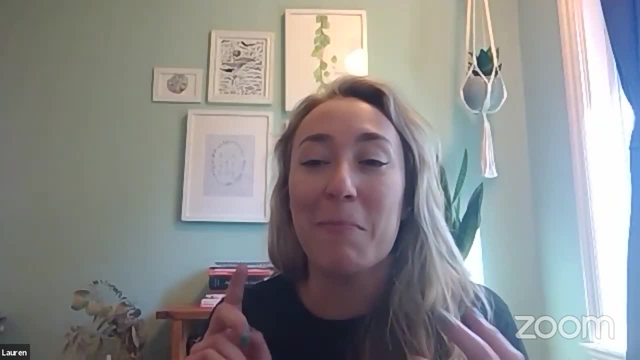 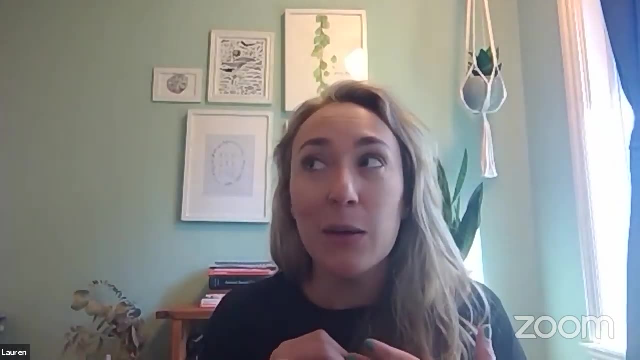 So I got to study kit foxes in Utah and mice in the in the upper peninsula of Michigan, Wisconsin, And I got to study monkeys in Brazil. So probably I'd say I've been doing some version of the work I'm doing now for about 10 years. 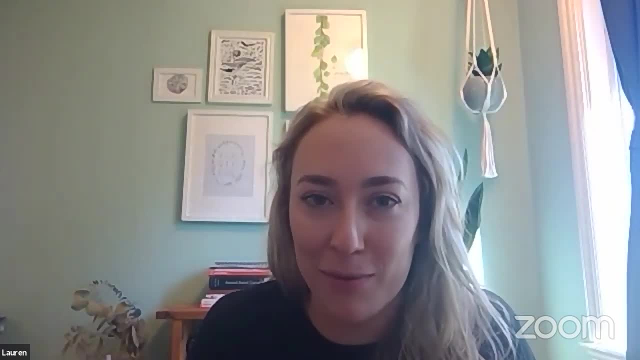 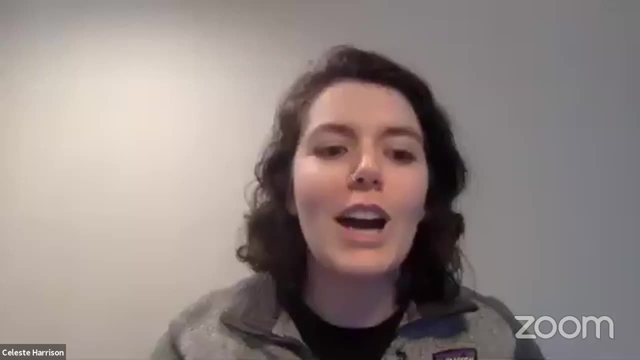 but I'm really lucky to do what I love, And so I kind of feel like I'm doing it. Yeah, Yeah, Yeah, Yeah. I feel like I've been learning about this stuff- always Awesome. We've got tons and tons of questions pouring in online. 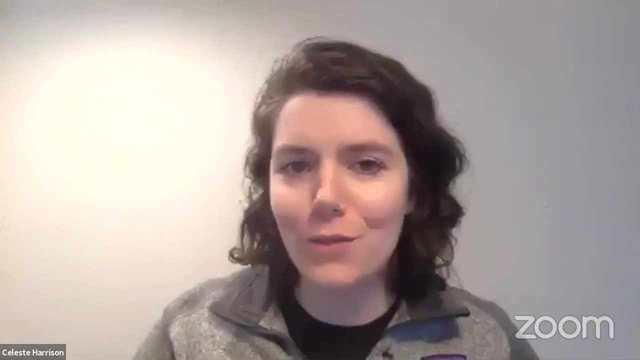 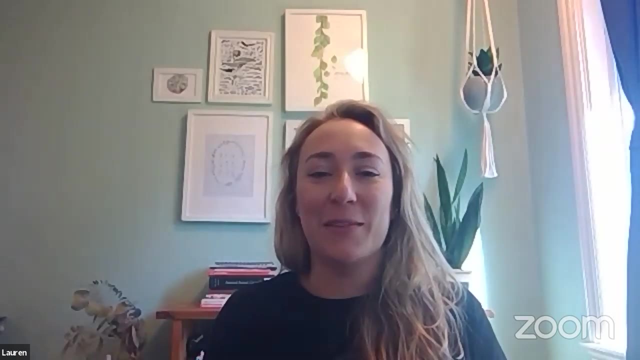 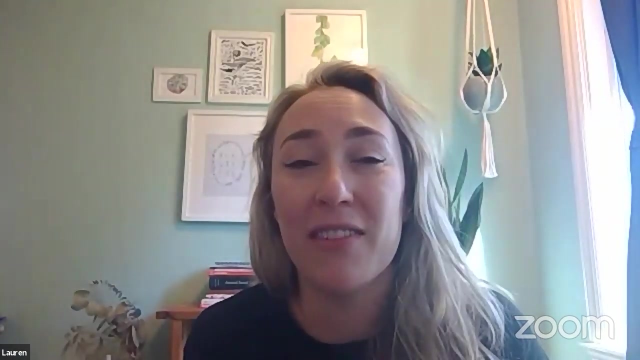 Thank you, Keep those coming. Allie Glenn from our YouTube audience is wondering if you have a favorite animal and if you've gotten a chance to study it. Oh gosh, That is a really, really, really hard question. I have two dogs at home with me and they're my favorite. like individual animals. 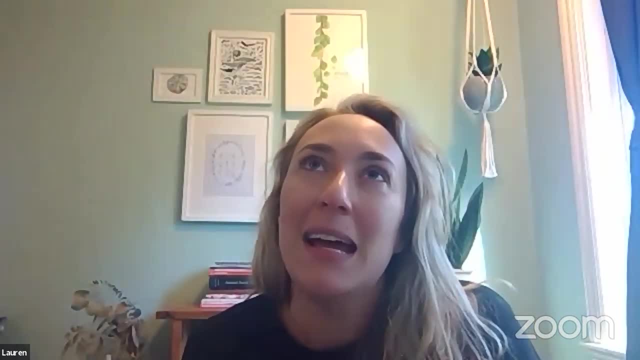 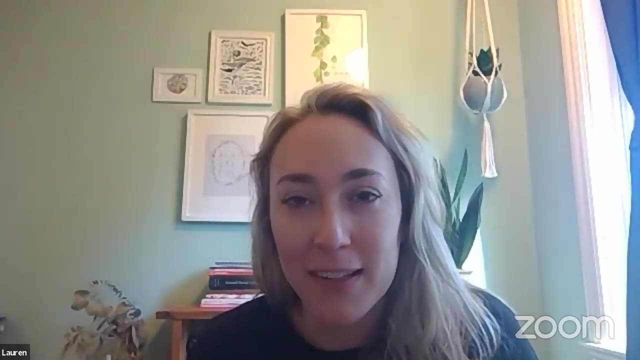 I'm really lucky to have them, Especially now with so much time at home. I think I have to stay true to my seven year old self and say that my favorite species of animal is the cheetah. I haven't gotten to study the cheetah, but I have a long career in wildlife science ahead. 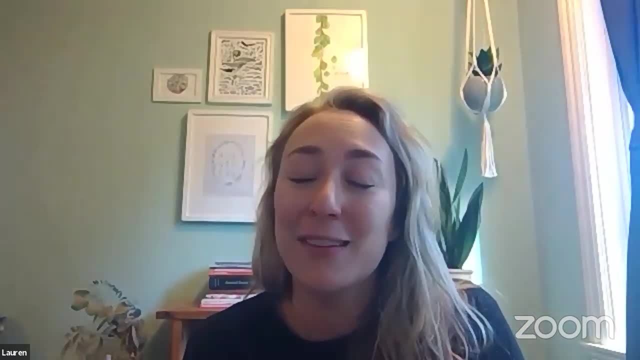 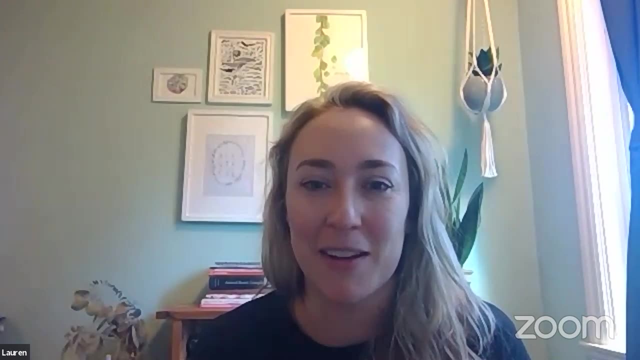 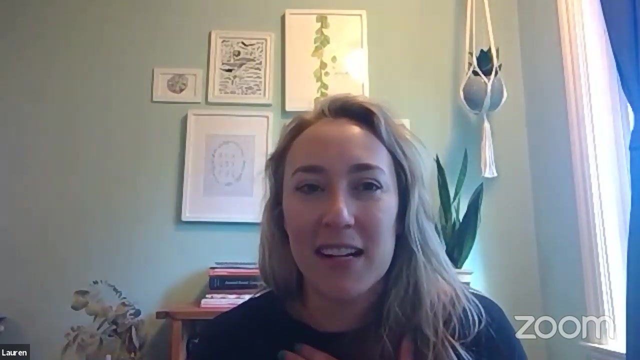 of me, So maybe someday I'll be able to. but I also feel really lucky that the internet exists because I have got to spend so much time watching videos and documentaries and reading other researchers work about cheetahs, And I also feel like I really like studying the animals in my own backyard and where I 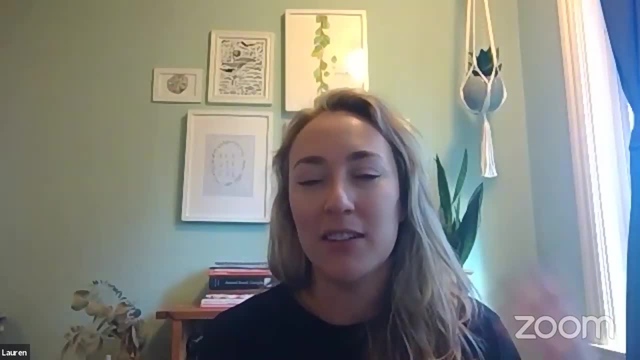 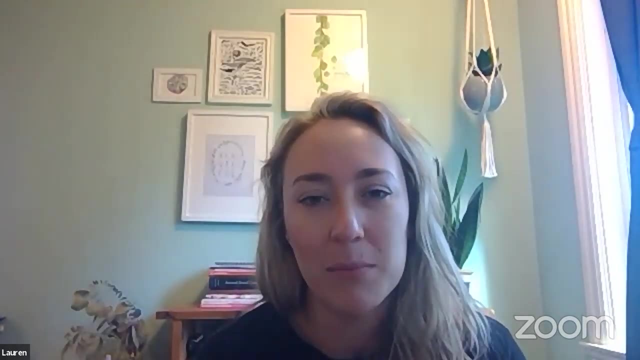 live right now. black bears are very much in our backyard and are also really incredible animals. So it's a little bit of a cop out answer, but I love them all. Cheetahs are probably my favorite. We'll still take it. 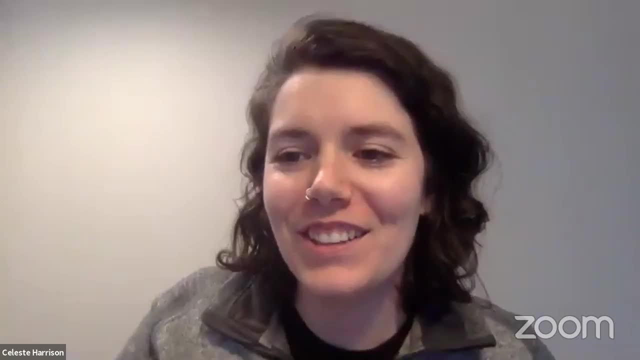 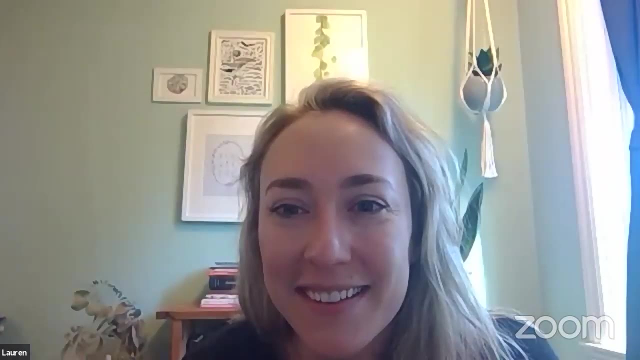 I love it. Let's go to the Olson family for our next question: Your microphone's on What is the most challenging part of the job. Oh my gosh, That's a good question. Hmm, Okay, I have two answers. 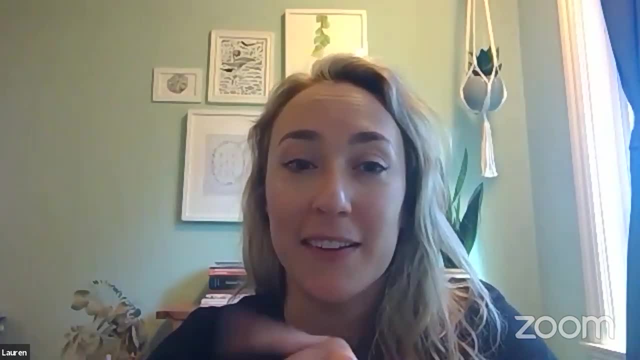 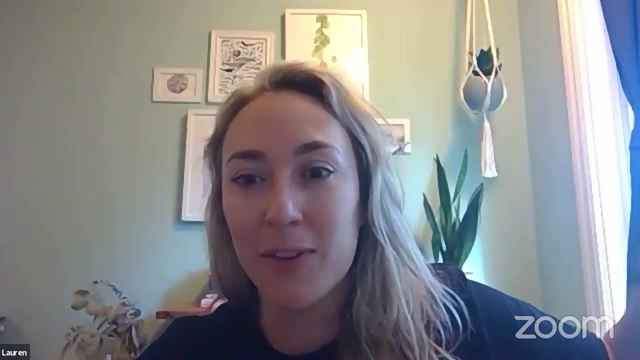 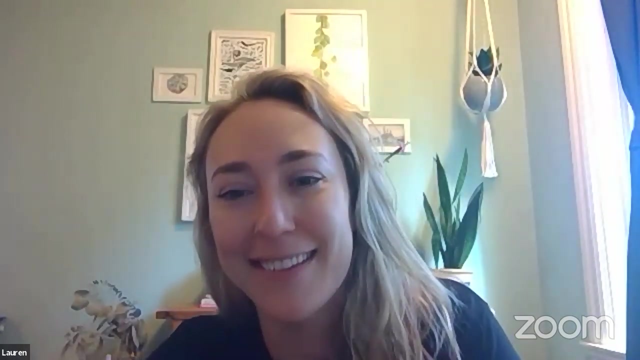 I'd say. one answer is that I'm really lucky and that I get to go into the field a lot and set up cameras and watch animals and talk to people, But about half of the year I actually spend sitting at a desk answering emails and reading. 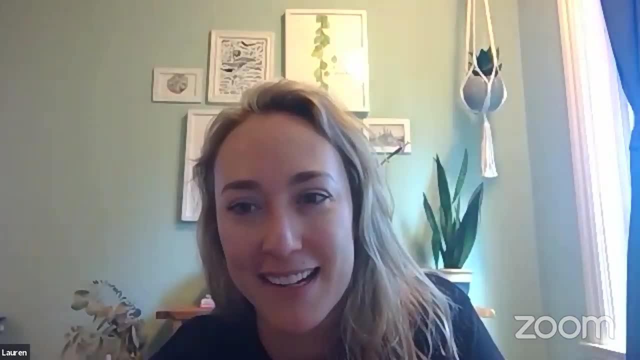 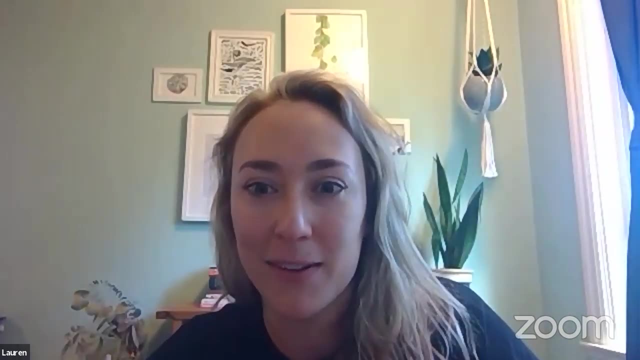 and reading, and reading, and writing, and writing, and writing. And for someone who loves being outside, that can be challenging. Yeah, For someone who loves being outside, that can be really hard, But doing that work is what enables us, as scientists, to go outside and research wildlife. 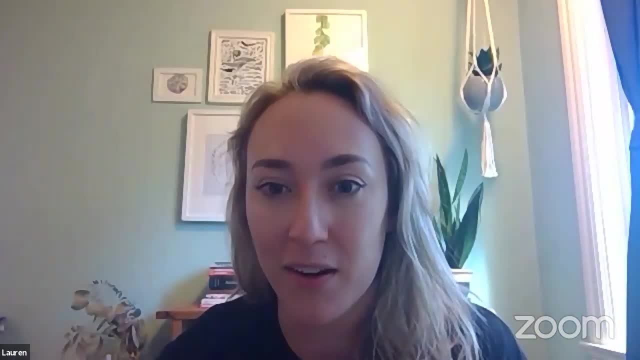 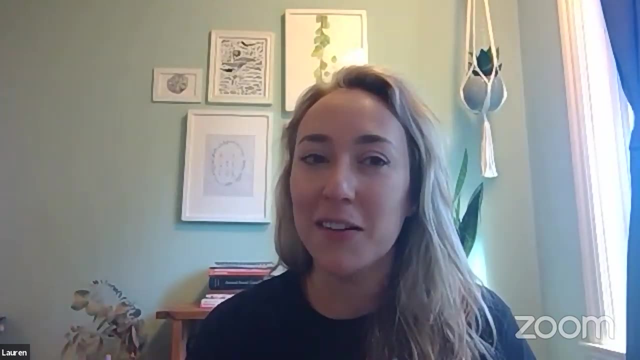 And it is also how we share the information. we learn right Once we collect our science. the way we share it is by writing about it and reading about what other people have done, But it's hard sometimes to sit inside and sit at a desk. 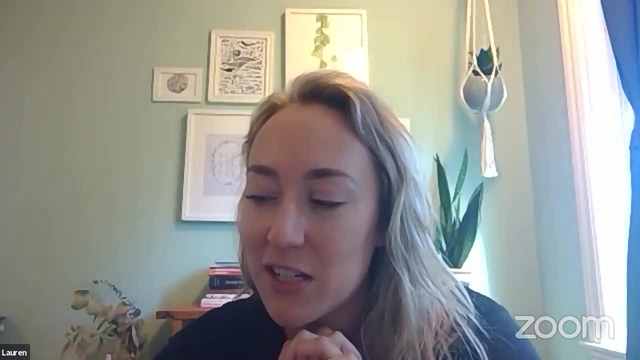 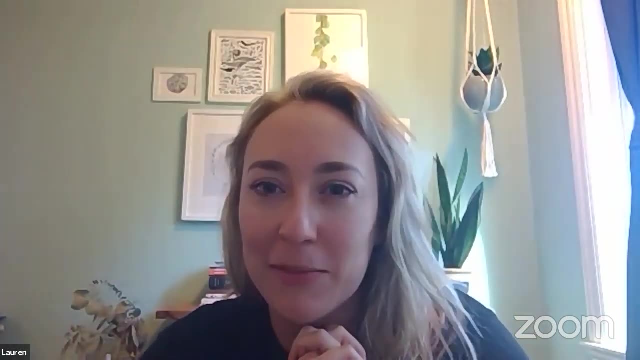 And I'd say the other hard part of the other challenging part of my job is just worrying about the wildlife. I care about Worrying about the world. I'm sure many of you do too. There are a lot of really good reasons to be hopeful. 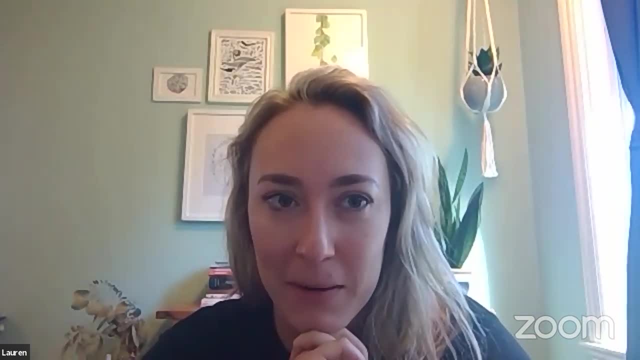 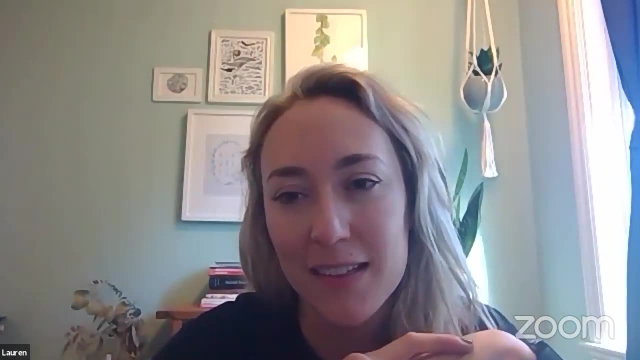 But there are some hard days when you know that black bear maybe goes into someone's yard again and knocks over a garbage can, Or you hear about, you know, another species endangered. So that's definitely a hard part of the work. 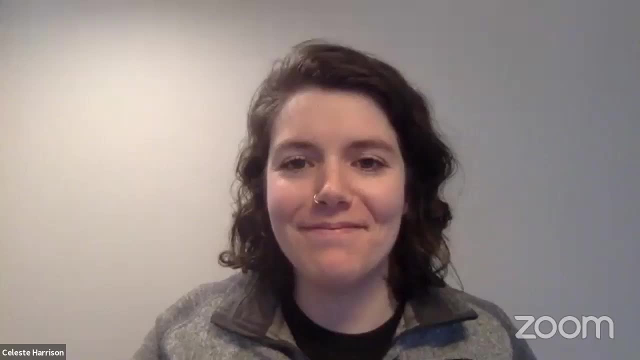 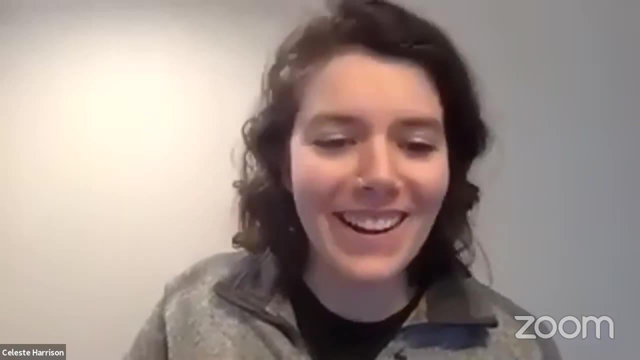 That's a great question. Let's take our next question from Ms Fisher. I'm going to turn your microphone on. Feel free to give your kids at home a shout out And then go ahead and ask a question for them- Awesome. 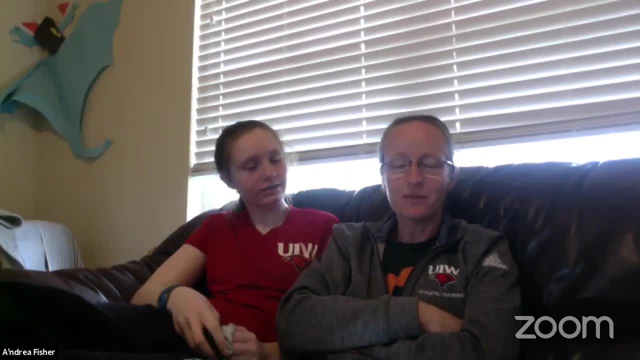 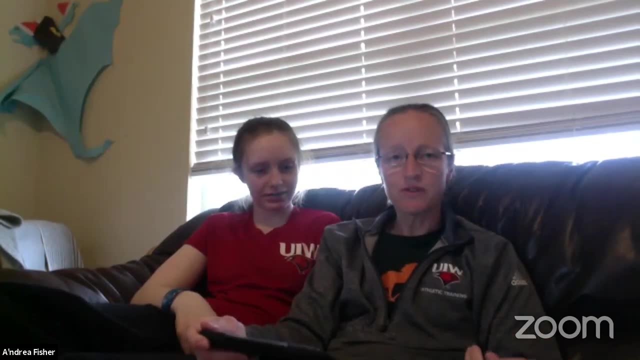 Thanks for letting us jump in. I've shared out this link with like 170 of my kiddos So they've been typing in questions this whole time as a Google Doc. One of the things we've really focused on this year in our class has been the impact. 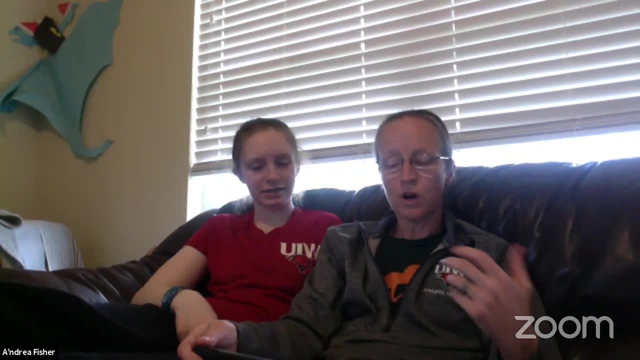 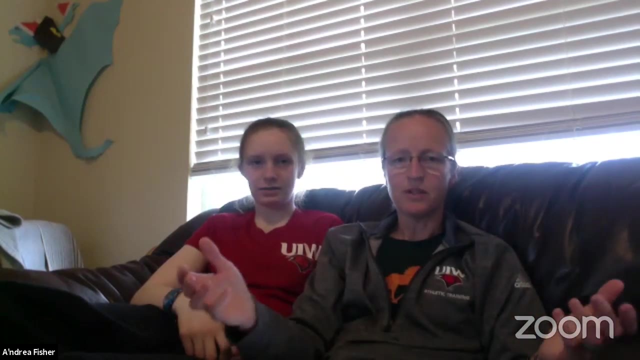 we can have on everything around us. So a lot of the questions seem to come along. What is it not just looking at just the black bears, but what are some things that we can do in our everyday lives to really impact any of the species around us, so we don't end up? 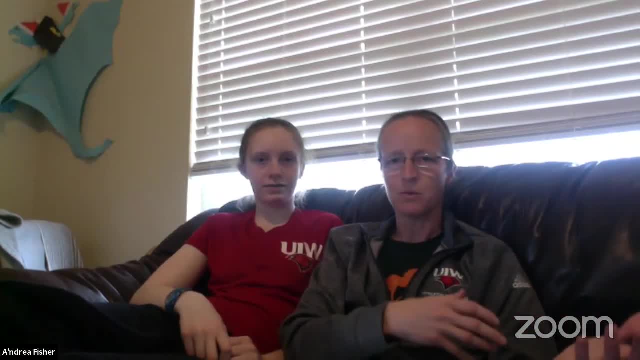 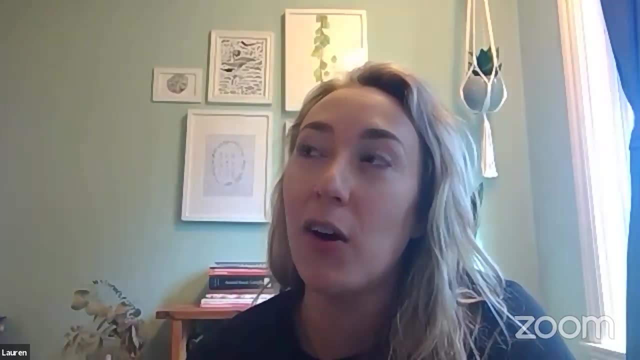 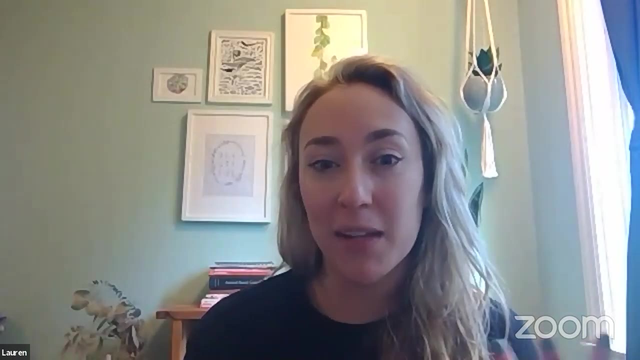 having things disappearing from the food chain and changing up their world and their ecosystem Totally? That's a really good question And the answer is a little bit complicated just because every species has really really different requirements. You know, pigeons are adapted to people's presence in a really different way than, say, 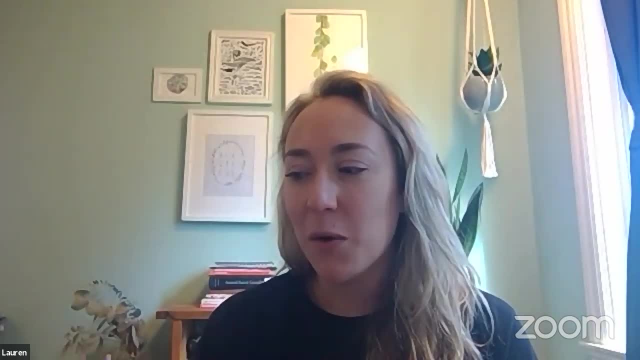 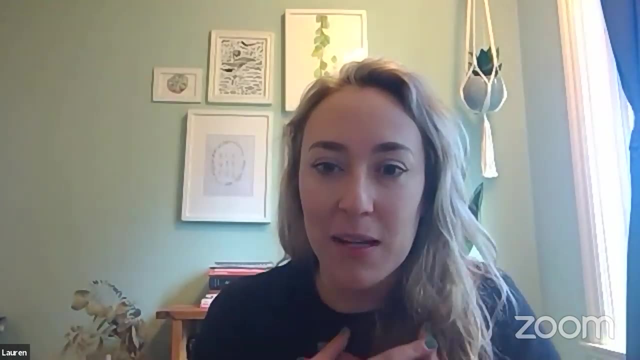 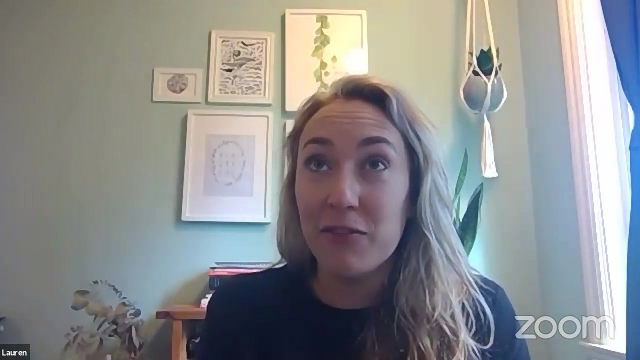 rabbits are. So I would say, You know. first, it's really important that we all just recognize how interconnected we are, that everything we do impacts the wildlife around us, whether we're thinking about it or not. And what I would recommend everyone do. the first step is just to start observing a little. 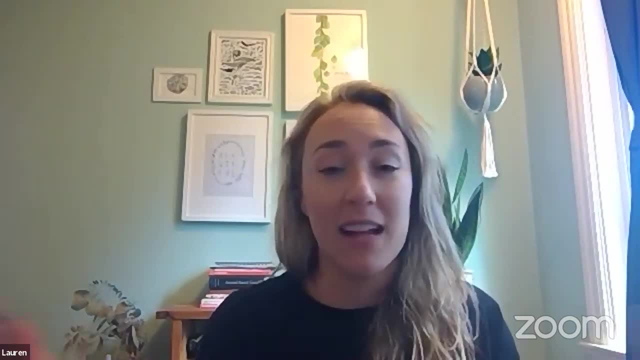 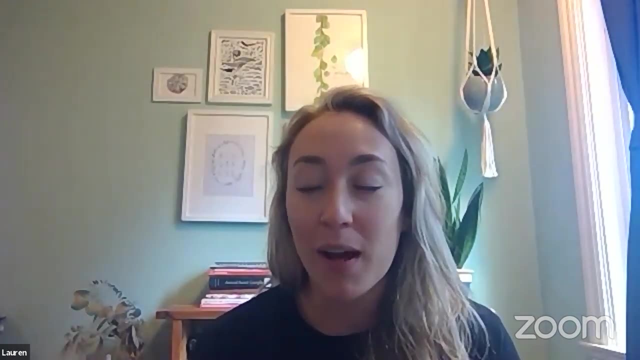 bit more than we normally do. Just start really- especially now that so many of us are at home- spend a little bit more time than usual actually looking around your home. What animals are coming into your yard regularly? Which ones should be, but aren't? 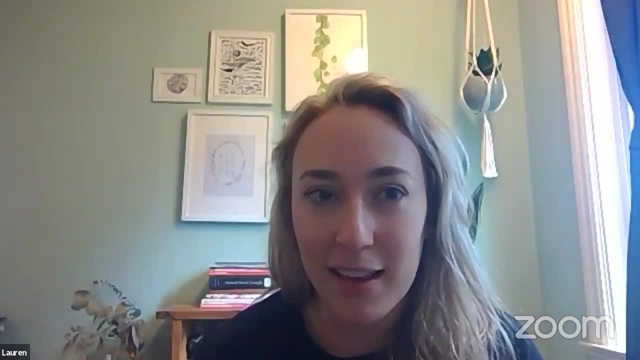 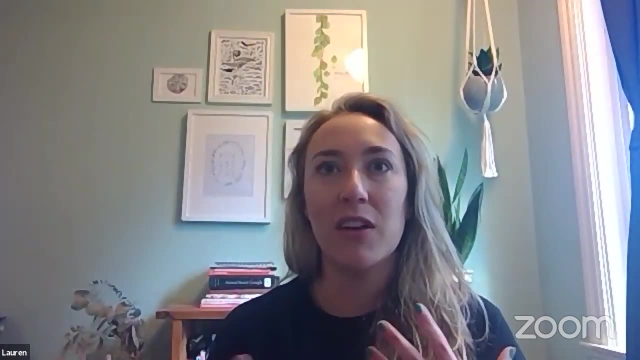 What can you find to read about the species of squirrel that lives where you live, or the raccoon that's getting into your cat food every night? And once you start observing and reading, you can start figuring out what species live near you and what those species need. 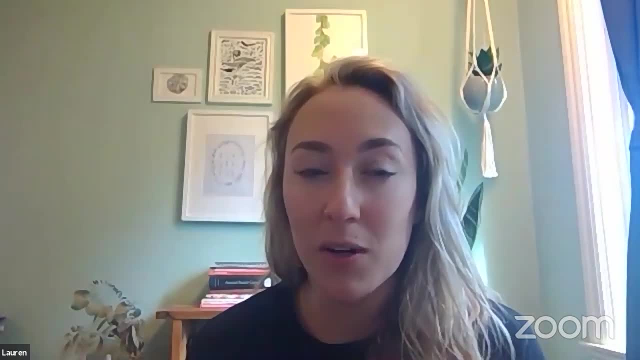 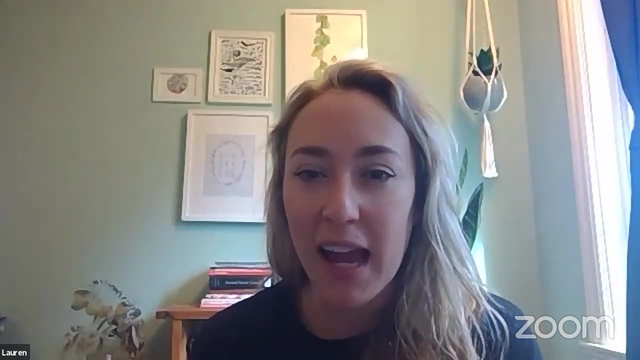 So for a lot of species it's really important that we're good stewards, good caretakers of our backyard. So that might mean, if we have a yard, doing things like taking out invasive plants, plants that come in and aren't native to the area you're from and can choke out other plants. 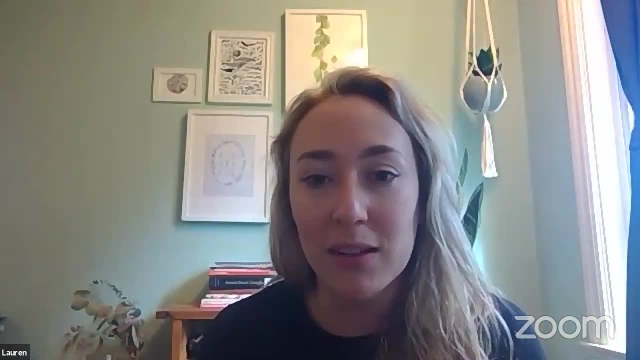 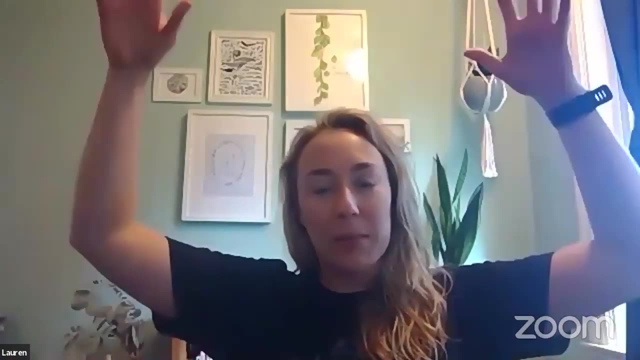 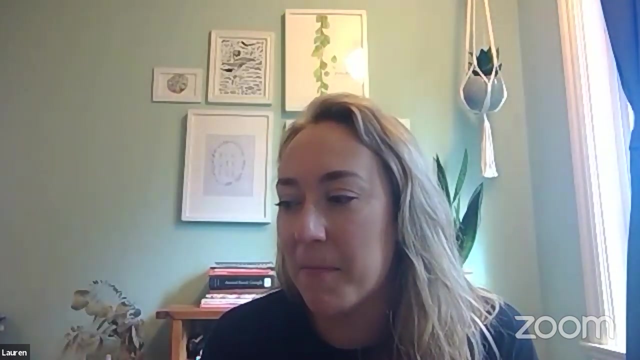 that things like rabbits or squirrels or raccoons need. It can mean making sure we stay out of conflict with some animals. So if we have gardens, putting up really big fences so we don't have to worry about deers getting into our plants and then putting us into a state of conflict. 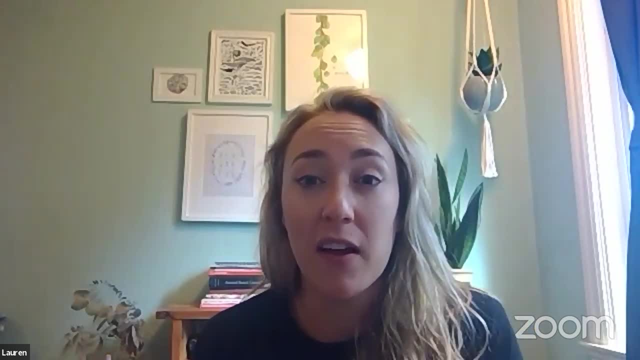 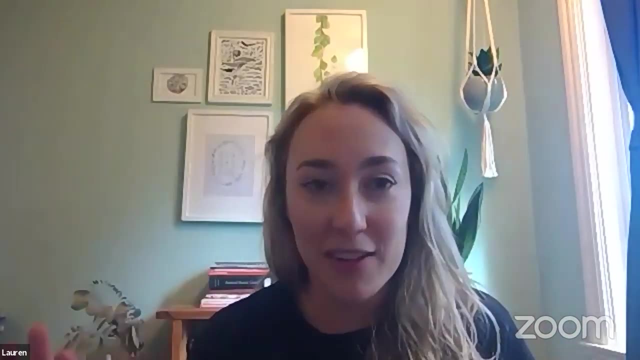 Yeah, so it really depends on the species that live around you, But there are a lot of day-to-day opportunities to observe those species more and then take care of them. Mostly, taking care of them means not feeding them and making sure you're not creating reliance. on what's in your backyard and making sure you're staying out of conflict with them, but also making sure that the wild things they rely on have a chance to thrive in your yard. Starting a bee or butterfly garden is a really awesome thing to do to help out native wildlife. 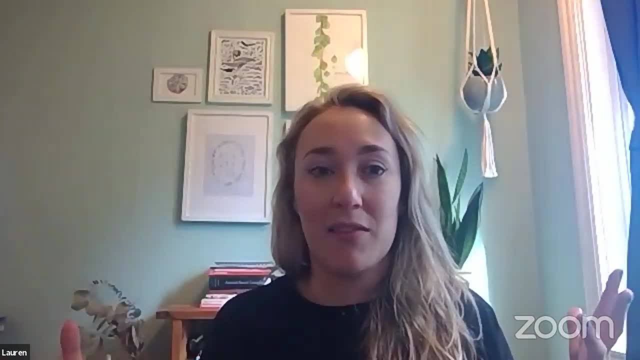 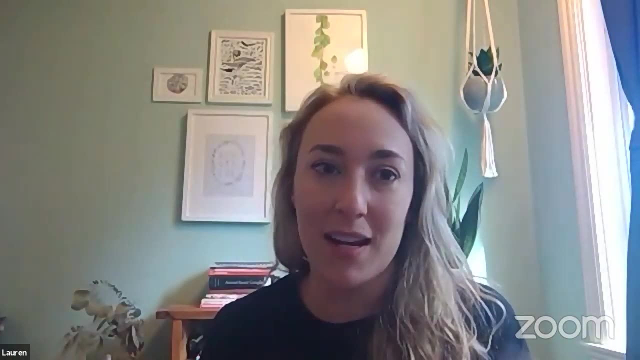 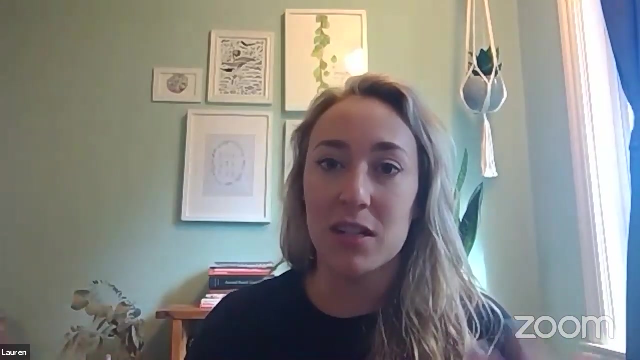 And then also think about sort of the bigger decisions we make every day, recognizing that we're all globally connected, right? So where do our clothes come from? Are we buying things we need? How much are we throwing into the garbage? What can we not use instead of throwing away as plastic that ends up in the ocean? that? 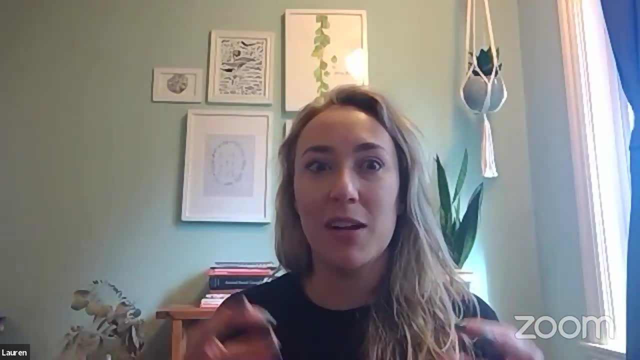 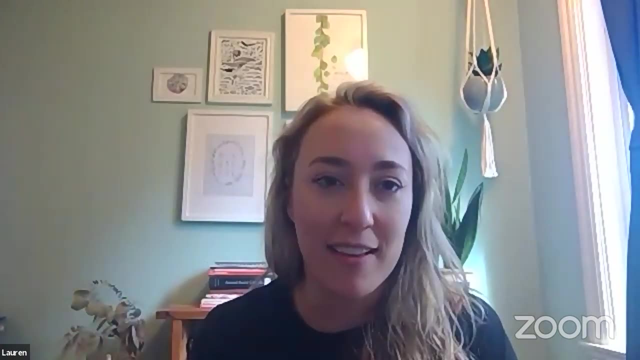 impacts wildlife. So I think there's a lot of stuff we can do in our backyards, And we also just really need to think about our actions every day. Let's reduce our waste, Let's drive less, Let's fly less, Let's use less plastic. 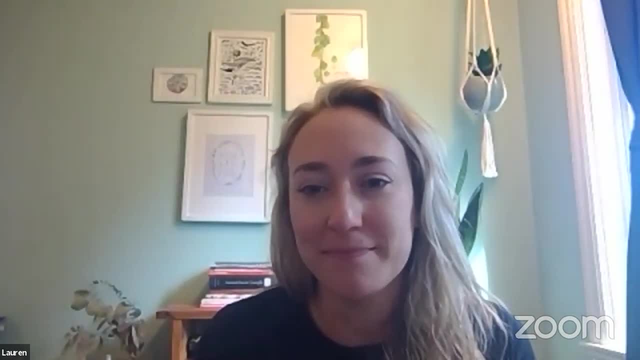 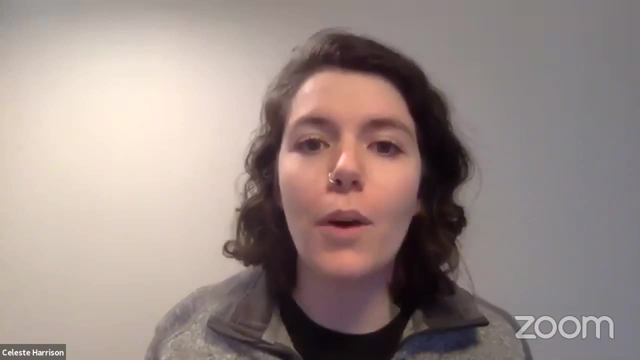 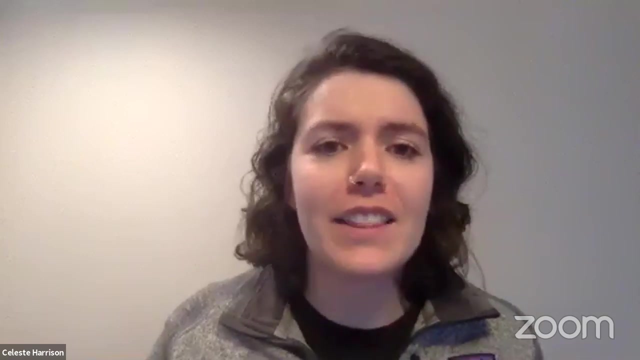 There's a lot we can do as individuals, and that feels really good. We've got a really thoughtful question. It's from a YouTube viewer named Christina Cook, who also lives along a coastline and is wondering if there's anything special she should be doing for wildlife conservation. 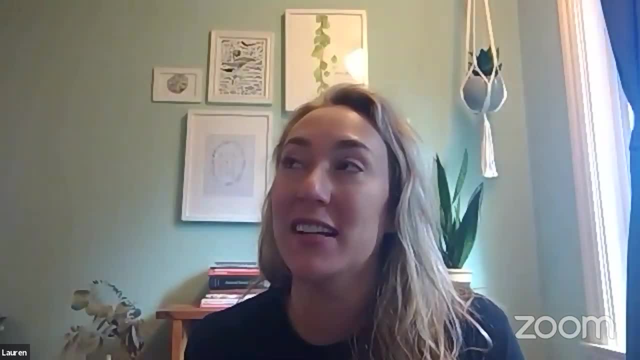 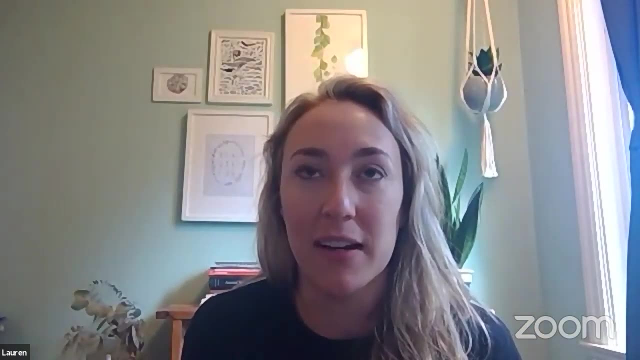 around her beaches? That's a really, really good question. I'm not a marine biologist, but we do have to have special considerations when we live in coastal areas. But a lot of those considerations are similar to what folks should be thinking about on. 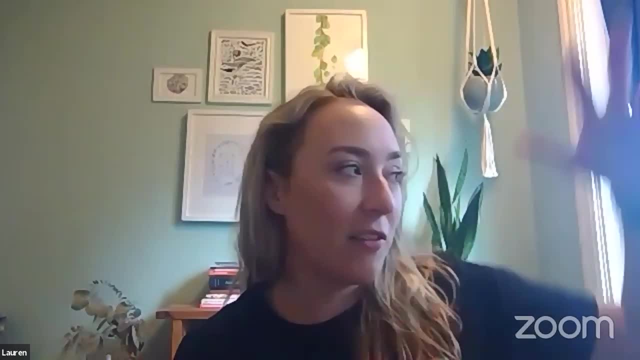 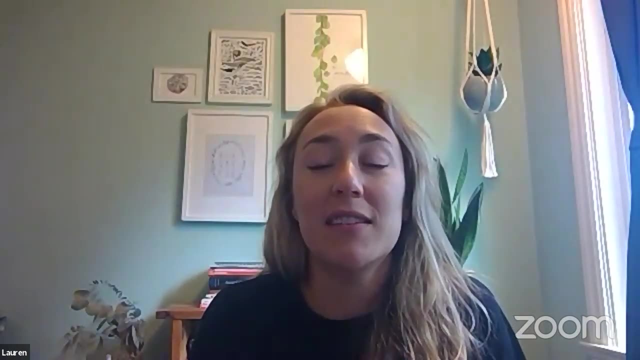 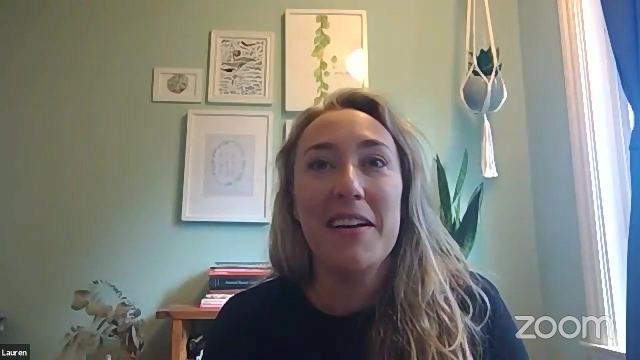 a global scale. You know, I live near a beach. All of our drains on the streets go directly to the ocean, And so there's really good reason to be extra careful about what pollution happens in a city like Victoria. You know, I'm kind of hilarious about making sure we don't use any plastic we don't need. 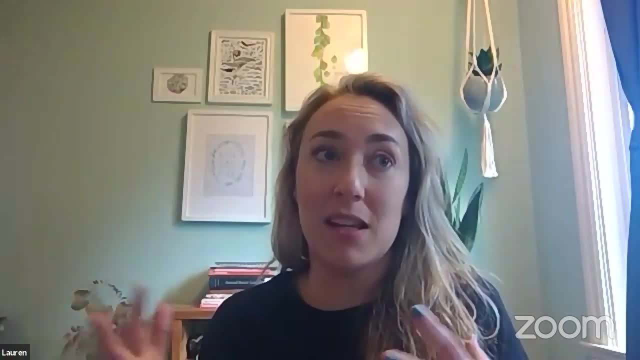 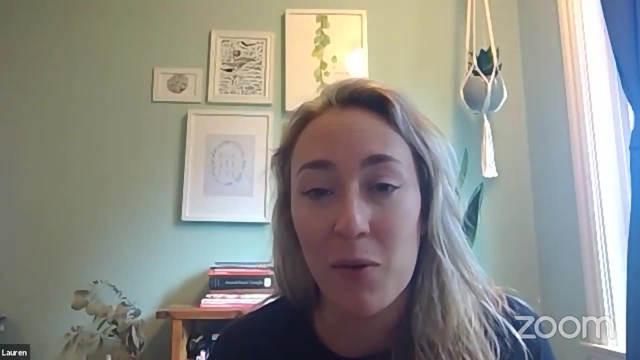 at our home. Now that plastic may end up in the ocean here and it may end up in an ocean far away, But we also have a lot of other species. A lot of other species that the other folks don't have in our backyard. 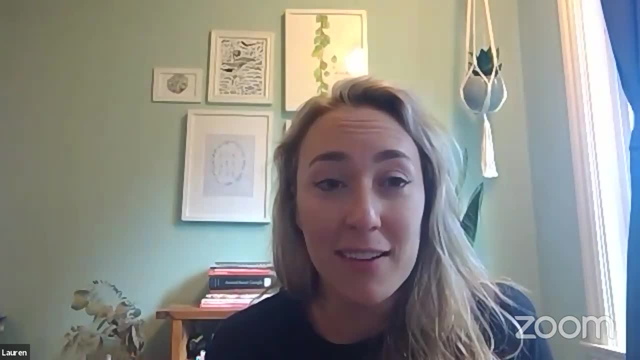 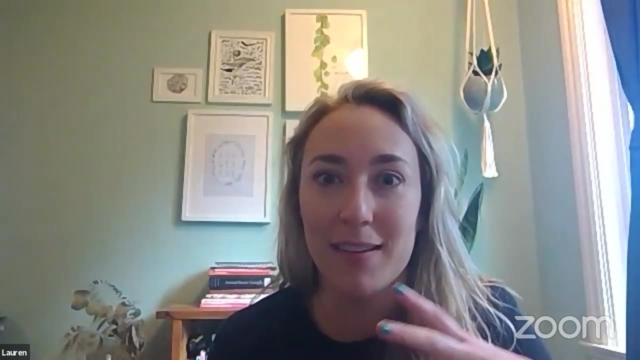 And those can be things as common as gulls, seagulls or, you know, we may have the opportunity to see whales in our backyard. So some of us have to make a decision about when it's appropriate to be in a boat, because 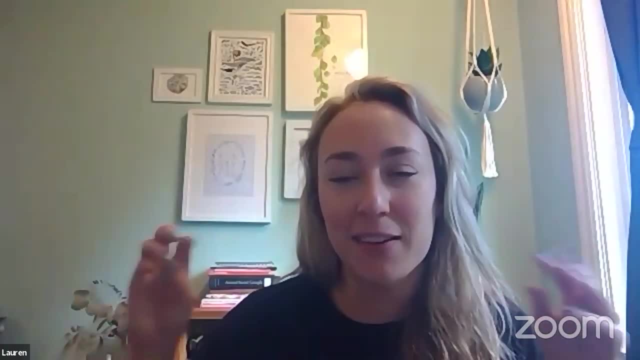 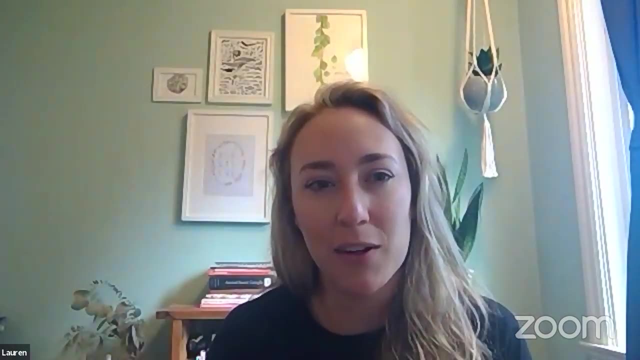 the sound of that boat can affect things like killer whales who use echolocation to talk to each other. So I would say similar advice to folks who live on the coast: Really observe what's near you and learn about those species and what they need from you. 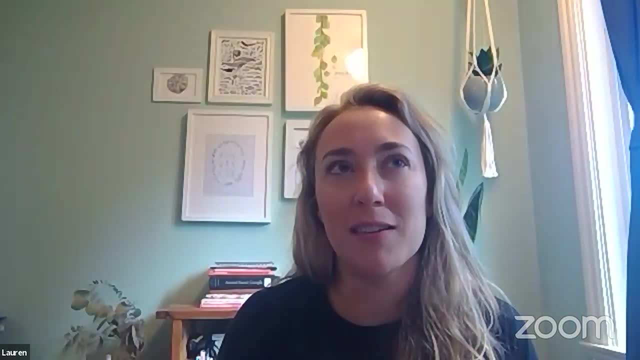 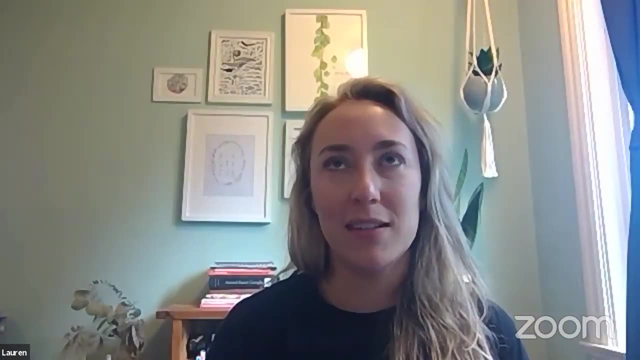 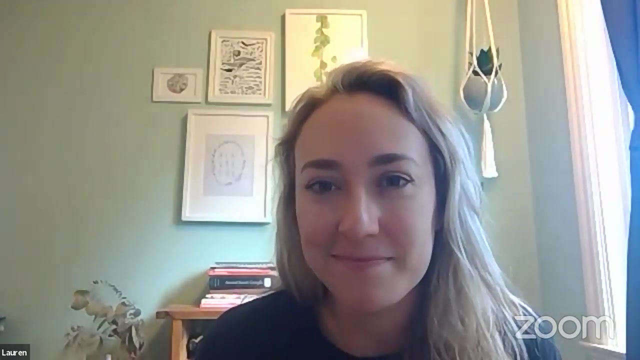 But it's a good reminder how connected we are to that giant, massive body of water that connects us to everywhere else on earth, And to really double down on being careful about things like pollution and consumption and waste. Yeah, Let's take a question from Lily and Isla. 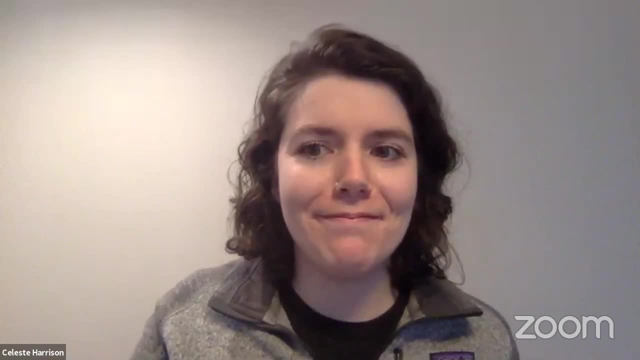 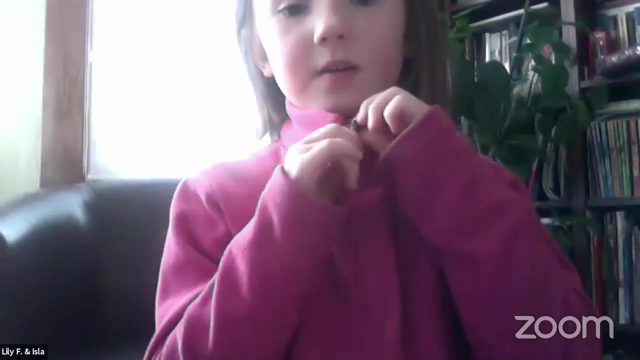 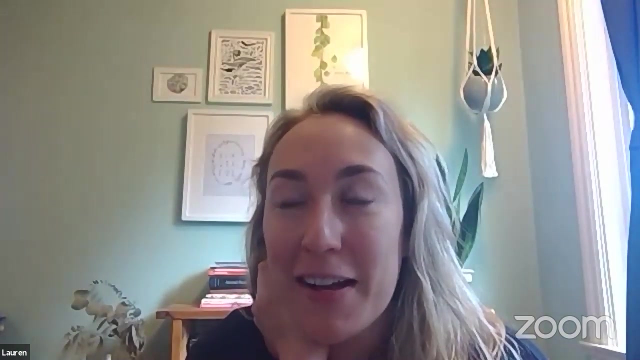 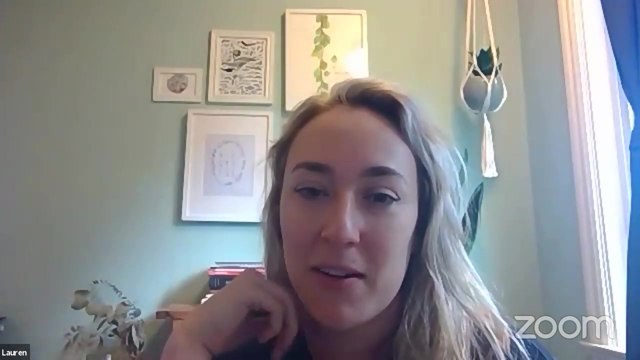 Your microphone's on. What's the what's the question? What's the favorite part of your job, My favorite part of my job? I have so many favorites and- and I'm glad you asked, because I talked about what's challenging about my job- and the favorite things I have about my job far outweigh what's challenging. 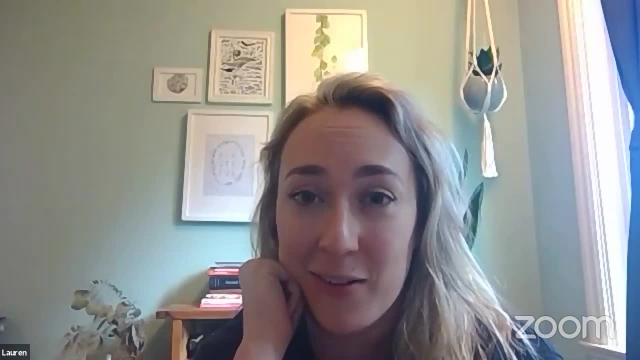 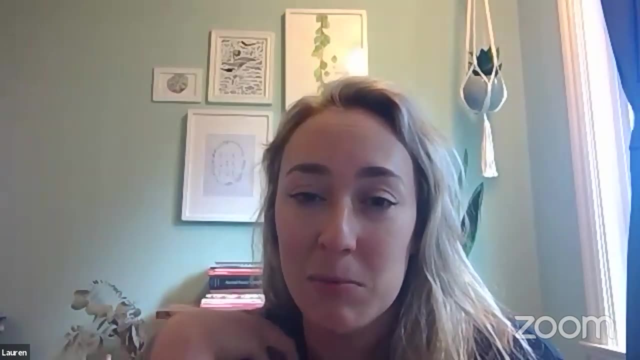 about it. So one of my favorite things is doing what I'm doing right now. It's being able to talk to people like you guys about why I love science, what I do, what I do and what we can all do to make the world a more wonderful place for people. 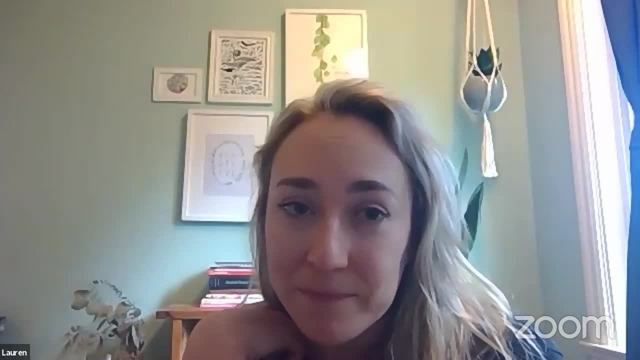 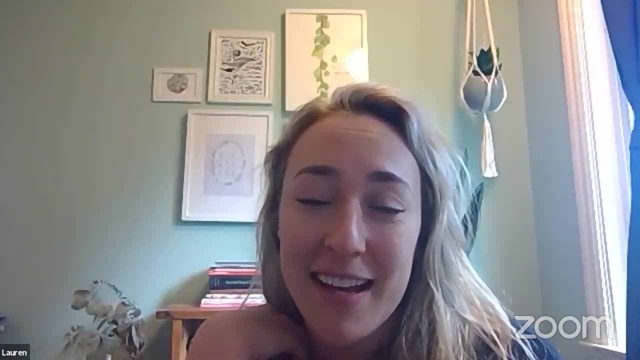 but also for wildlife. When I was a little girl, I would watch documentaries on Animal Planet every chance I got, And I wish I would have heard more from scientists, especially women, about, about their jobs and what it's like to be a scientist. 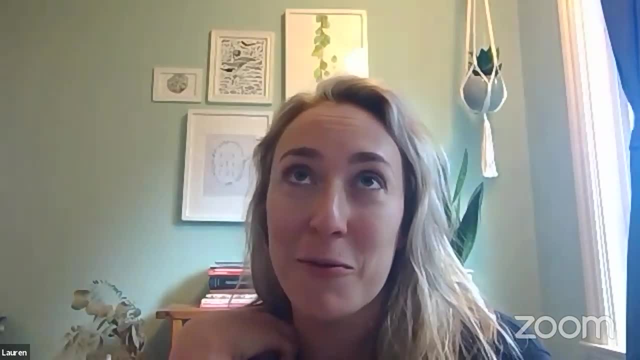 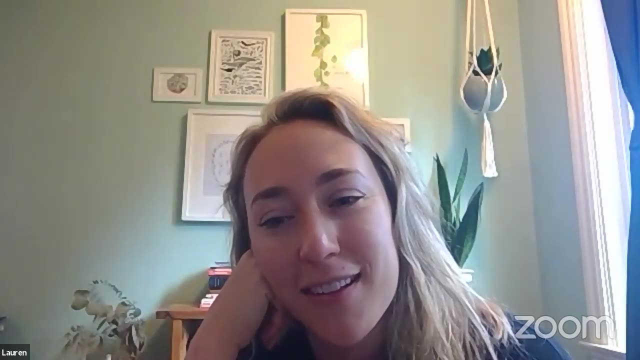 Cause I think many of us don't really know. I mean, I didn't know what scientists did until I started my career. So I love talking with people about my science and I love connecting with people on the internet about science. I also love spending time outside. 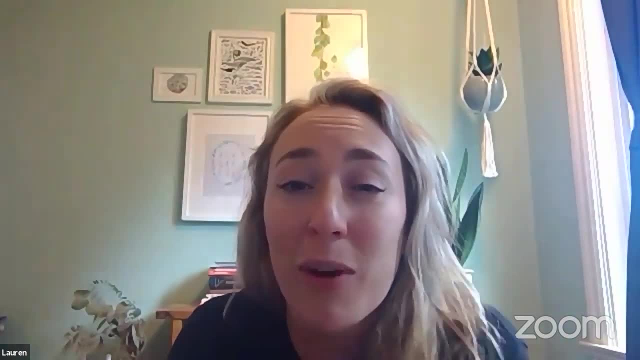 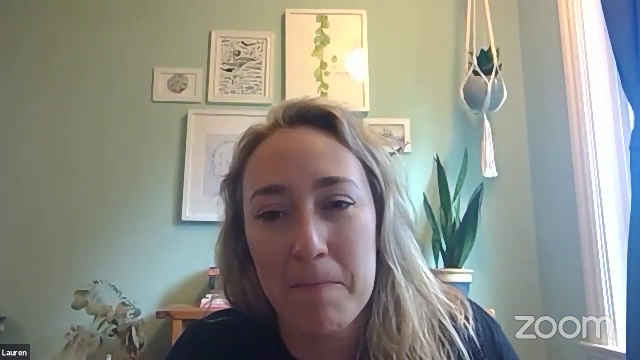 I love learning about animals. I love learning about animals That I care about. I love working with young people who are like doing incredible things out in the world to make the world a better place. So those are all really really cool parts about my job. 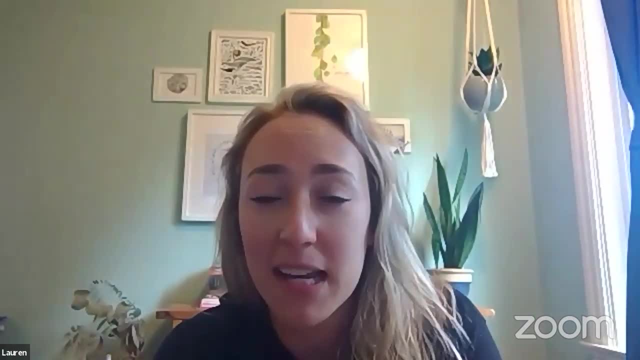 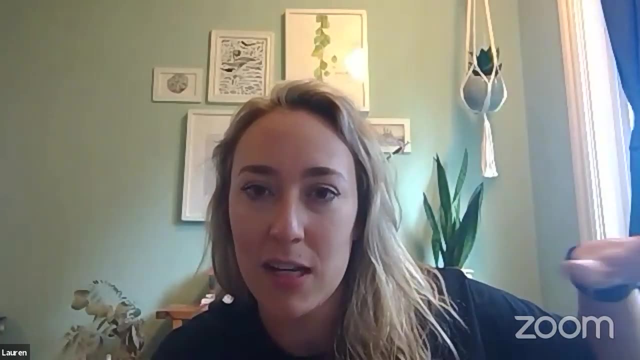 The other thing I'll say is Celeste mentioned at the beginning when she was talking about the work I do that some of my work in the past I've got to partner with Coastal First Nations, So those are the Native American indigenous peoples that live up far up on the coast. 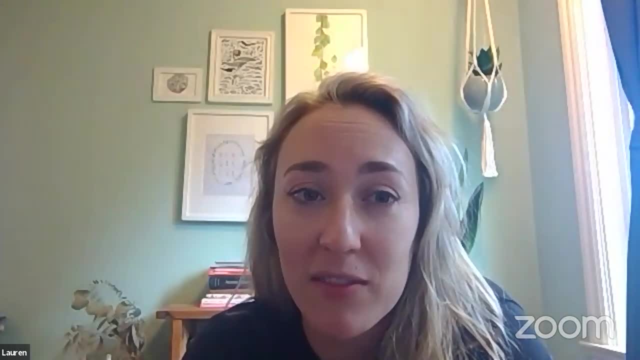 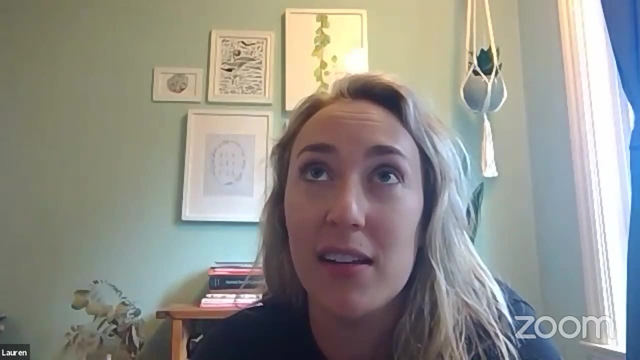 sort of in an isolated region of British Columbia, Canada, And they lead a lot of really awesome wildlife conservation projects And I just feel really lucky to be able to work for and with those people. You get to meet a lot of really cool people when you're studying animals, as it turns out. 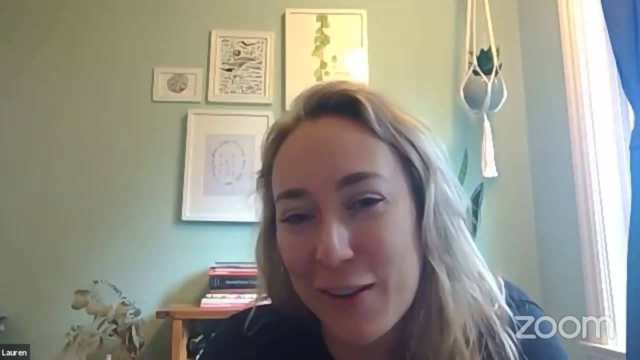 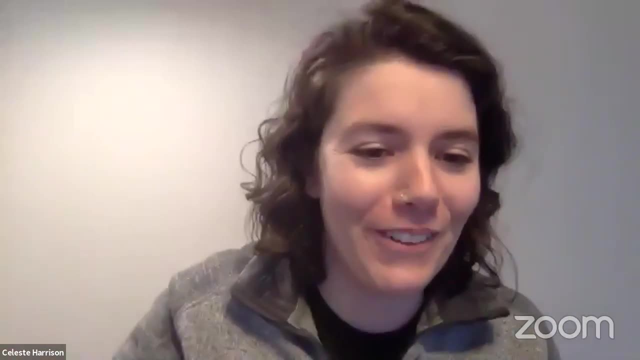 So that's my favorite part of my job. I think That was a lot of answers, but We'll take them all. We love them. There's a lot of questions online, So if you keep answering, we'll keep hitting more questions. 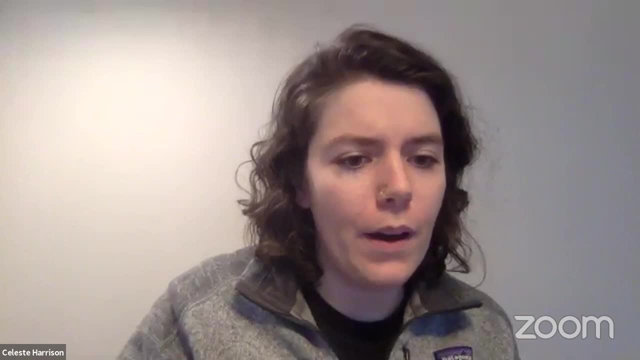 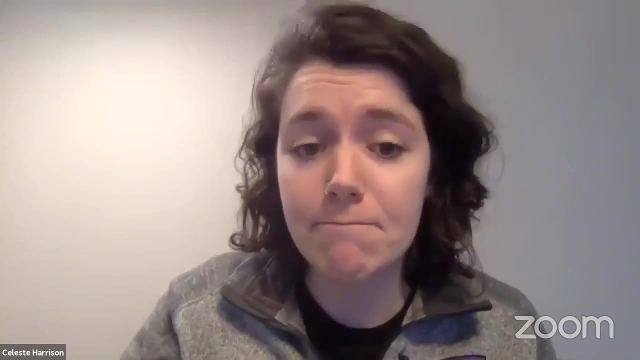 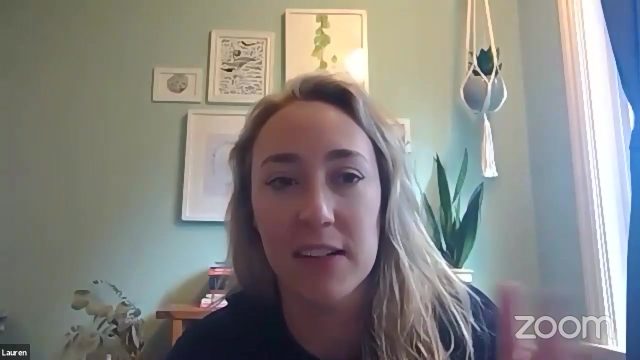 A couple of questions that keep coming up are: is there a main place that you go out into the field to work And is there a main place that you study? Yeah, Okay, So all of my research during my graduate school during the last sort of six years? 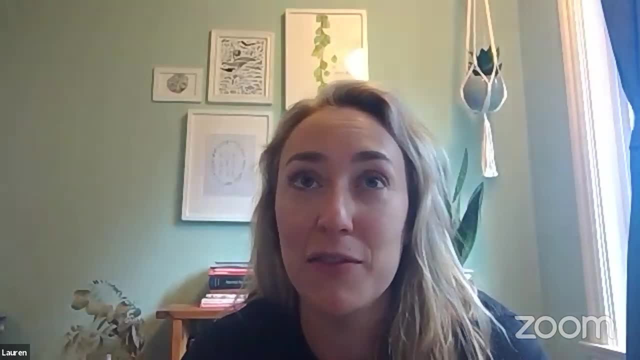 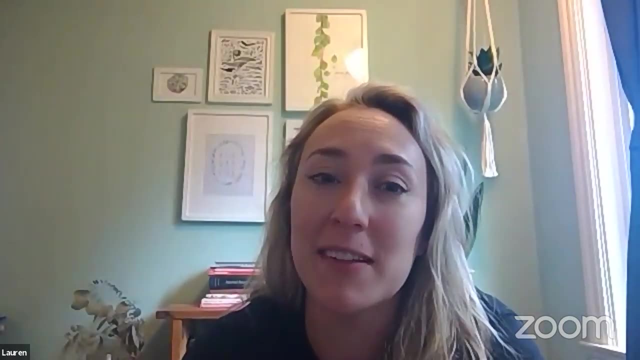 has been in British Columbia, in Canada, Actually, for my research project a while ago I studied fish called rockfish. That's a whole other story, but that was in the ocean off the coast of British Columbia And now all of my work is in British Columbia. 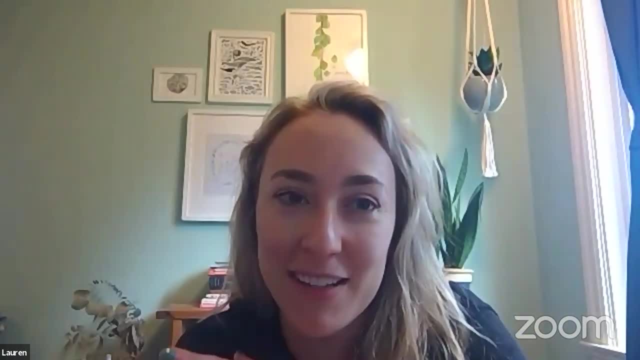 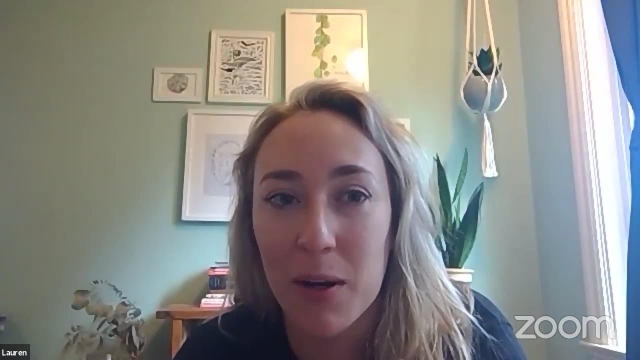 And my field work, which I was supposed to be leaving for in two weeks, which I've postponed for now, so I can stay at home and keep myself and the community I work with safe. yeah, was supposed to be in that picture that I showed you at the beginning with the river. 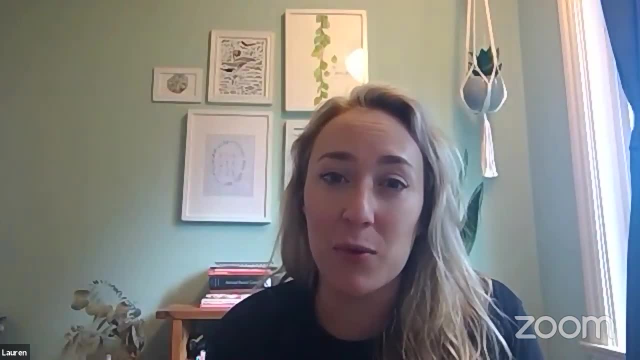 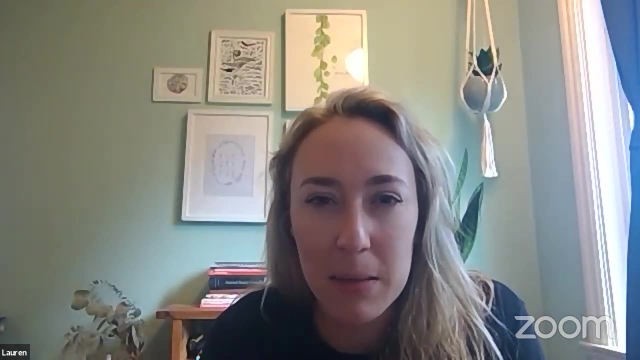 and the mountains on the Sunshine Coast of British Columbia, in a city called Powell River, And it's a city of about 20,000 people, So not a particularly small town, But you have to take a ferry to get there, So it's kind of isolated. 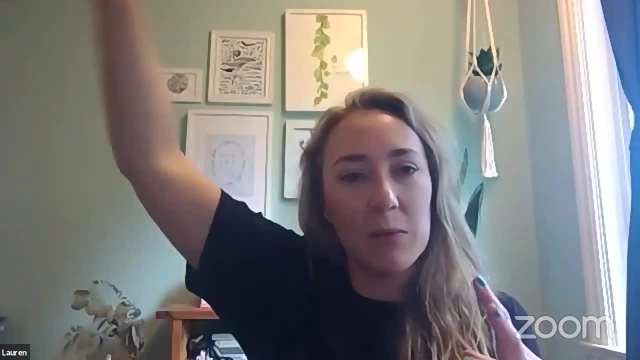 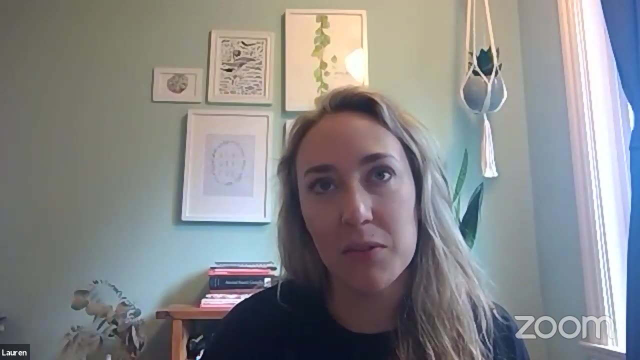 And they're right near a bunch of coastal mountains where a lot of wildlife lives, So they have a lot of problems with black bears coming into town, as well as with other wildlife. So that is where my field work is going to happen, But all of my work is pretty local. 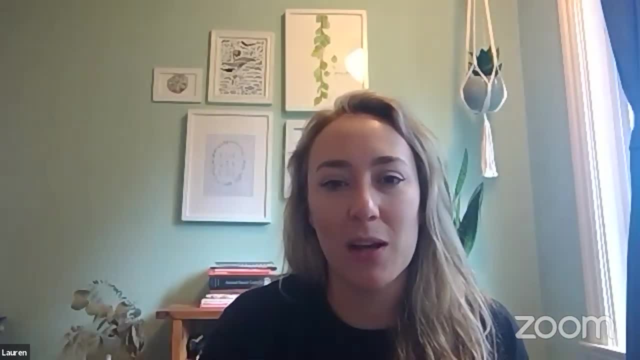 Some people travel a lot for their research and that's really cool, But I feel really lucky to be able to, from where I live now, to get to the field site that I will eventually go to when it's safe to do so. 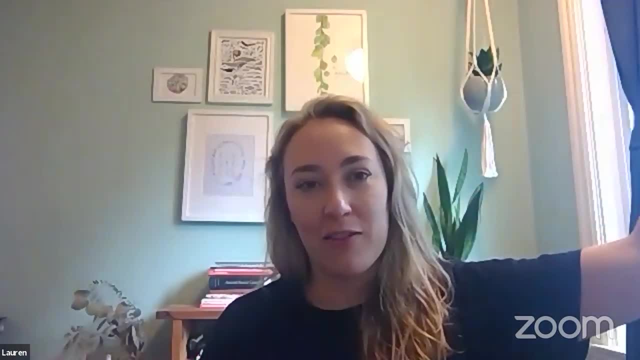 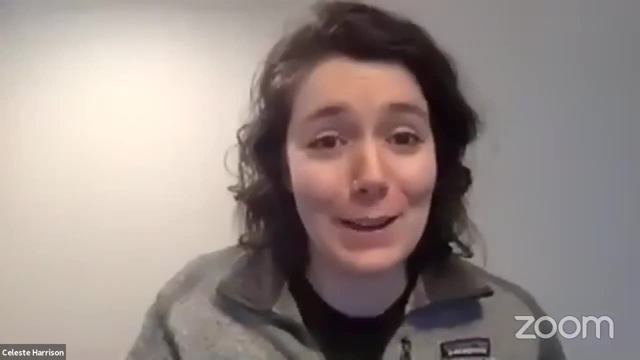 It would just be a four-hour drive and then an hour and a half on a big ferry And then I would be there. I love how that's your definition of local. For me that sounds like to each their own. Let's head to the house for our next question. 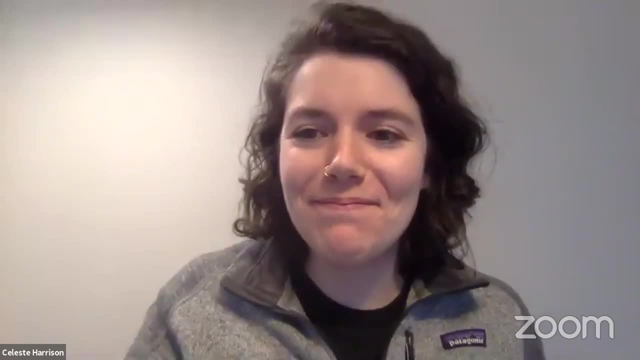 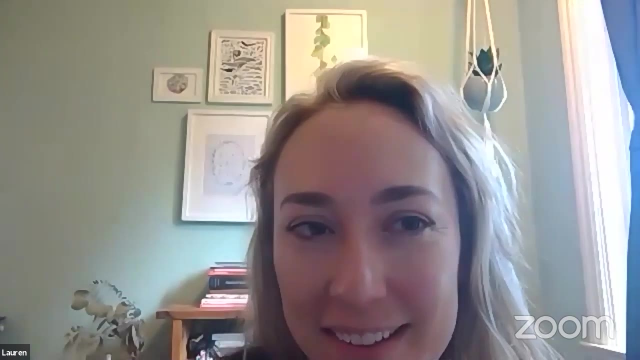 Lily, your microphone is on. Have you ever been a Daisy Scout? A Daisy Scout, Lily, can you tell me what a Daisy Scout is? My answer is no, but I don't know what it is. It's like a Girl Scout. 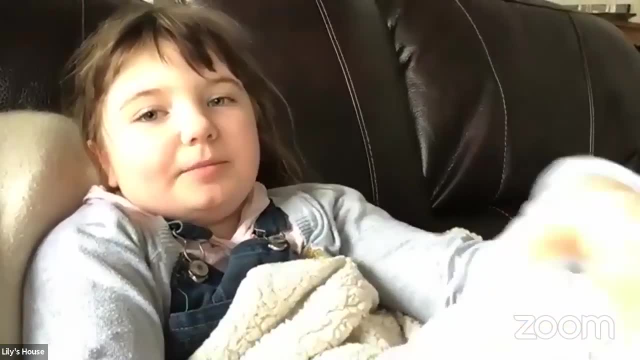 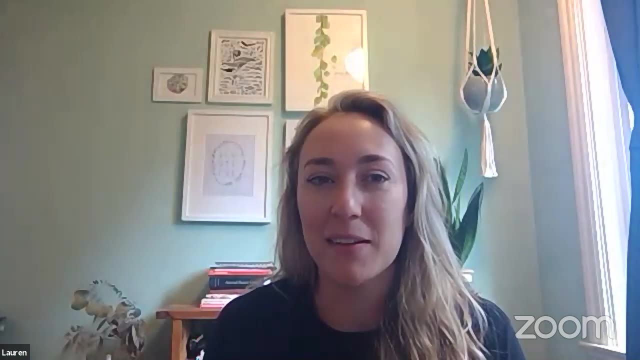 Okay, You do all 10 steps and go outside and learn about more nature. Oh my gosh, I wish I had been a Daisy Scout. No, I was not a Daisy Scout, but it sounds incredible and like something I would do now if I could. 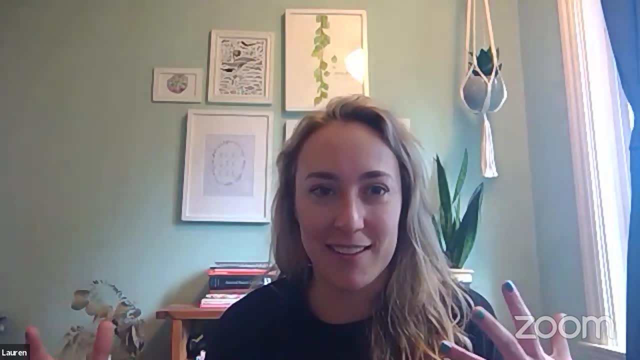 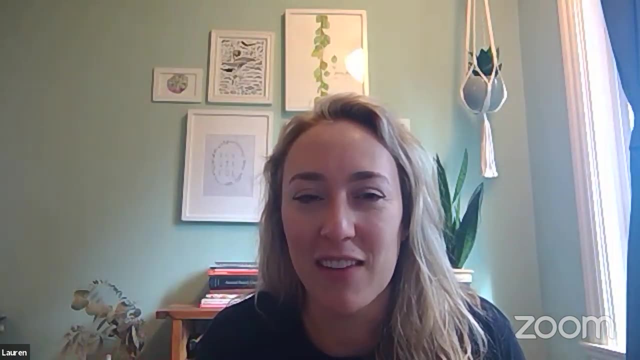 It sounds really important to helping build the skills you need to be a good scientist or anyone who works outside. I was in 4-H so that was kind of as close as I came to any of that stuff. I didn't learn a ton of outdoor stuff in 4-H, but I had horses. 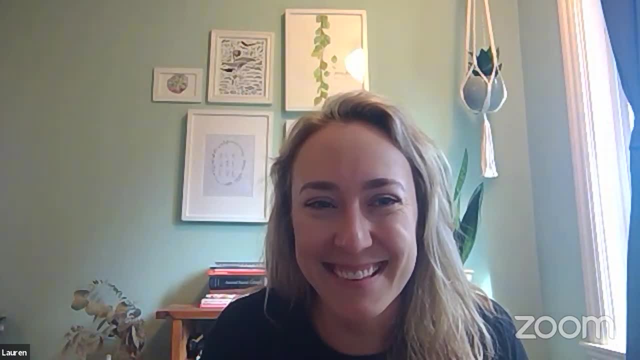 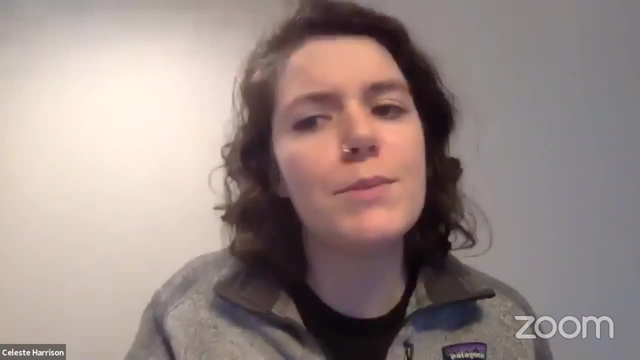 So I really liked it. Let's take our next question from Kristen Larson, Your microphone. I'm having some difficulty with your microphone but, Kristen, maybe you can help me out. Once your mic is on, you can ask a question. nice and loud for us. 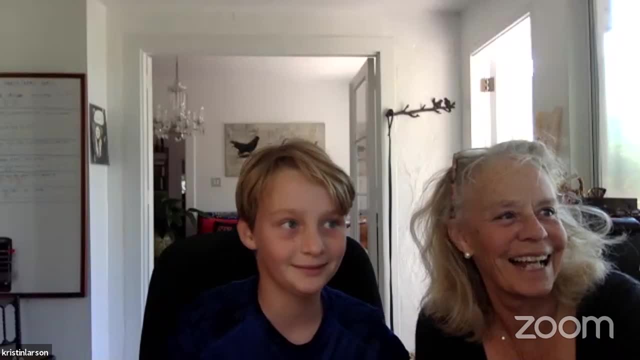 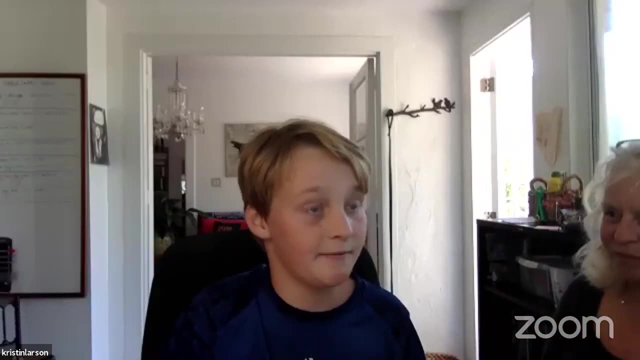 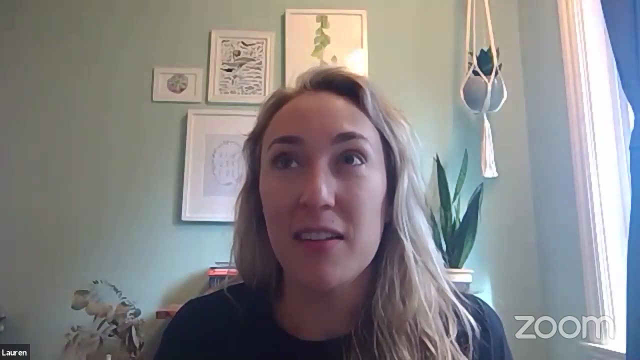 Is it on? We don't know. Is it on? Yeah, This is Gus. actually, He's our student here today. Yeah, Do you believe that saving animals can save us in the long run? I think definitely, and I think that's a really good question for so many reasons. 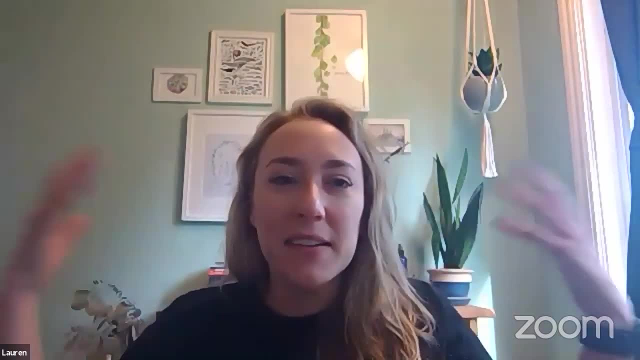 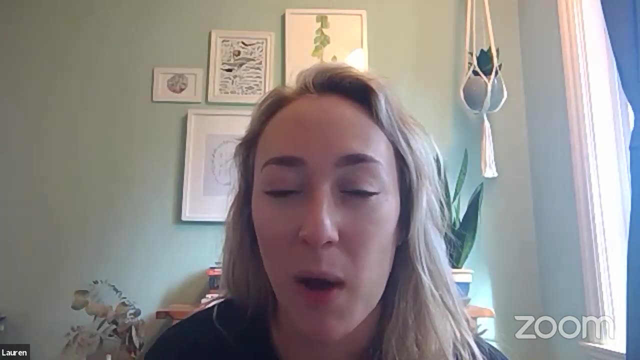 I mean one, I think. because we have so much technology and so many of us live sort of in or close to cities, I think it's really easy to forget how much we rely on wildlife. right, Wildlife provide really, really important services for all of us. 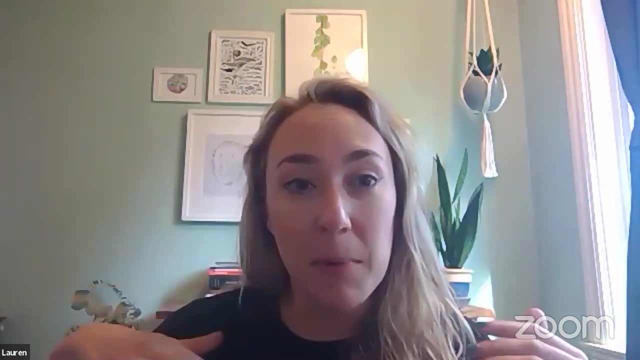 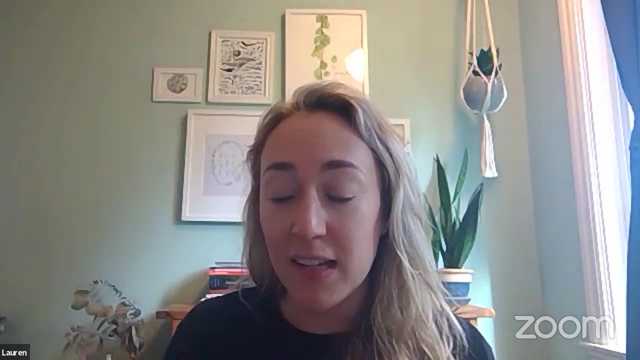 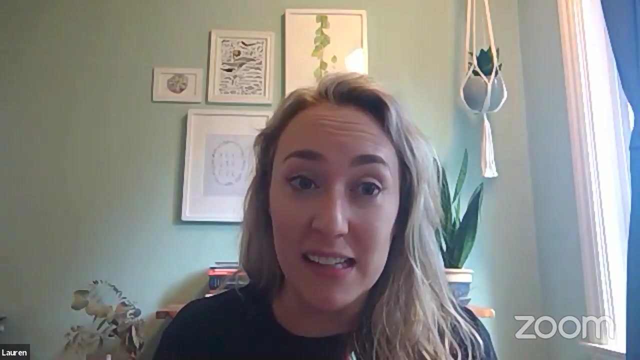 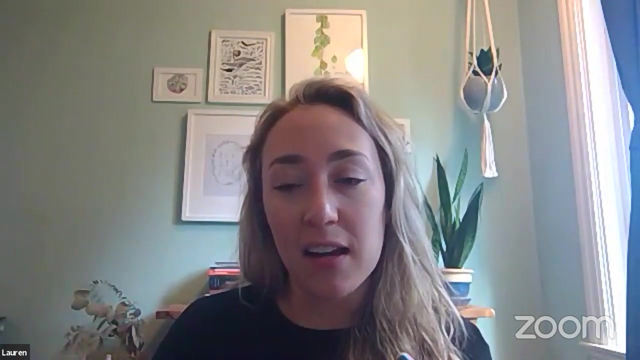 And in some places where there are predators, they control deer populations right. So things like wolves and cougars and even sometimes bears- And even sometimes bears can help with big populations of other animals. There's research that shows that if we treat animals appropriately, we can limit the spread of disease, which is a really relevant conversation that's happening right now- that it is important that we respect the space and habitat of animals. Because when we come into too close of contact with some wildlife it can transmit diseases. Also, we rely on animals, I think, for, like our animals, Our well-being in a less concrete way. You know, animals bring us a lot of joy. 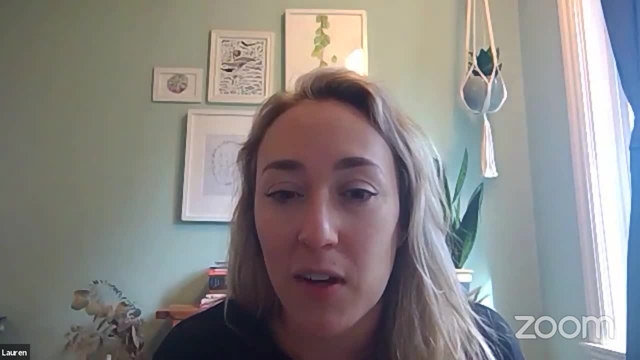 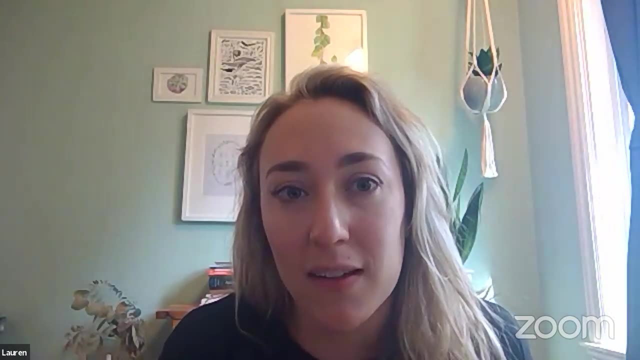 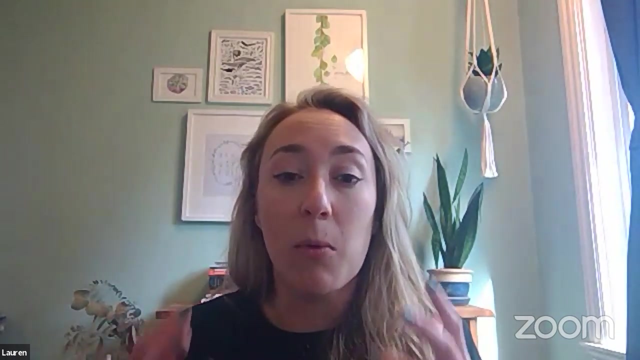 I, as a little kid, was just transfixed by how beautiful animals are, and I still am, And so I think also animals are a signal to us of the state that our world is in, Because in some ways the impacts of things like climate change or pollution are more immediate for animals that live in forests than they are for us. 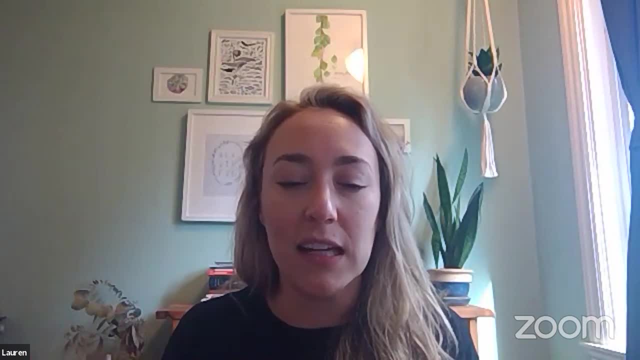 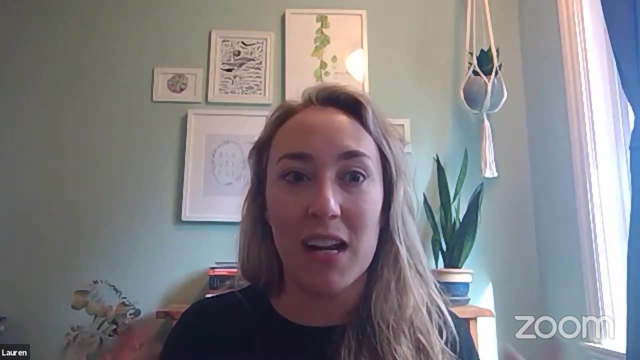 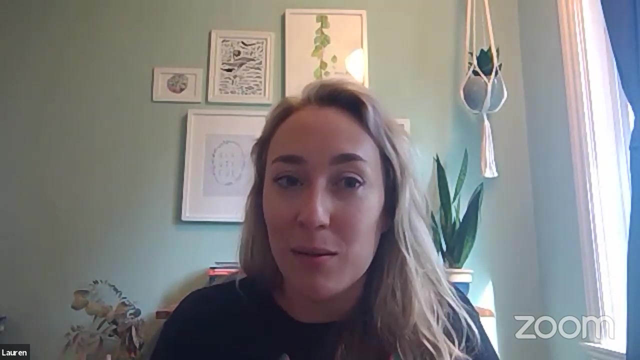 We're a little sheltered from that, even though we're connected to all of those things, And so I think a really important aspect of paying attention to the health of animals is not only that they can save us by providing us with things, providing us with joy, but also that if they're doing poorer, we will too. 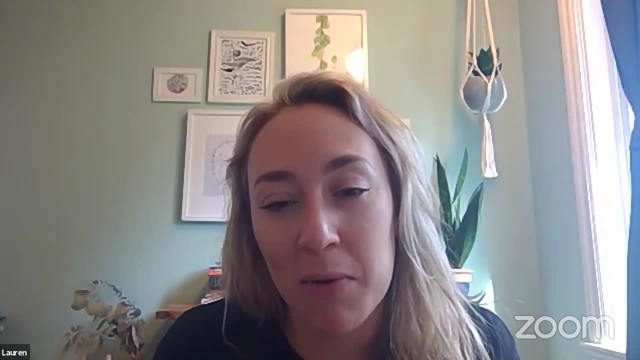 So that's a really good question, A really important one right now. That was a really good and thoughtful question. guys, I feel good about that. one Tons of people on the Internet are wondering, Lauren, if you have any questions for us. 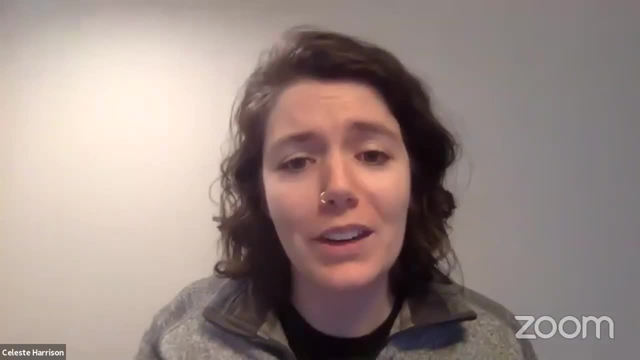 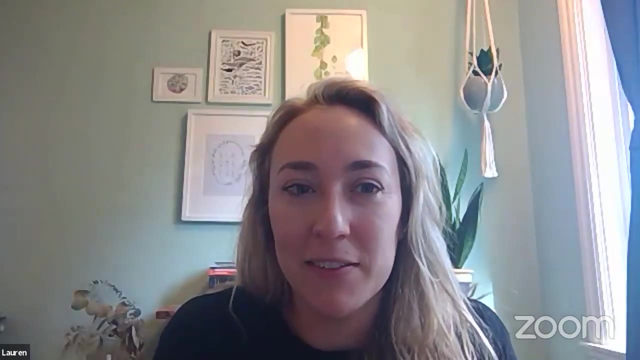 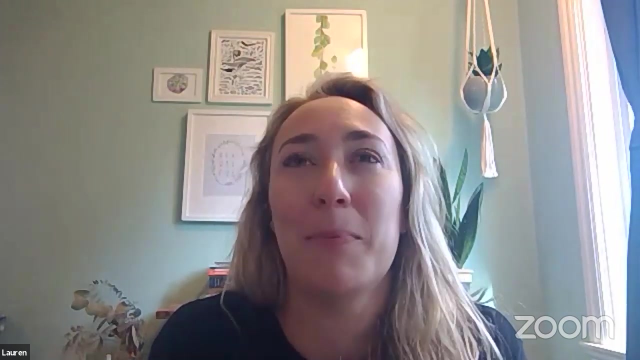 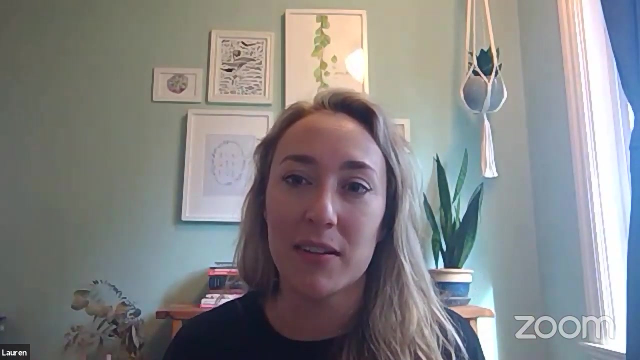 Yeah, I'm wondering, Lauren, if you have any inspirations in your work, any people that got you into this line of work or that keep you motivated now. Oh my gosh, So many people. Two National Geographic explorers that come to mind are, of course, Jane Goodall and Sylvia Earle, two women who are brave and bold and brilliant and really paved the way for me, when I was little, to have someone to look up to, who looked like me and who was doing this work. 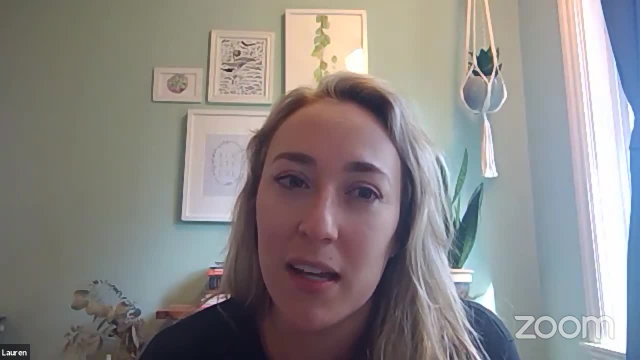 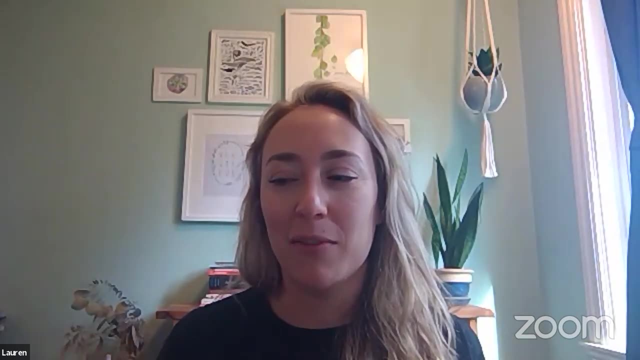 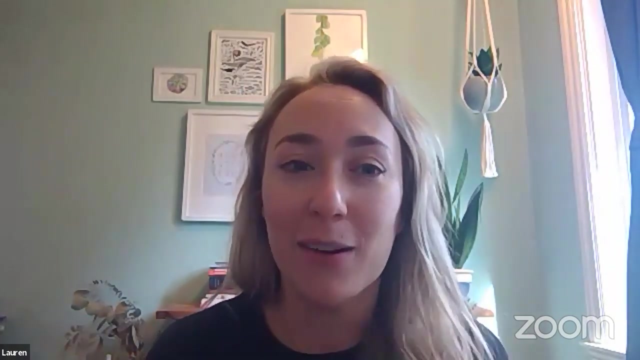 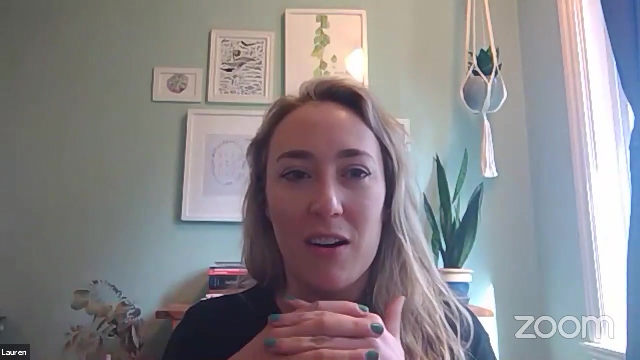 And also who. Both of those women do their work in really visible ways, really ethical, kind ways, and engage the public, And so I'm really inspired by people like that. I'm inspired by my supervisor- His name is Dr Chris Daramont- who does really incredible work in this world we live in of conservation science that thinks about people and wildlife in our inner connectivity or places in the world. 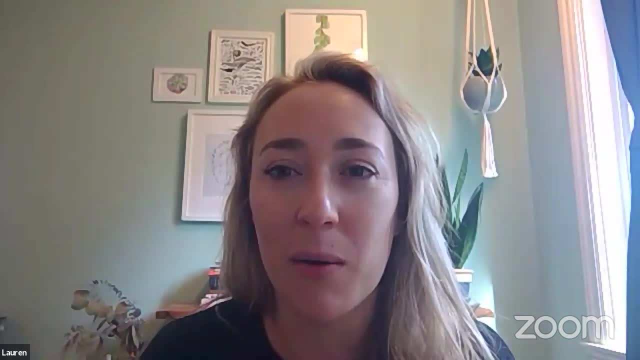 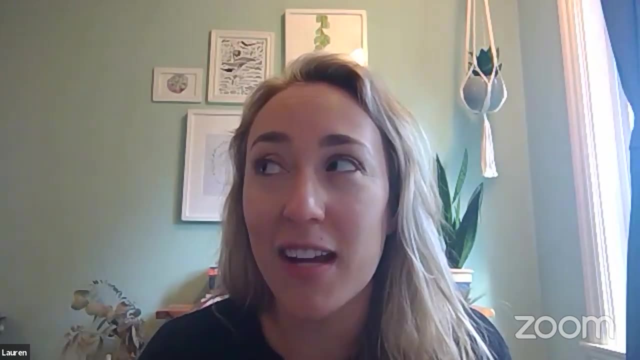 And I'm inspired by every single person that I work with. I said one of my favorite parts about my job is the people I work with, and all of them inspire me every single day. They're all working really hard to make the world a better place. 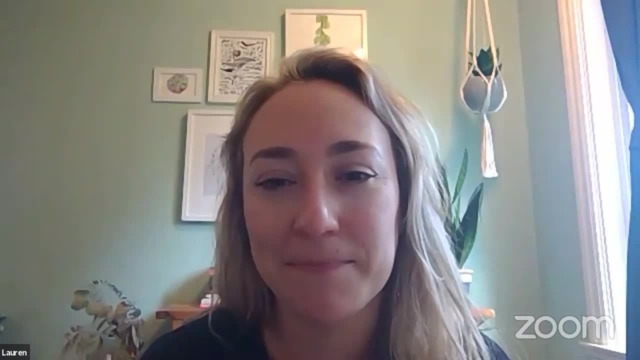 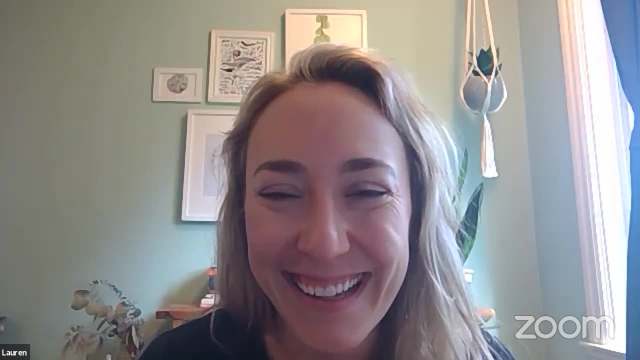 So I have endless inspirations. I'm really lucky in that way. Awesome, We've got tons of people asking kind of opposite questions: What is the coolest thing you've ever seen on the job and what is the most scared you've ever been on the job? 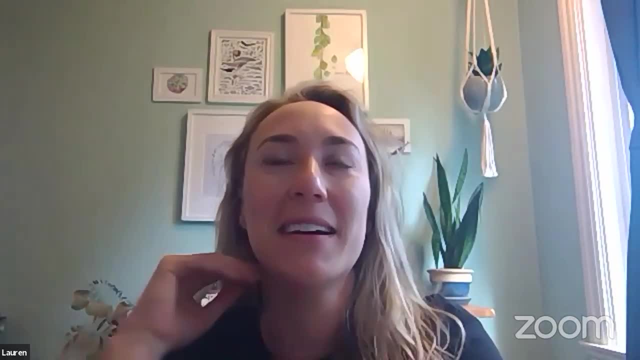 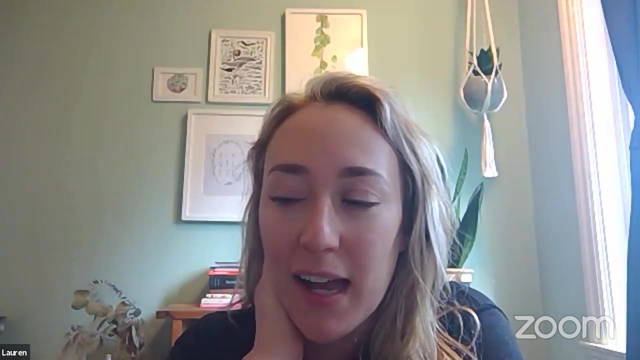 Okay, Those are both really good questions. They might not be two different answers actually. So I really am lucky to work in the places I've gotten to work and particularly lucky to work in places way up on the coast in British Columbia that are still pretty remote. 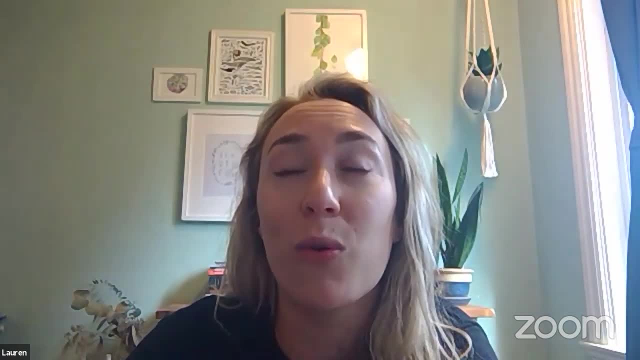 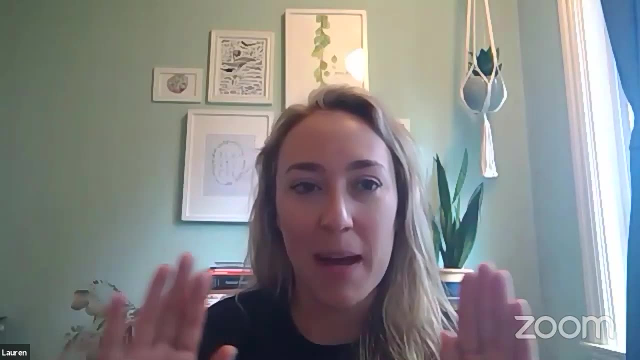 And I've seen a lot of grizzly bears, which are incredible animals, but animals that definitely deserve a lot of space and a lot of respect, And so probably the scariest thing that ever happened to me was in the field was being bluff charged. 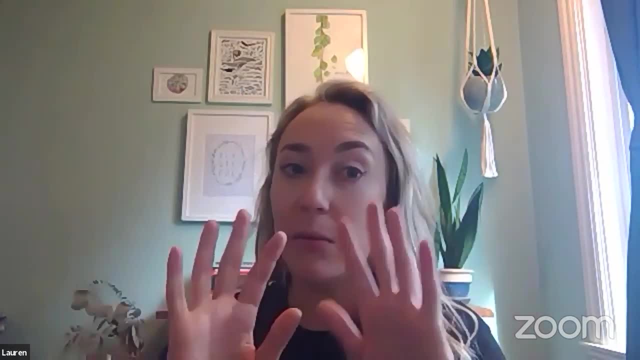 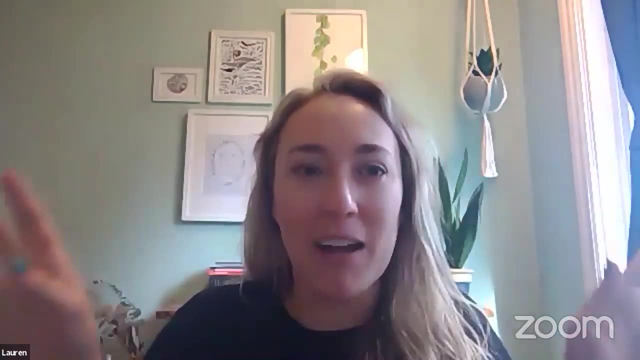 I was being bluff charged by a young male grizzly bear. He was totally behaving appropriately. We were not. We accidentally got too close. We were in like really thick forest and we popped out and there was a grizzly bear in front of us. 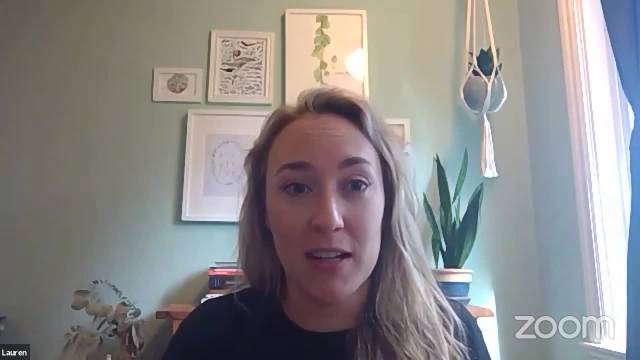 So grizzly bears do something called bluff charge, where they make a bunch of noise and start, and then he sort of started running at us And we of course, immediately we're like, oh my gosh, I'm so sorry we're here. 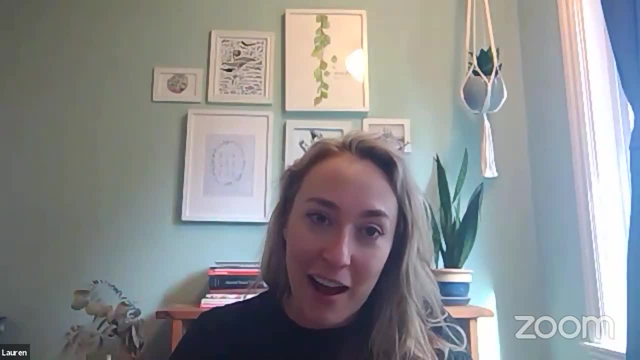 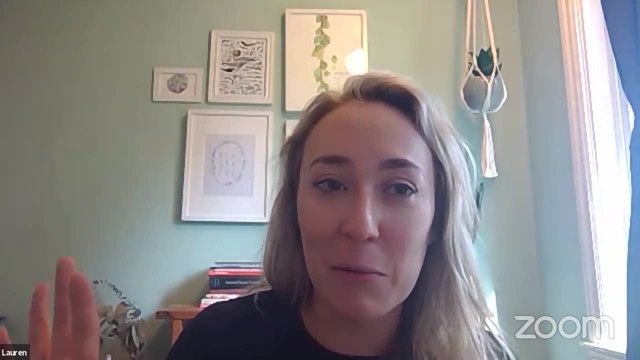 We stood our ground. We had some bear spray, But we luckily didn't have to use any of it Because we were so close And we were so close. We were close, We were close, um, because the bear said, okay, they respect me, they're afraid they know to back off, um, and he did. 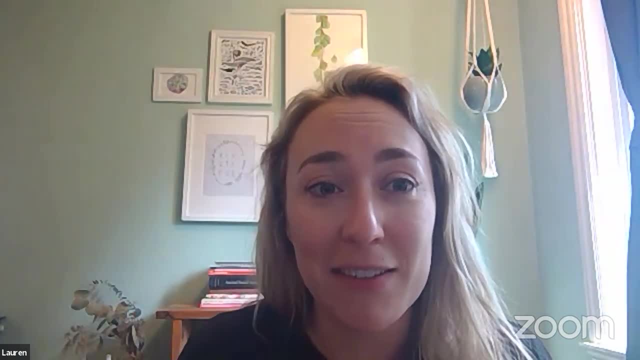 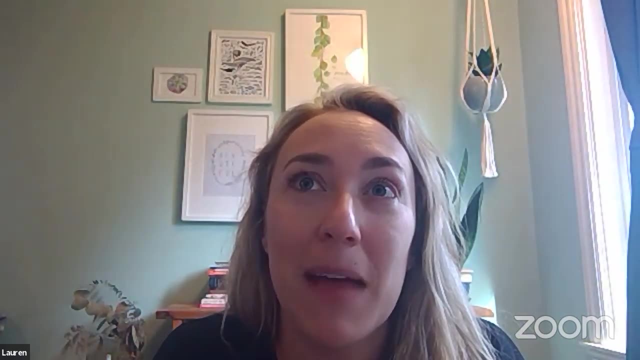 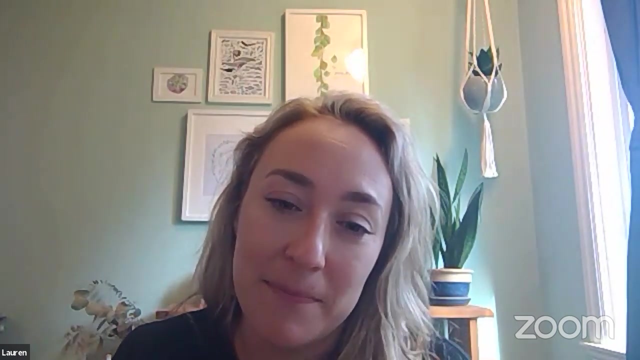 so that was really scary, though, and a good lesson to learn to make sure to respect animals at all times. um, the coolest thing i've seen in the field um happened probably about three or four years ago and i was really lucky. i was working um up in coastal first nations territories and there is 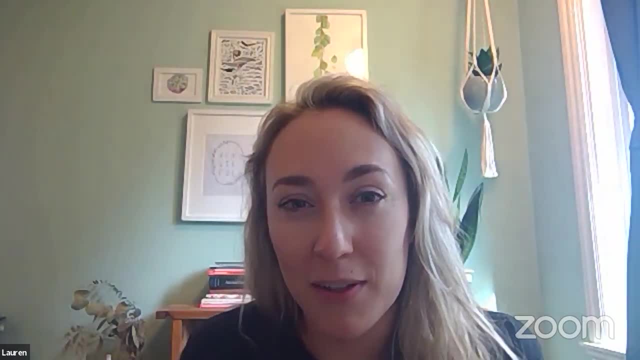 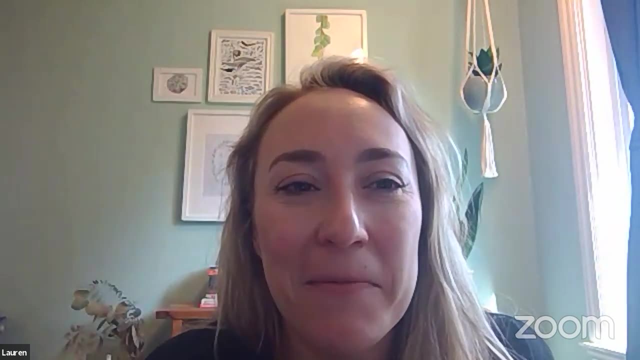 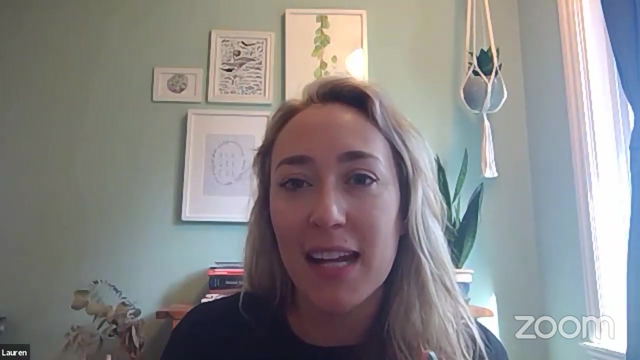 this magical thing on the coast called a spirit bear. raise your hand if anyone in the in the group has heard of it. yeah, okay, celeste has. oh, we got a couple, gus has. um, so a spirit bear is just a. it's a subspecies of black bear. it's a type of black bear that about one in ten cubs are born white. 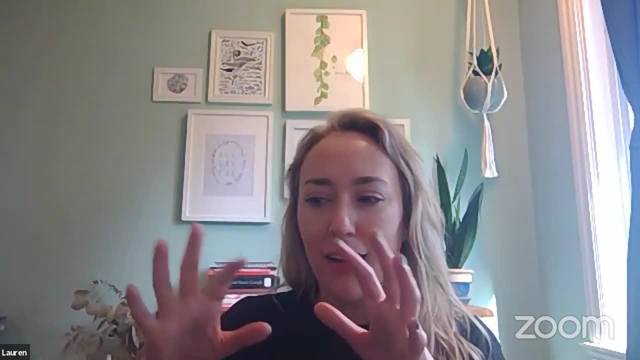 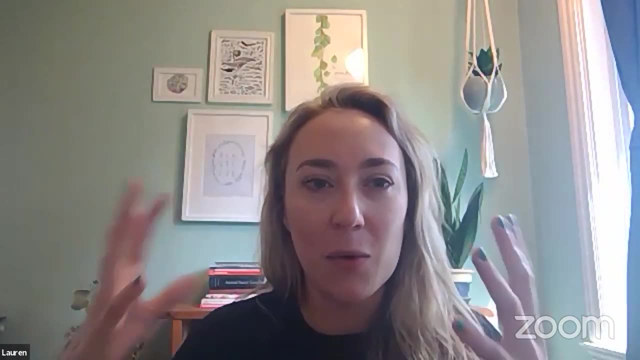 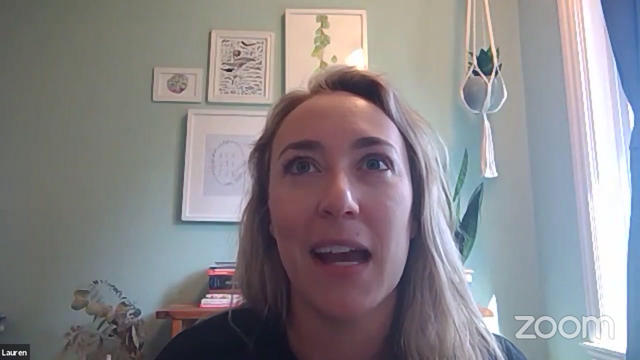 and they're really beautiful and they're really striking to see when you're like coming off a boat from the ocean onto sort of a forested landscape and it's so striking it's almost ghostly to see a sort of a white bear walk out in front of you. and so, um, i was with a. 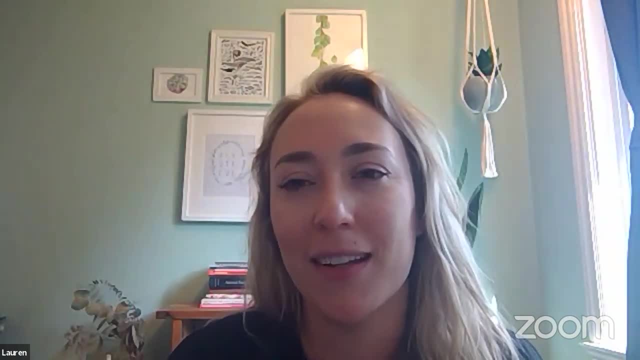 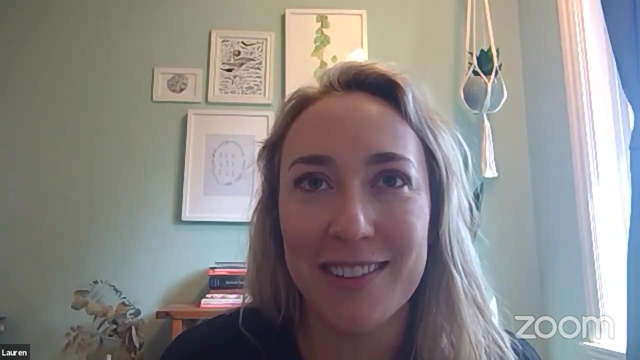 crew up on the coast and we got off a boat to check some trail cams and there was a bunch of black bears and there was one little young white spirit bear fishing. he was trying to fish. he was doing a really bad job. he was still really young, um, but it was incredible. it was really cool that. 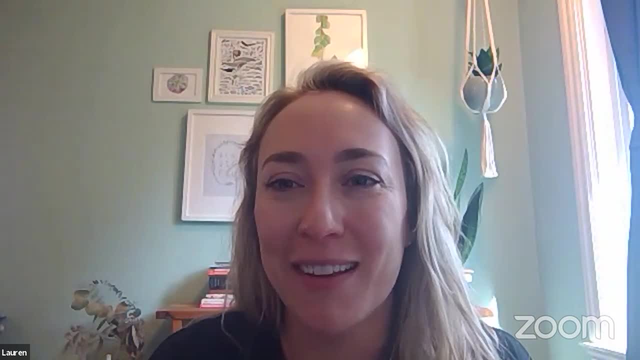 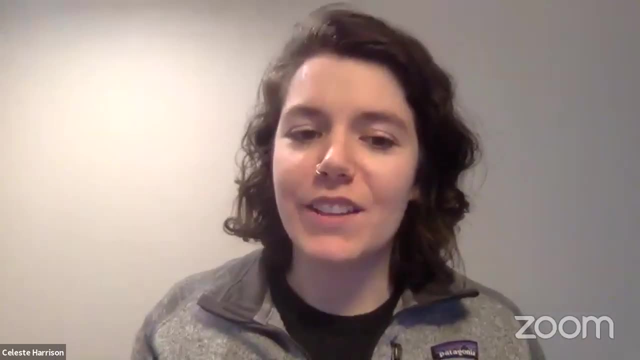 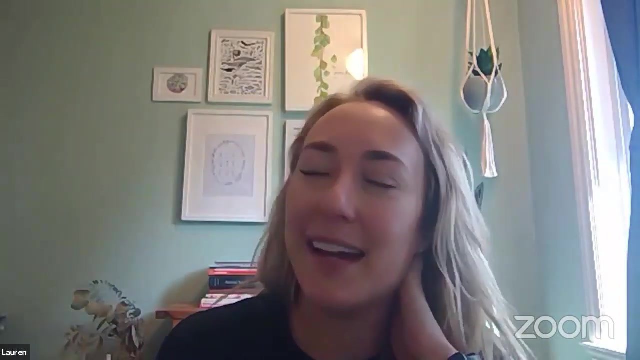 was one of my favorite things i've ever seen. all bear related- uh, it's not on purpose, just bears are really cool. all right, out of all of the different paths in science that you could have taken, what's brought you to your specific discipline now? it's a good question because, admittedly, i i feel like i'm not someone who's really in one. 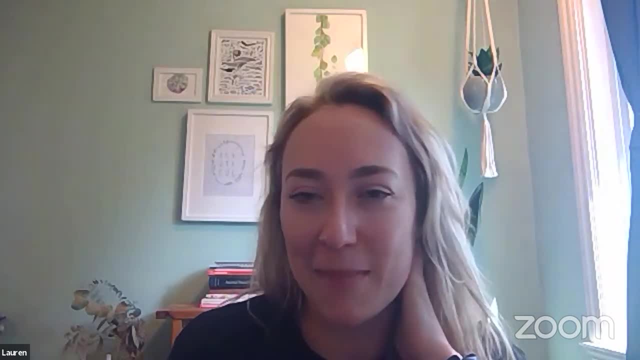 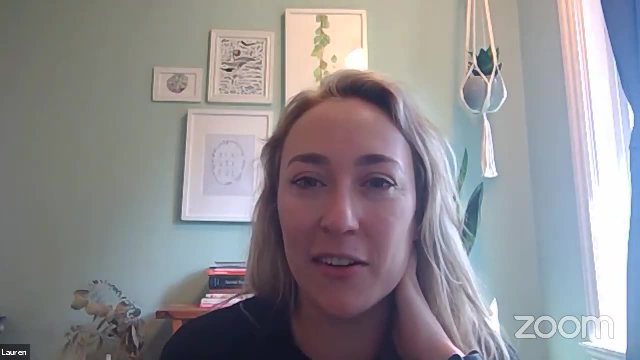 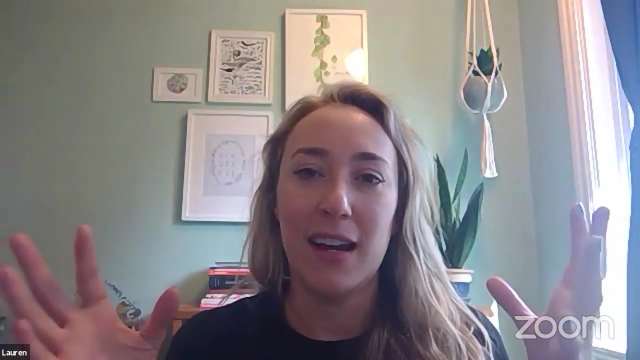 discipline, um, whether that be because i can't make a decision or because i i all- all of us scientists are increasingly recognizing that focusing on just one piece of the puzzle is really important for some of us, but others have to do this tricky thing where we live. 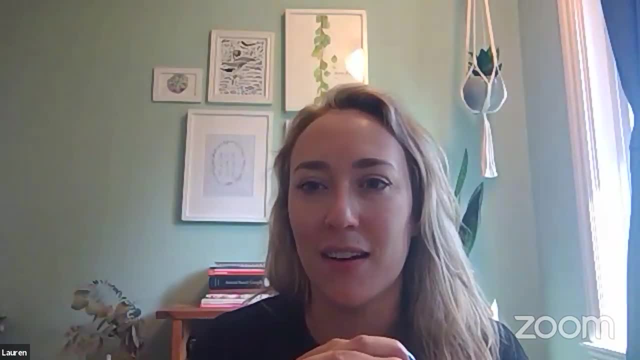 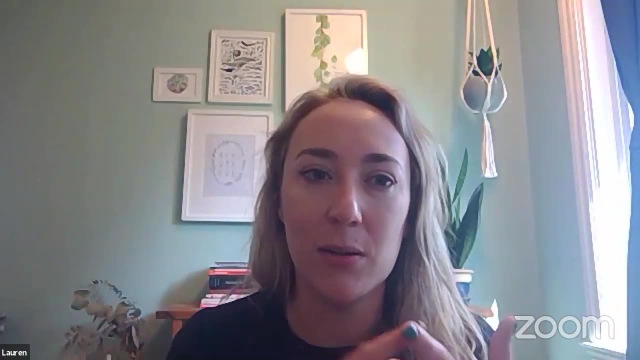 and work in multiple sciences to try and bring them all together to better understand our world. Because, as we see in this moment in life, like we are so interconnected humans, we have to understand social sciences, things like psychology right To understand people, why we do what we do. 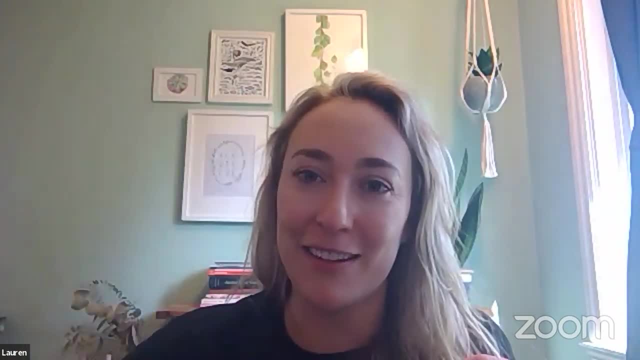 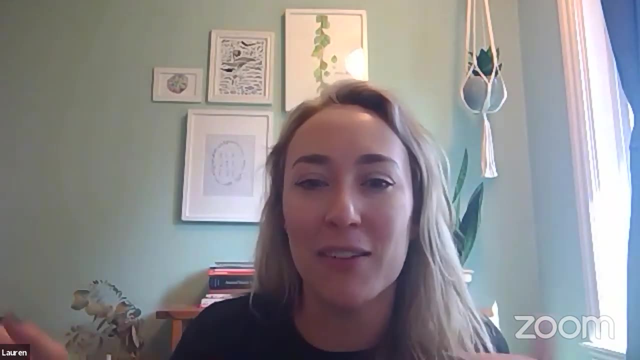 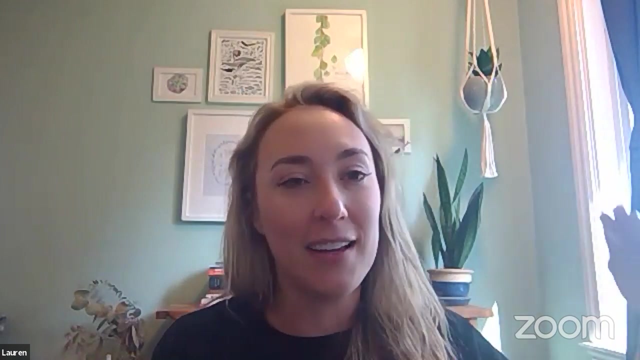 how we think we have to understand bears, like why they do what they do where they are, to understand things like nutrient fluxes, so where calories are in a system and why bears go there. So that's all, just to say I definitely didn't end up in the position I'm in on like a 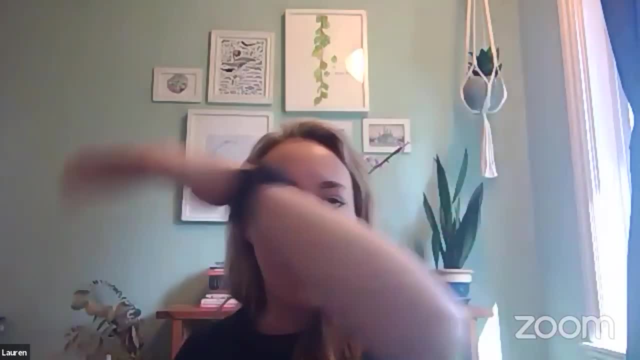 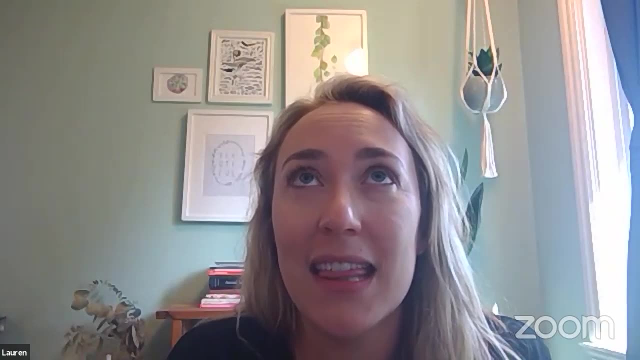 straight and narrow path. I feel like I've sort of jumped around my career so far And I'm lucky, really privileged to be able to have done that- And I think I've sort of gotten to where I am as a social and natural scientist, as a conservation scientist, 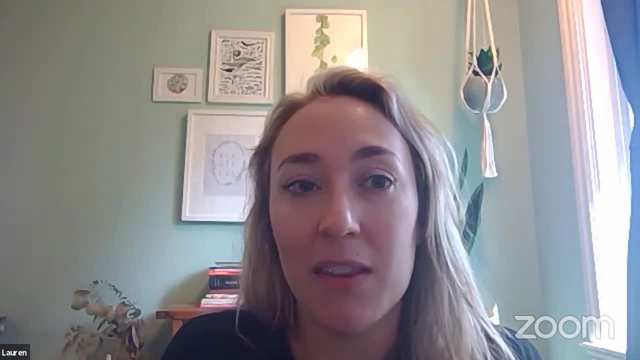 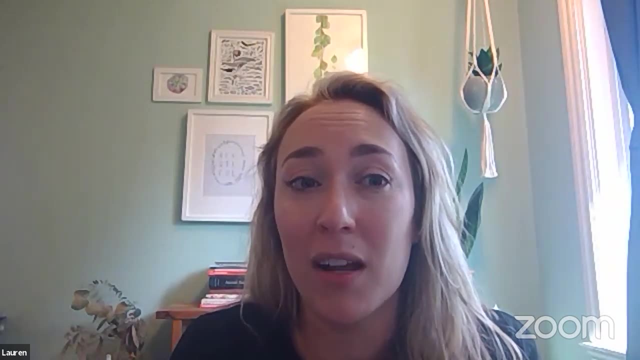 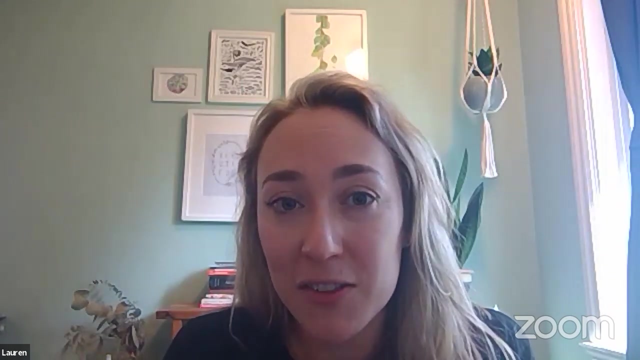 in response to the lessons I've learned working with other scientists in the field and kind of trying, you know, seeing what works and what doesn't, And I learned really early on that what doesn't work in science is excluding the people who live in the places that we do research. 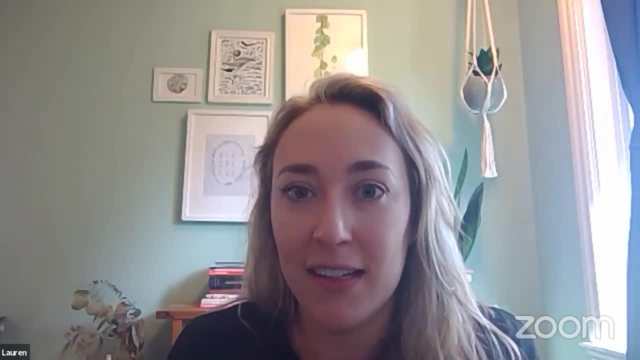 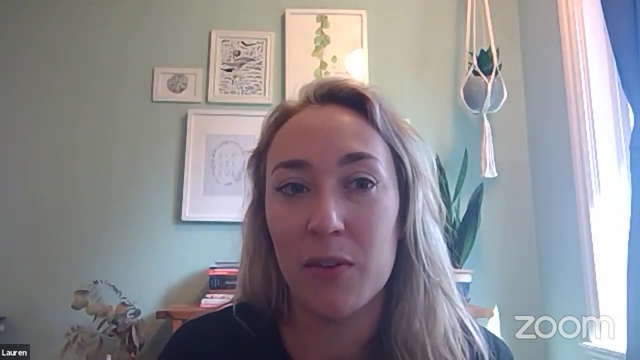 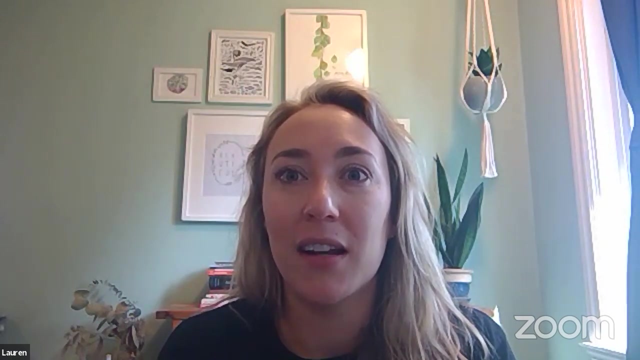 And what doesn't work is doing science that doesn't recognize the value of all sorts of knowledge types, And so I think a lot of us, as scientists, are moving towards science that better includes everyone at the table and also that recognizes that we can't make conservation work. 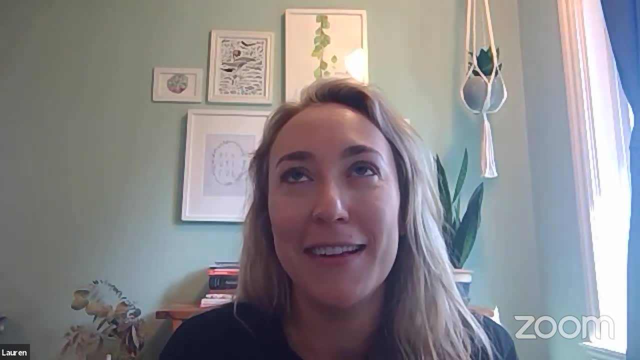 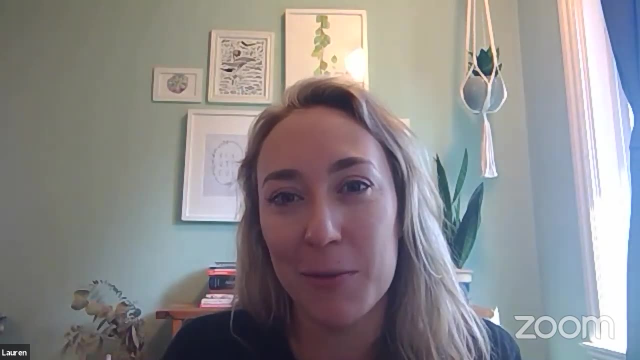 if we don't understand people. So, yeah, this is. it was a very nonlinear, like zigzaggy path to get here And I I'm sure it will continue to be that way And I'm really lucky for that. It's pretty. 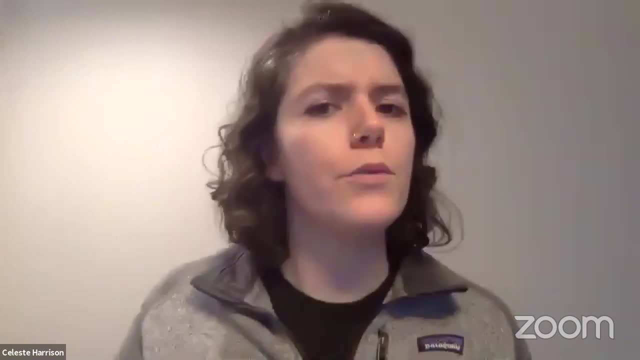 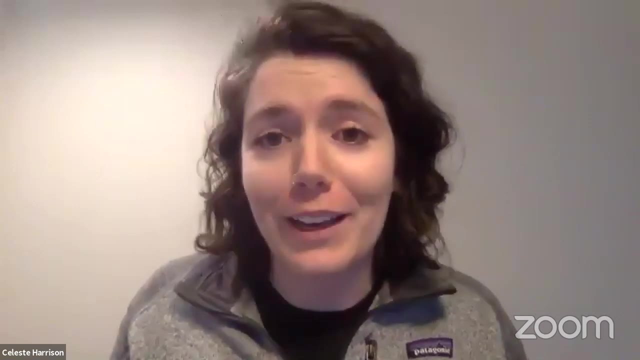 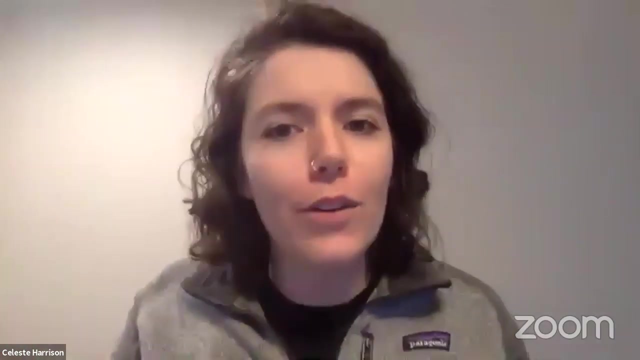 cool, Awesome. We've had a lot of back and forth with different users in the chat bar, You know, trying to decide if it's okay to have bird feeders in your backyard, What exactly to do should they wander into your space. So let's let the expert in Lauren. 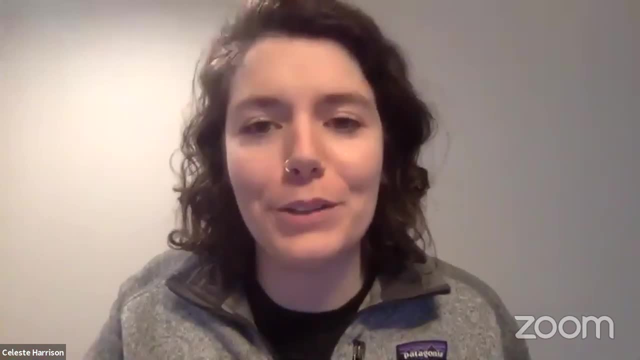 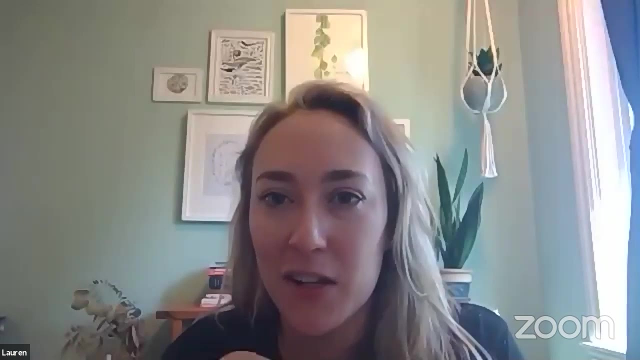 should you put food out in your backyard And what should you do if a bear ends up in your space? So this is a tricky one, And this is why, when I was asked about what you can do specifically sort of in your backyard, I think it's really important that it's context specific. One thing we learn in: 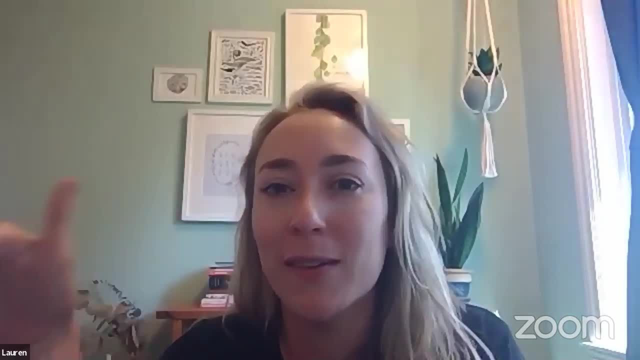 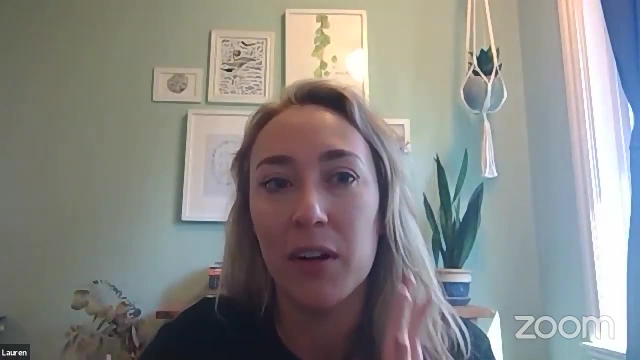 conservation, science and in life in general is no one size fits all solution works for any of us. Um, so If you live in a place like Power River, where I'm hoping to work later this summer or next year, and there's a ton of black bears, you have really high density of black bears. 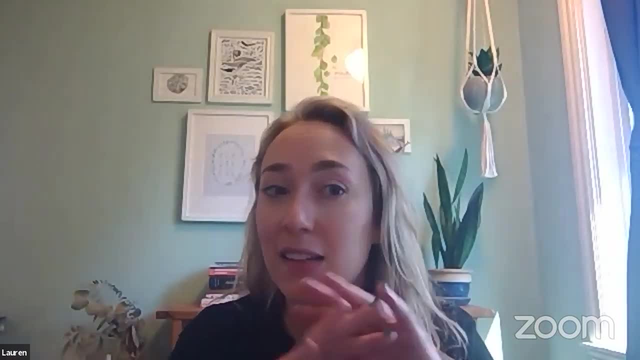 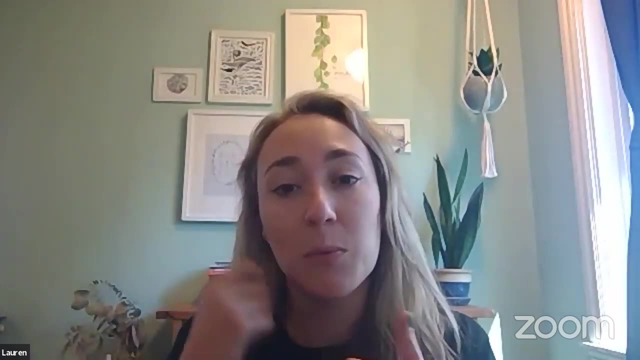 and those black bears are very likely to be in your yard. It is not a good idea to have a bird feeder, And the experts who work in the arena of avoiding conflict will tell you that there. Now, some people still choose to have bird feeders because it's really important to them, And that's. 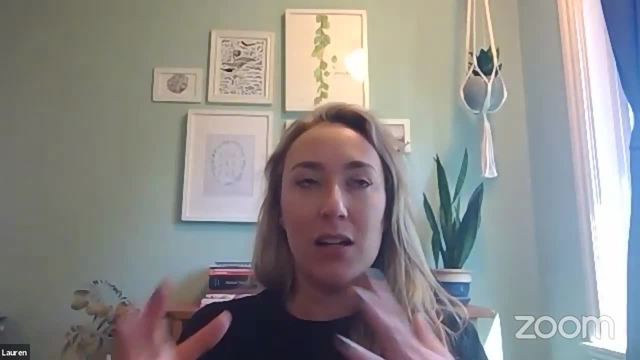 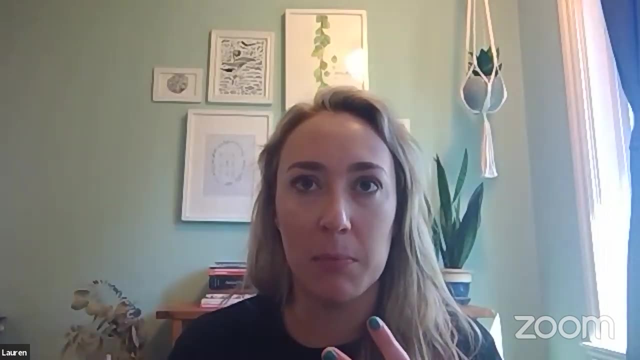 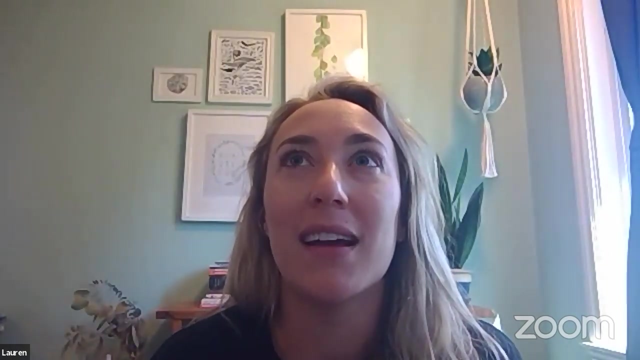 one thing we're trying to understand in the research we're doing is: you know, why do some people value sort of having birds in their yard over avoiding conflict with bears? And how can we work with those people to find creative solutions that say, you know, like how can we make people 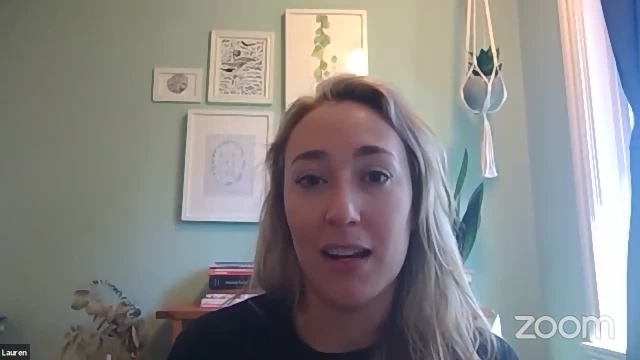 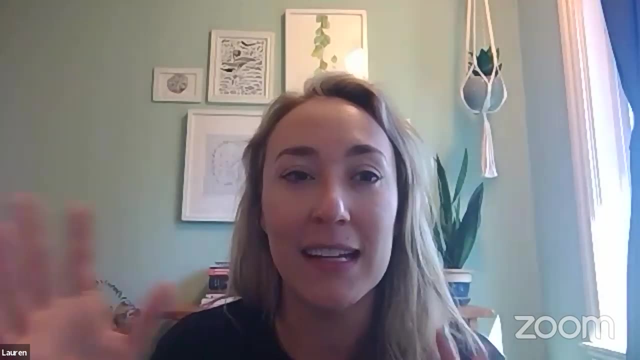 give up the least and still be able to coexist with bears in their backyard. If you live in a place where you're not worried about a bear coming into your backyard being attracted by the smell of sunflower seeds, it's much more okay to have a bird feeder in your backyard. So there's no one. 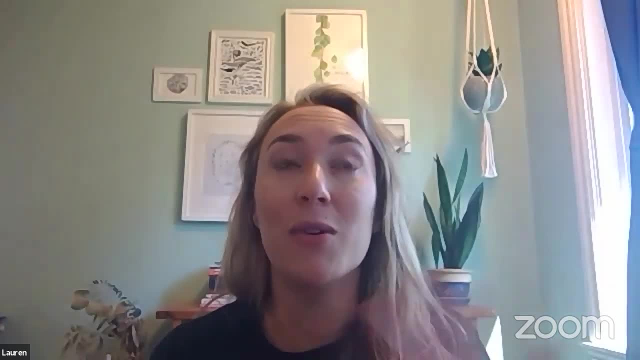 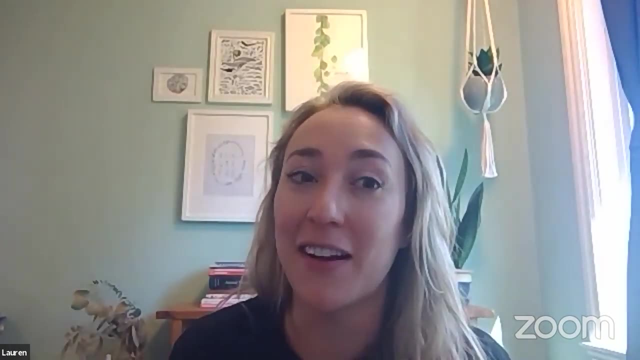 size fits all rule. It depends on where you live, It depends on who you live near, But if you're in high density bear, country bird feeders are not the greatest idea, but not everyone loves that. So that is my two cents on that one. 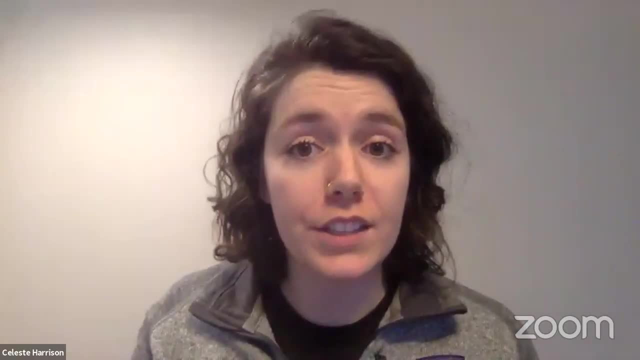 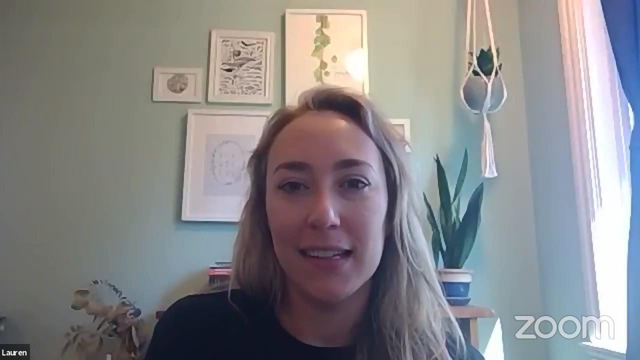 We appreciate that If a bear does make it into your space and you're concerned about that, you wait a little bit. should you call someone? Is there advice for that? So again, I'm still looking forward to learning about that. I'm still looking forward to learning. 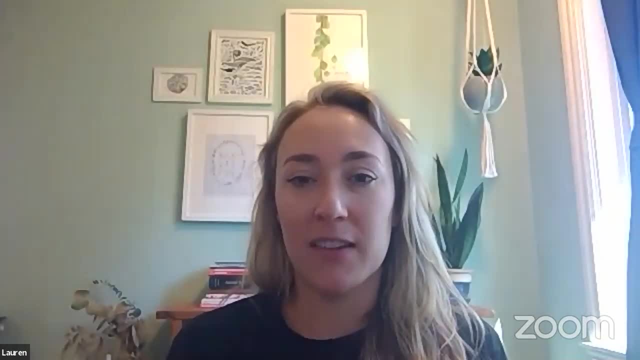 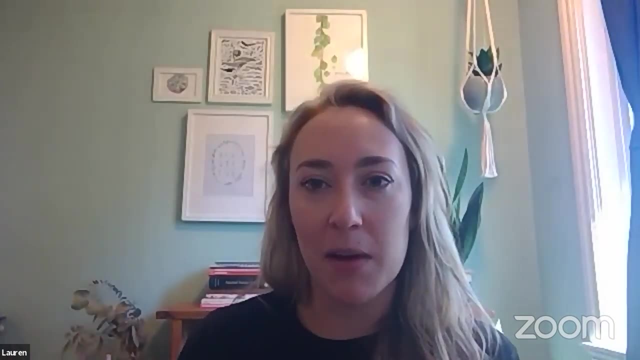 from a lot of people this summer about how they interact with bears in their yard, And so in some ways I feel like I'm not the expert in this stuff, because I have a lot to learn still, But what I do know- experts say- about dealing with wildlife in your yard, especially things like bears or coyotes. 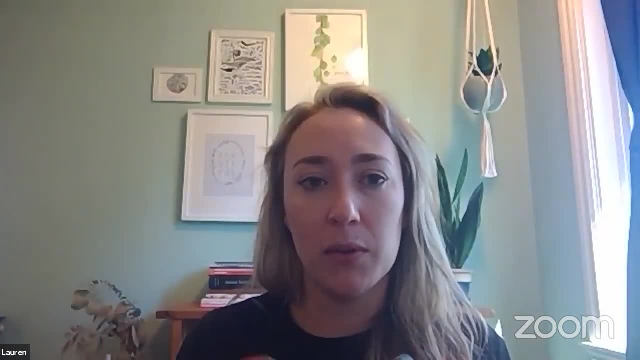 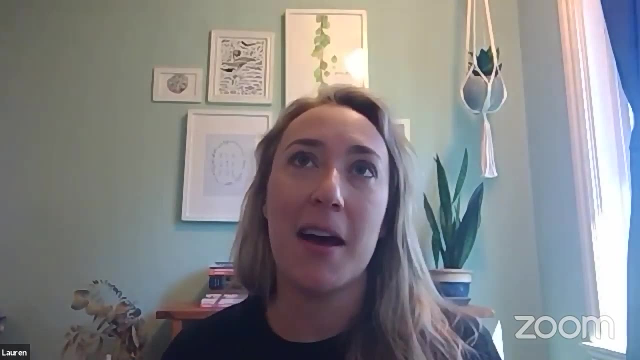 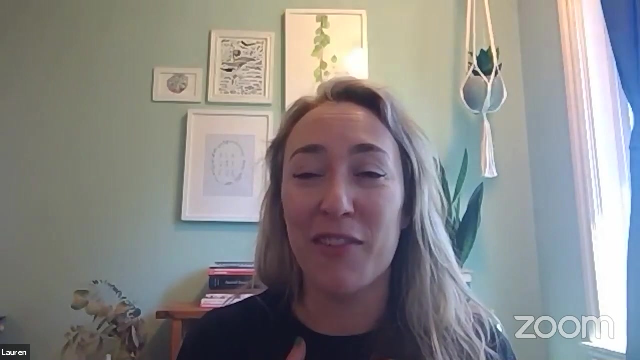 wolves. there's larger animals that can sort of pose a risk- unintentionally but can pose a risk if they're used to. spending time in your yard- is to let the animals know that your yard is not a safe space for them to hang out with, And that's really hard for some of us because it feels good. 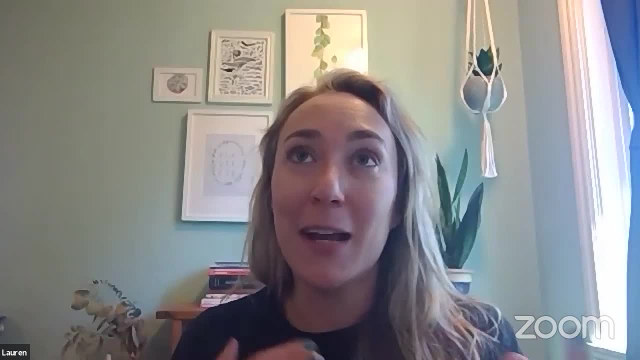 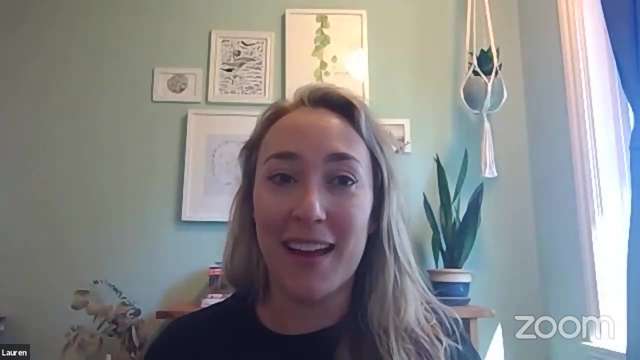 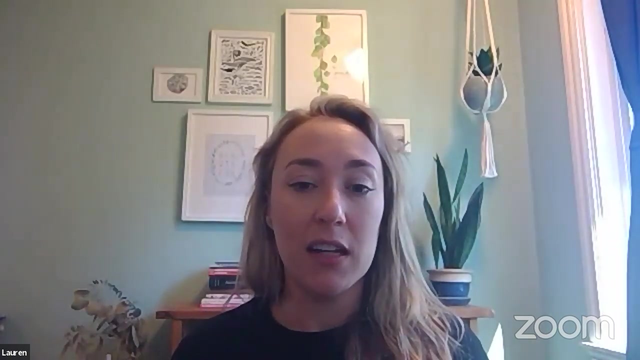 to be close to wildlife if you care about them, But, just like right now, we're all isolating because it's the best thing we can do for each other. The best thing we can do for wildlife is isolate them from us at all times, And so what that means is, if a bear is in your yard, even if they're not, 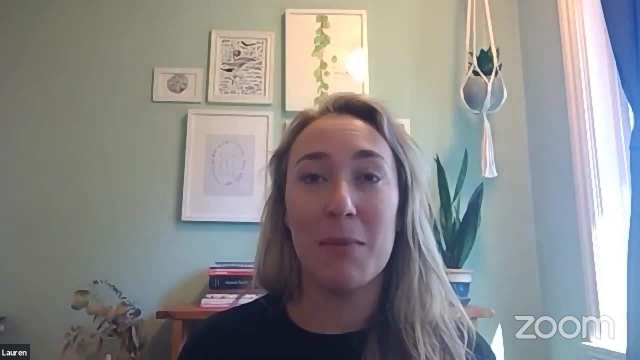 doing anything wrong. the best thing you can do for that bear is to make a really loud noise and say: hey, bear, this is not your space. you've got to get out of here, even if you love bears, And it's really hard. 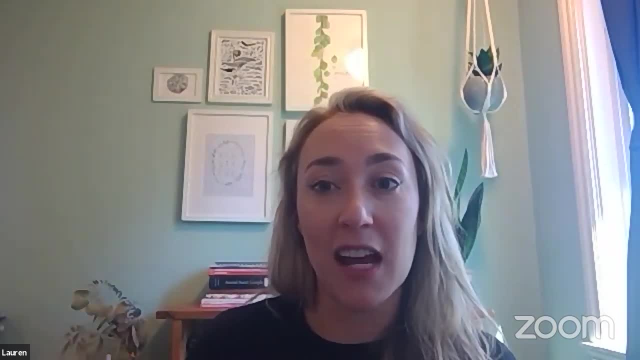 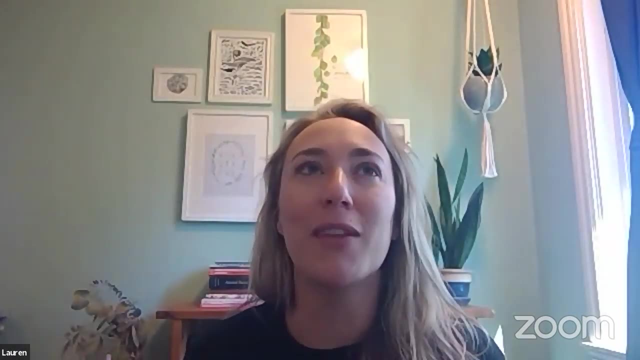 to do, But by doing that you give that bear a better chance to live in the wild, to live away from humans and to survive in the long run. So it's this weird thing where, if you love animals a lot, the best thing you can do is let them know where it's okay and where it's not okay for them. 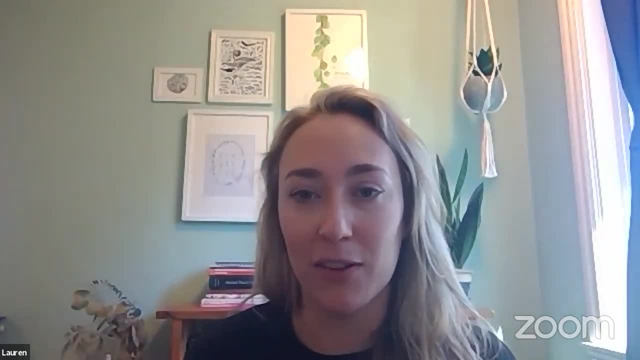 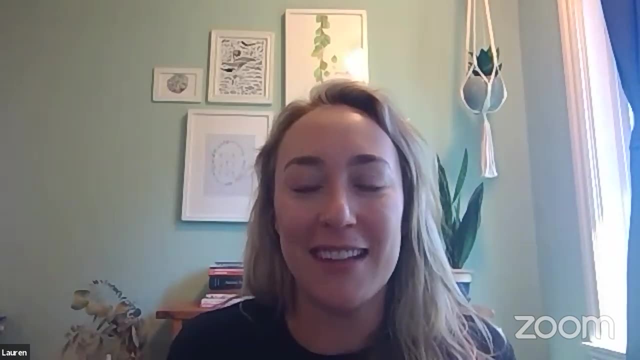 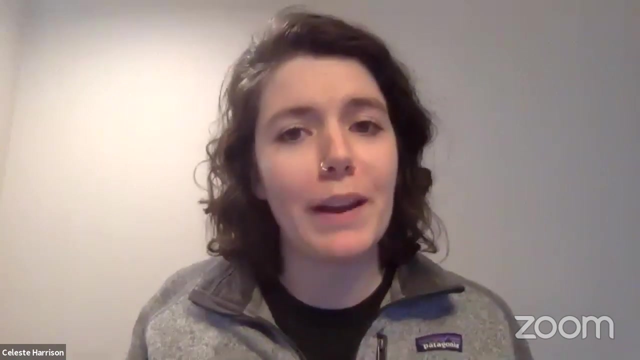 to be And unfortunately our yards are not okay places for them to be, So it feels strange We're saying like I care about you, so stay away. But we can understand that sometimes we have to do things like that. Amazing All right, Lauren, for students who are really inspired by your work today. 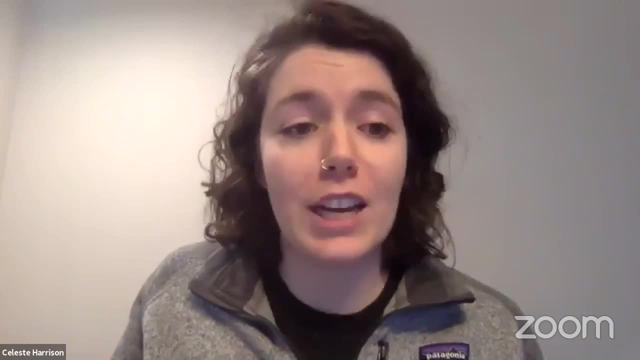 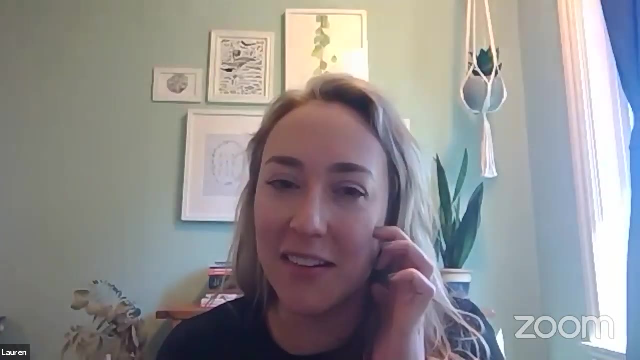 is there anything that they should be doing or that you would recommend to help out their own local wildlife or to get started in conservation? Yeah, I feel like I have a million things to say to that, And it's advice I still give myself every day and many awesome leaders. 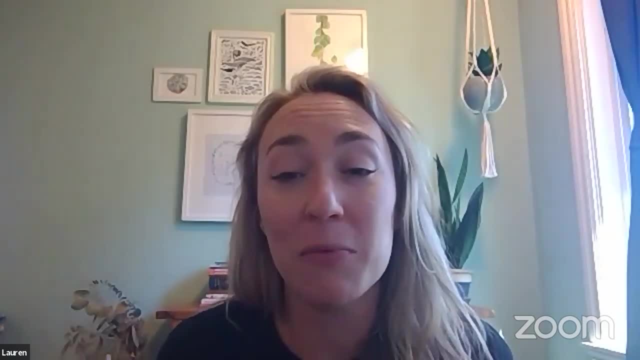 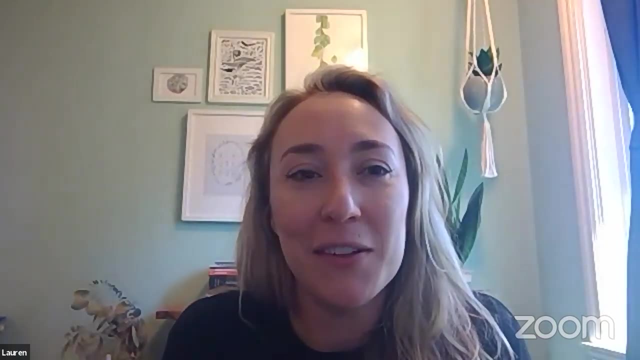 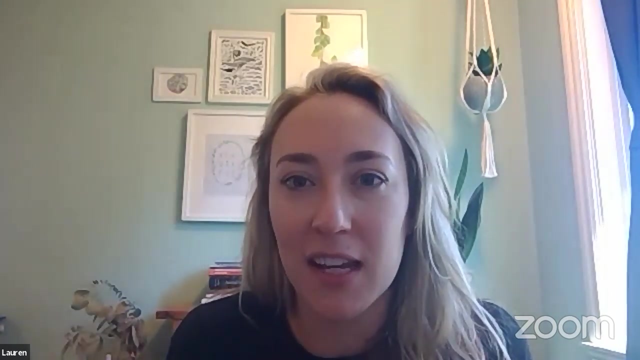 have given me throughout my life, And what I can just say is get really curious. we live in a super incredible world that i think we just get used to, so we forget how magical it is. our own backyards have so many magical things going on in them. if we can just take a second. 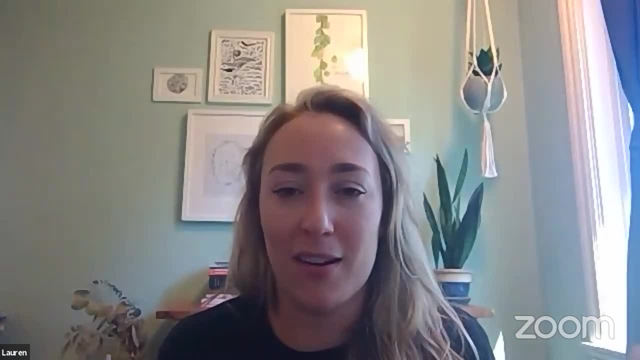 to look right, and if we don't have a backyard, the potted plant on our windowsill has really amazing things going on in it, and we're so lucky to have access to the world wide web of information. so my advice for everyone is to start by really looking around you like really getting curious. 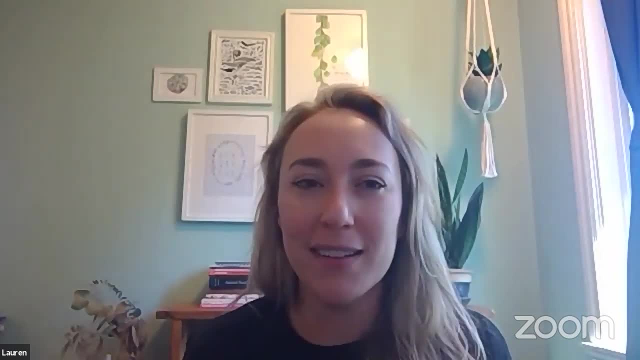 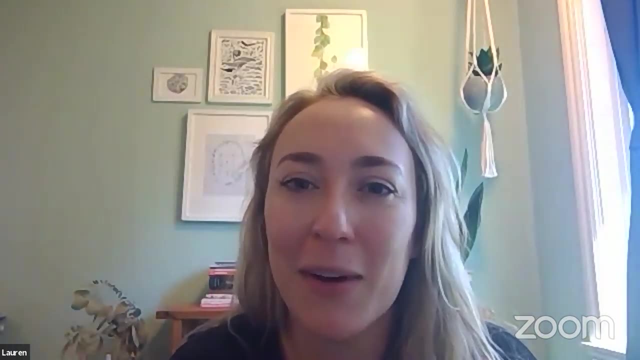 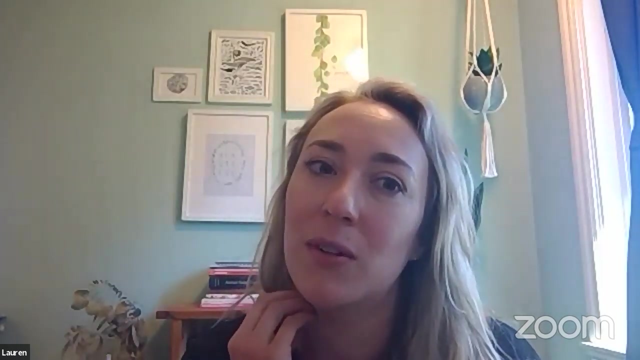 and chasing the things that you love. like if you read something or you have a question that you really care about, just it's yours. like, just pursue that question, just chase that thing you love, it's so worth it. um, and, and keep in mind that all of us do have a responsibility to each. 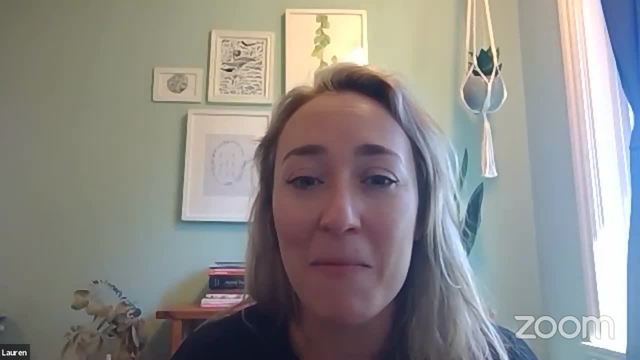 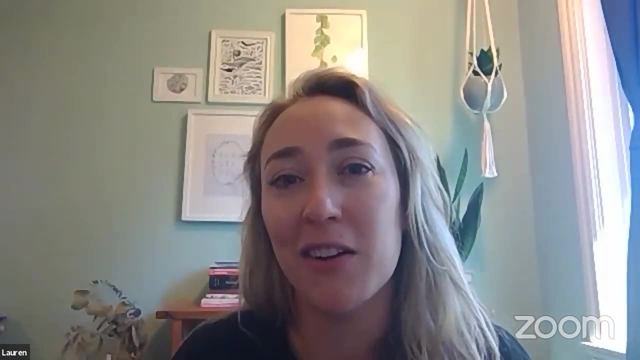 other and to wildlife to be kind. um, and there are a lot of creative creativity and a lot of creative creativity in the company that we work with and a lot of creativity in the company that we work with is these communities that are like ways to do that and those ways can with you guys, like you can start now. um, just being curious and 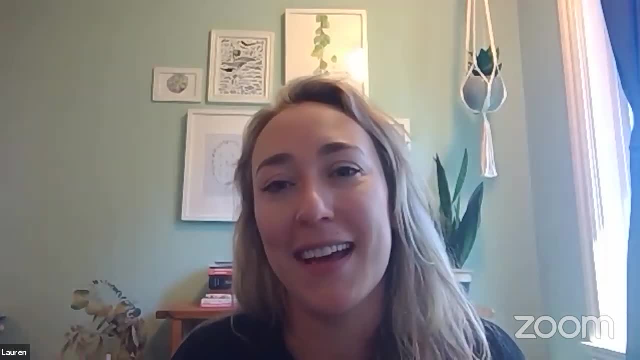 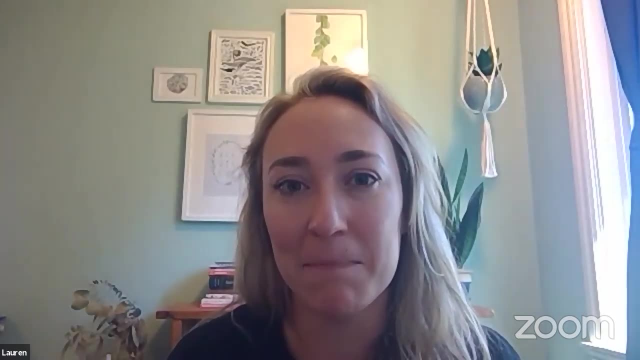 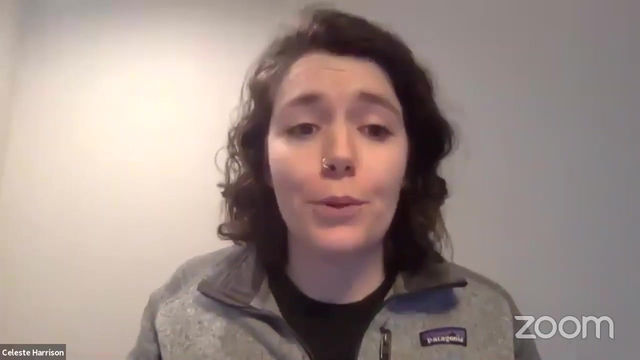 learning more and asking questions, reading books, um yeah, and- and wondering about all the amazing things that are happening all around us all the time. i love that. what great advice. all right, everyone be sure to check out. explore classroom: we've got many, many sessions coming up. we also. 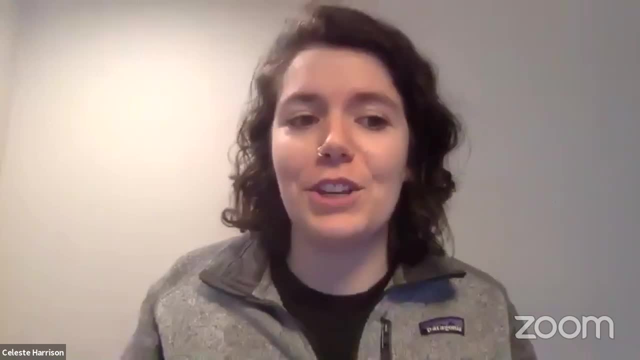 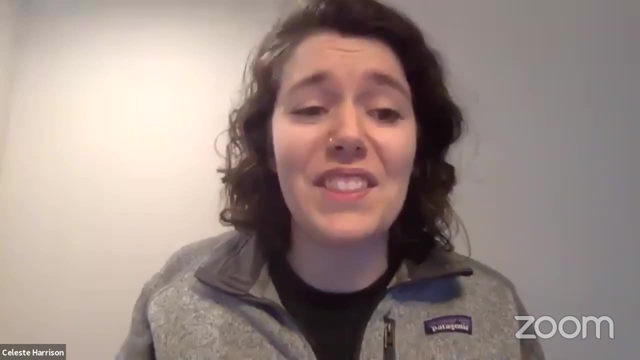 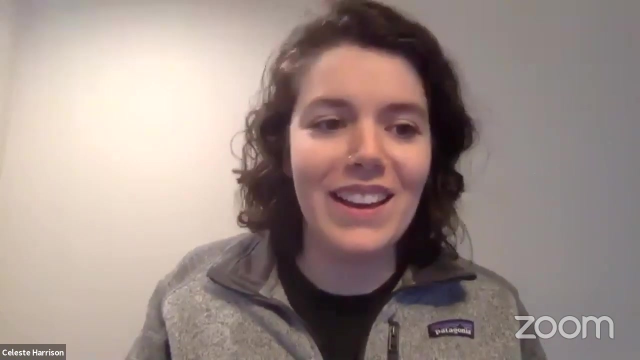 have many, many other educational resources on natgeoedorg. we hope to see you at some upcoming events and on some of our resource library pages. everyone out there can tune in at this same time tomorrow for a session about engineering critter cams with biologist kyler abernathy, and i think 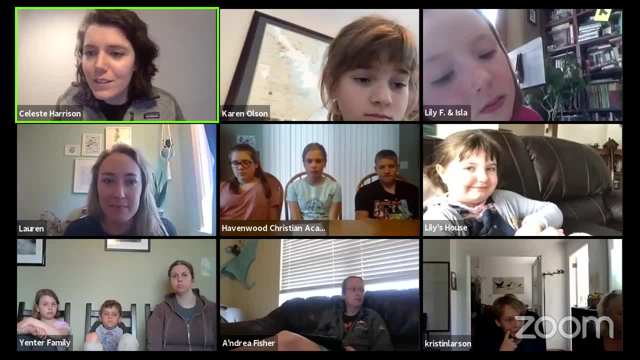 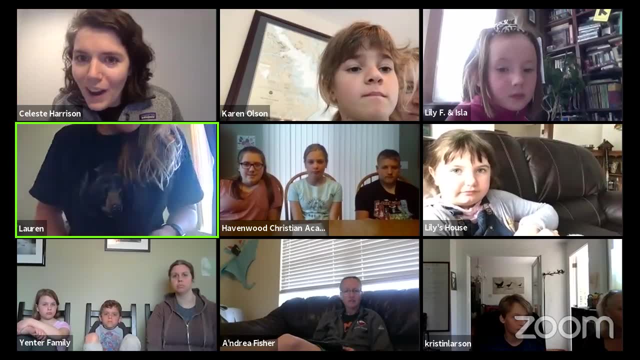 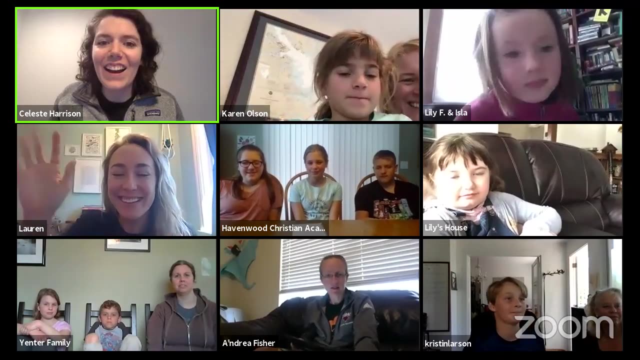 now it's time for me to turn on all of the different microphones so that our students have a chance to say goodbye and thank you. i'm gonna show off my shirt really quickly. i'm wearing a black shirt for all of you guys today. oh my gosh, i love it. all right, all the microphones are on nice, and. loud. everyone, let's say bye and thank you. 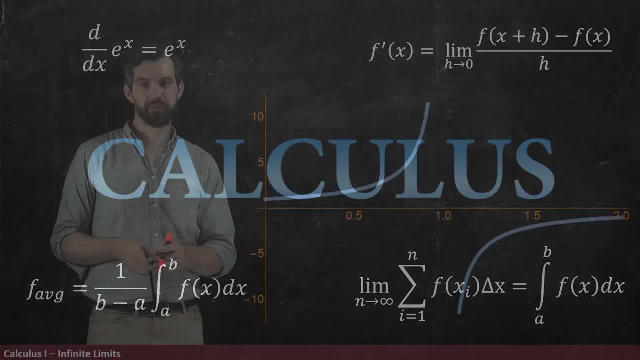 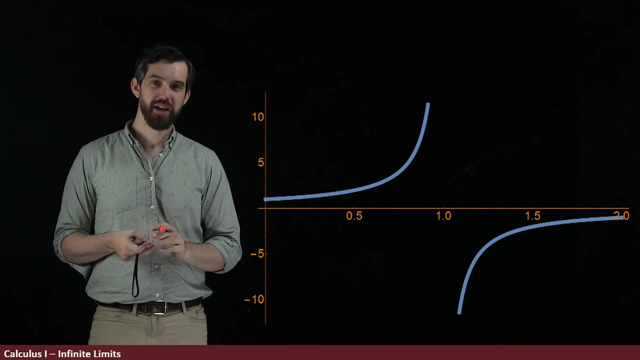 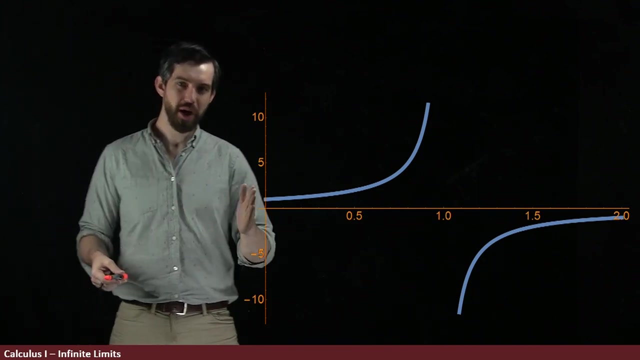 Here is a slightly different graph, and I want to try to figure out what limits might mean in this case. This is a very interesting problem at x equal to 1. Notice that if I'm coming from the left here, so I'm going along, I'm going along. 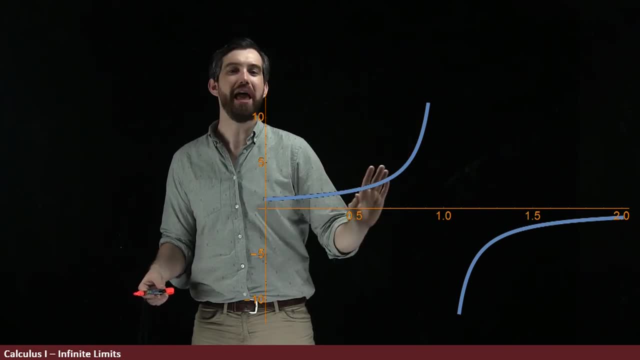 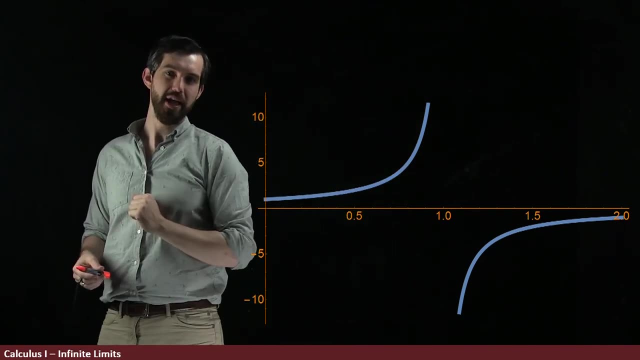 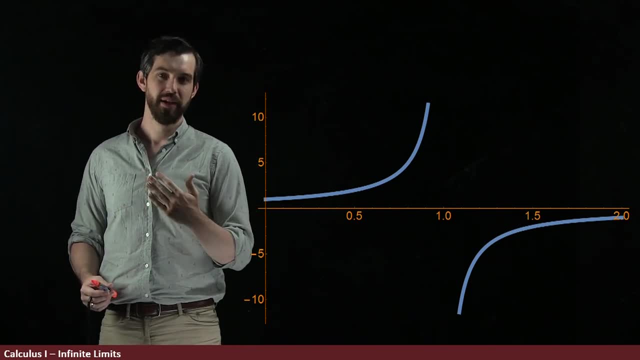 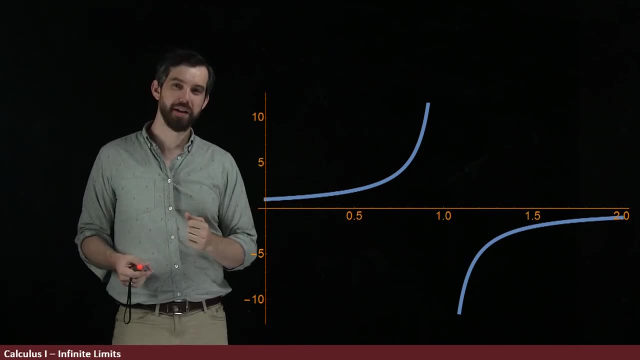 and sort of going down towards minus infinity. And then at the actual point of x equal to 1, this function isn't even defined. It's not like f of 1 is some number. So I want to be able to talk about the limits for this particular graph. 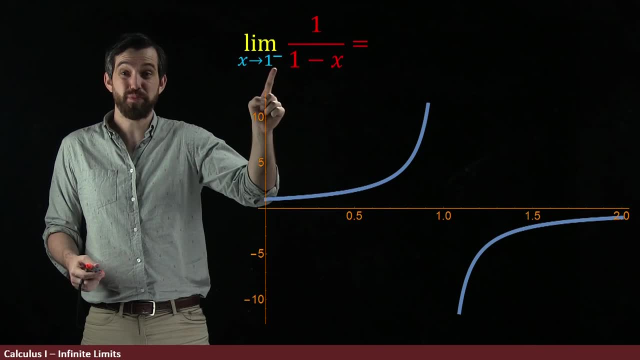 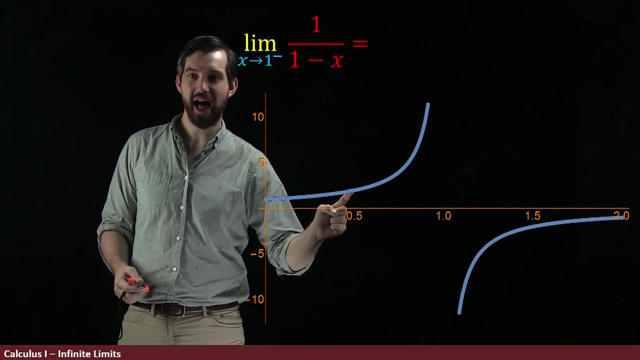 So the first one is I want to look at the limit. one is the clear spot. that's interesting. all the other ones, for example, if I want to know what the limit was as it got close to 0.5, I'd be like that's 0.5,, it's just whatever that height is. 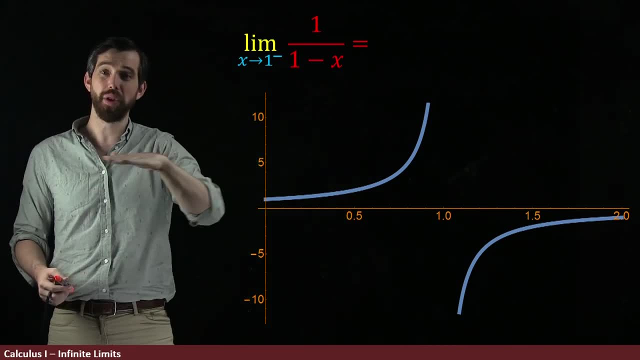 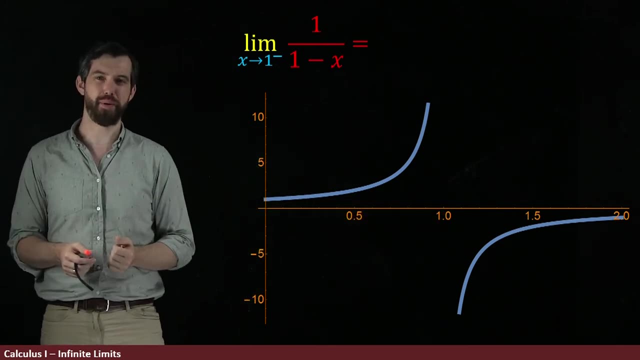 The limit's not that interesting when you've got this nice so-called continuous graph, But the spot that's interesting is this: x equal to 1.. That's where I got some interesting behavior, where I figure out what do I want to do? 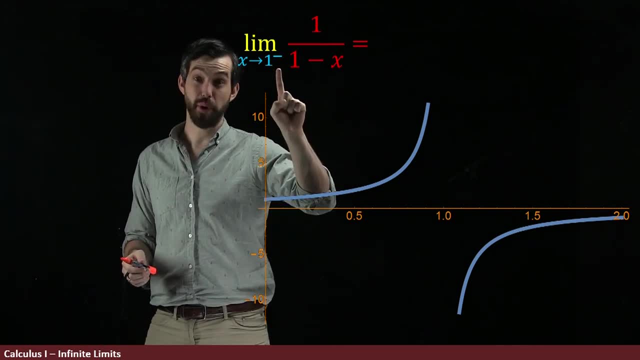 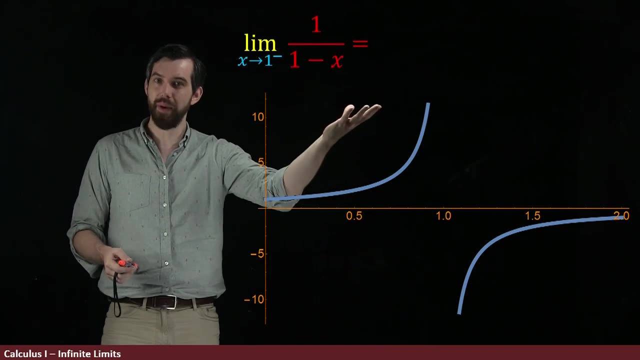 So first of all I'm going to do the limit from the left, where I put my exponent minus 1. here, The function that I've graphed is the function 1 over 1 minus x and you can see that there's a problem at x equal to 1, a division by 0..